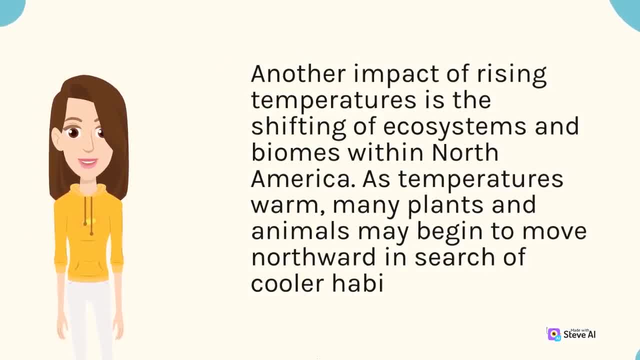 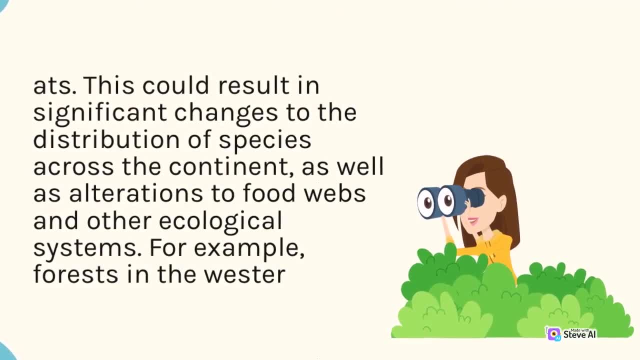 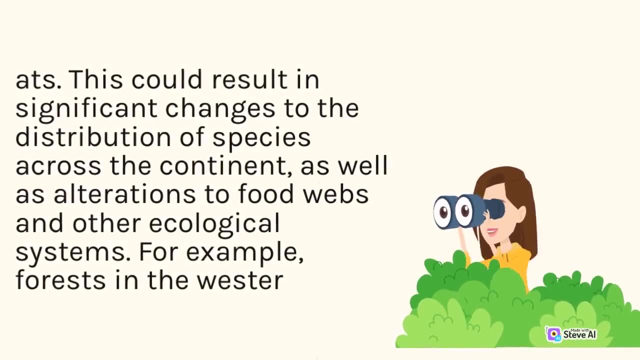 flooding, especially during the sitem attributeary season, For example in the mid 20-ärke seasons. more estan changer. albumia and magn任us type satellites will become rare to grow. The most significant effect of these climate changes is thatrising temperatures will continue. 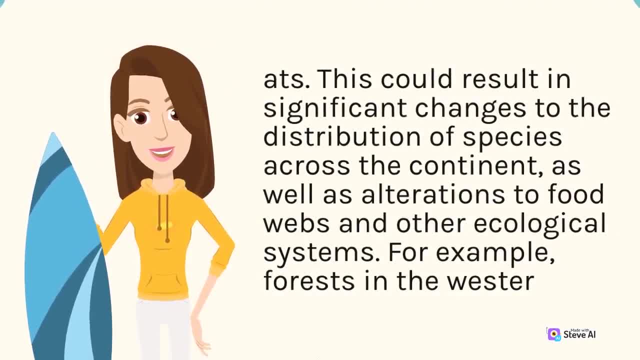 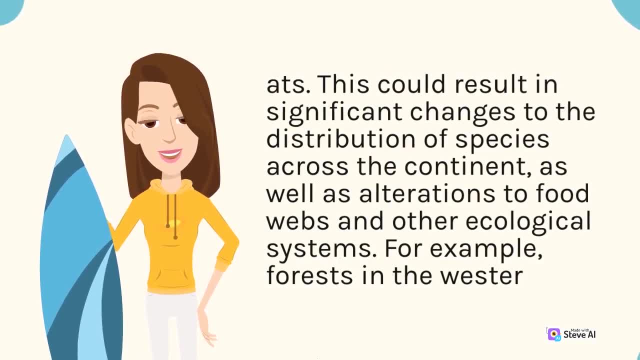 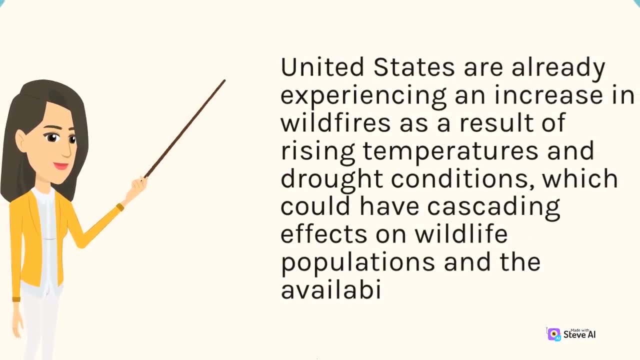 in the coming years. Autographs show what happened on August 23 in Happy Island, about a month after climate change wasینiziwa, For example. forests in the western United States are already experiencing an increase in wildfires as a result of rising temperatures and drought conditions, which could have cascading effects on wildlife populations and the available. 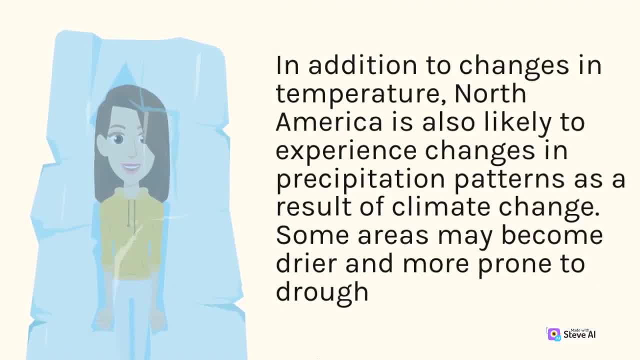 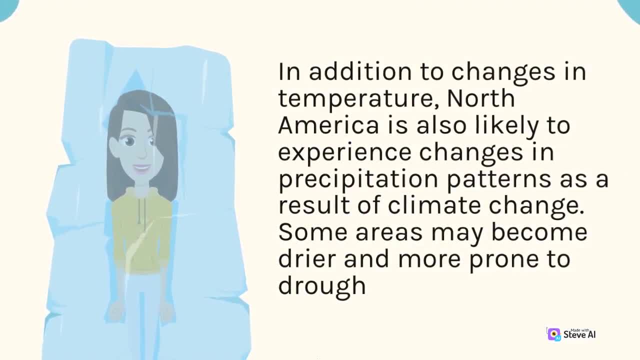 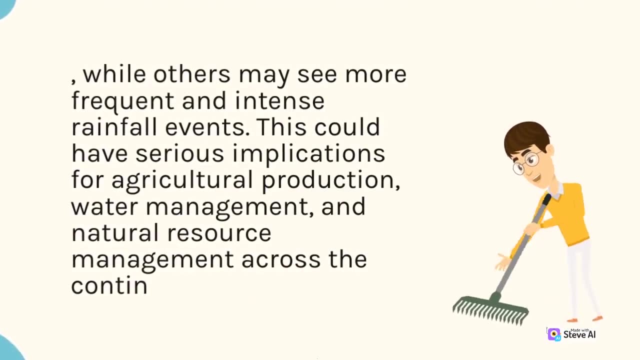 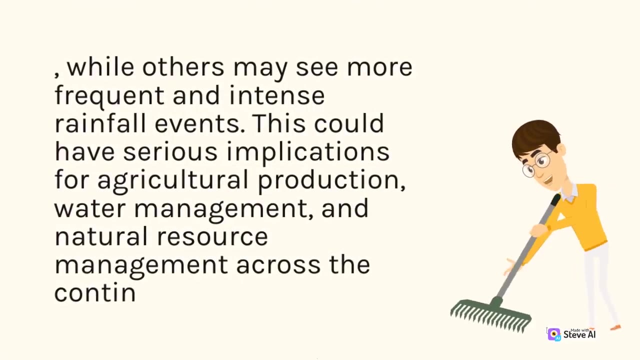 In addition to changes in temperature, North America is also likely to experience changes in precipitation patterns as a result of climate change. Some areas may become drier and more prone to drought, While others may see more frequent and intense rainfall events. This could have serious implications for agricultural production, water management and natural resource management across the continent. 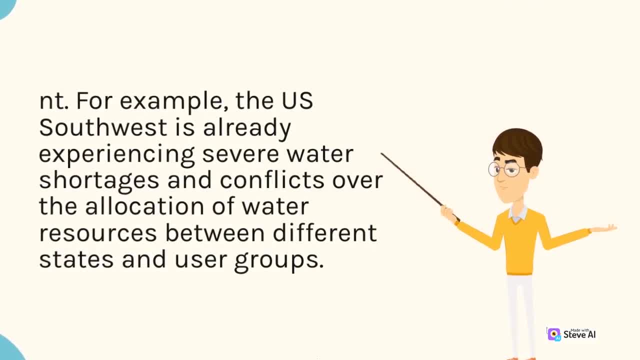 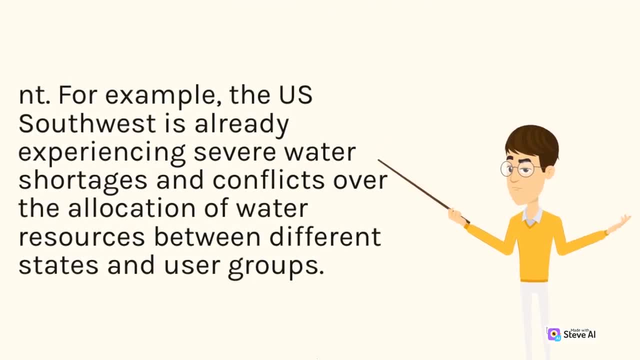 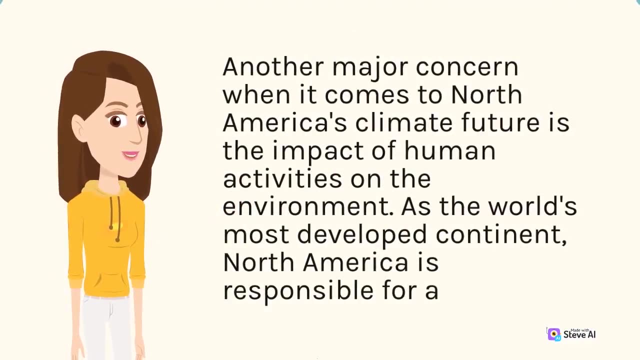 NT. For example, the US Southwest is already experiencing severe water shortages and conflicts over the allocation of water resources between different states and user groups. Another major concern when it comes to North America's climate future is the impact of human activities on the environment. As the world's most developed continent, North America is responsible for a 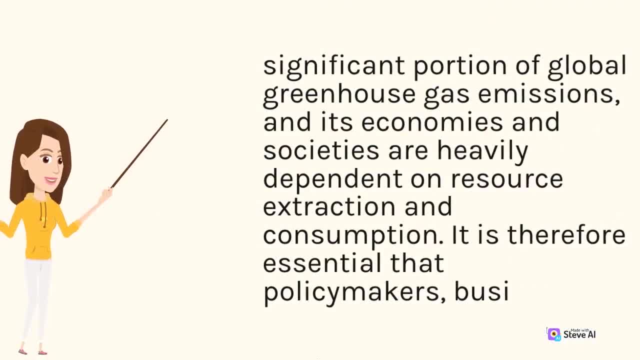 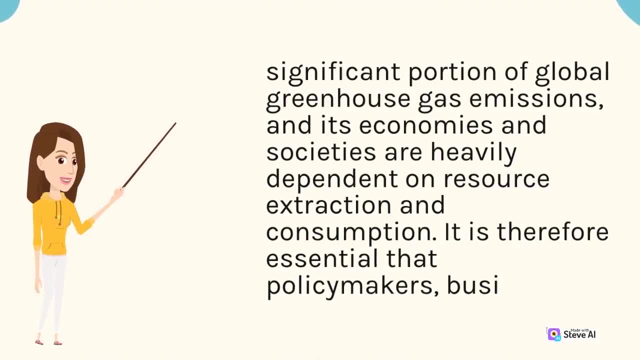 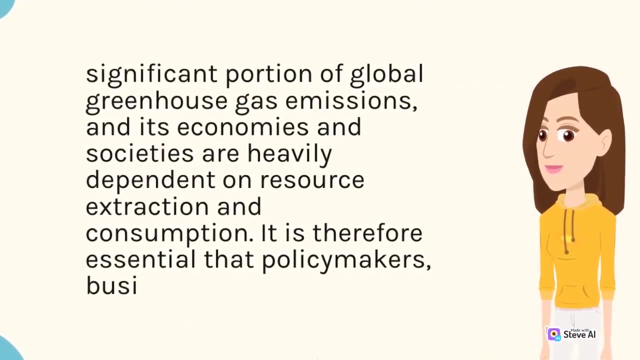 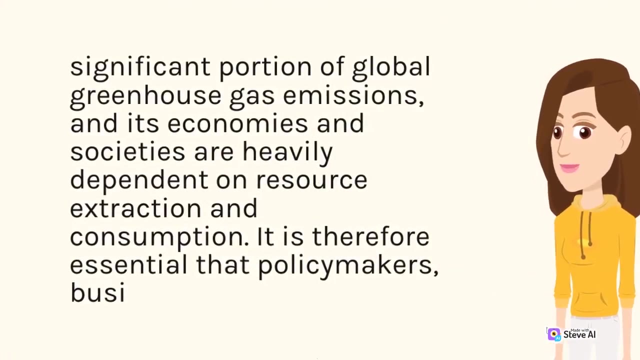 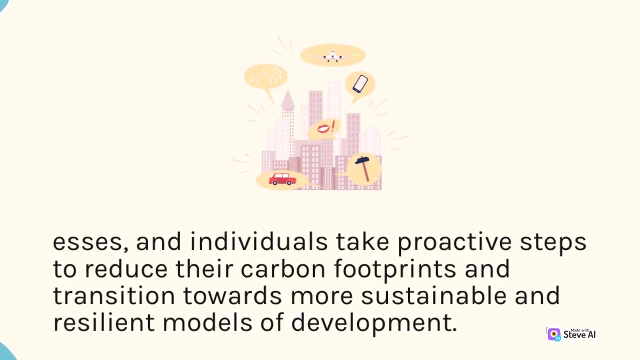 significant portion of global greenhouse gas emissions, and its economies and societies are heavily dependent on resources Extraction and consumption. It is therefore essential that policymakers Boosie significant portion of global greenhouse gas emissions, and its economies and societies are heavily dependent on resource extraction and consumption. It is therefore essential that policymakers, Boosie S's and individuals take proactive steps to reduce their carbon footprints and transition towards more sustainable and resilient models of development. 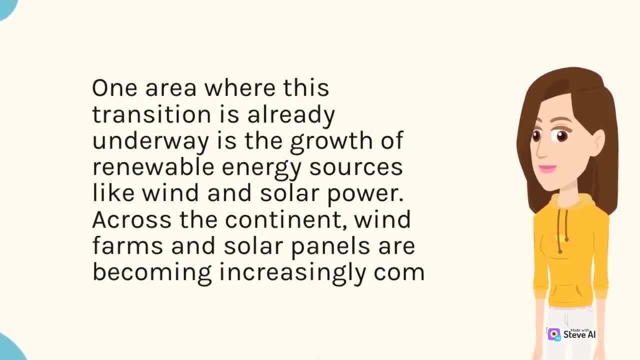 Right MARCUS. ONE AREA WHERE THIS TRANSITION IS ALREADY UNDERWAY IS THE GROWTH OF RENEWABLE ENERGY SOURCES, LIKE MARCUS. ONE AREA WHERE THIS TRANSITION IS ALREADY UNDERWAY IS THE GROWTH OF RENEWABLE ENERGY SOURCES, like 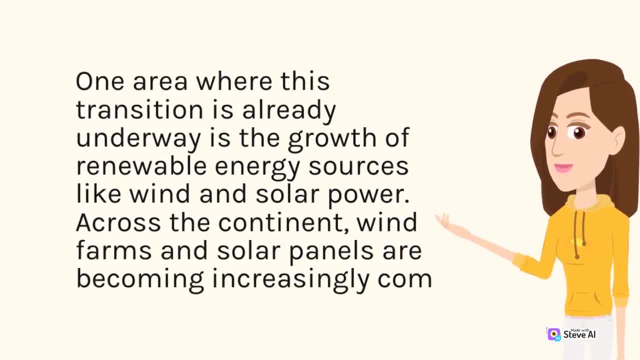 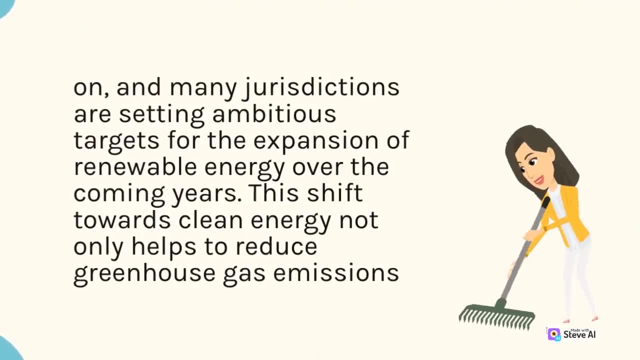 wind and solar power. Across the continent, wind farms and solar panels are becoming increasingly calm. MINE 축 자, ONN AND MANY JURISDICTIONS, ANTOGON AND MANY JUSB HDR are setting ambitious targets for the mildage to around the. 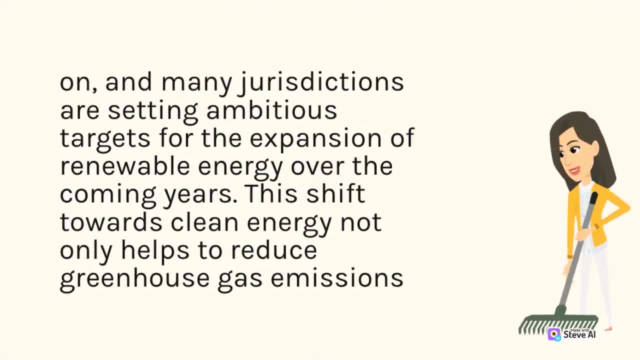 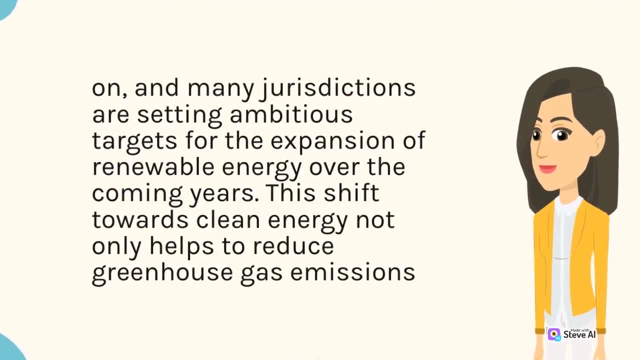 AUGUS AND MOOO TORTRES: energy over the coming years. This shift towards clean energy not only helps to reduce greenhouse gas emissions. MINE citing ONN AND MANY JURISDICTIONS, ARLETO setting ambitious targets for the expansion of renewable energy over the coming years. 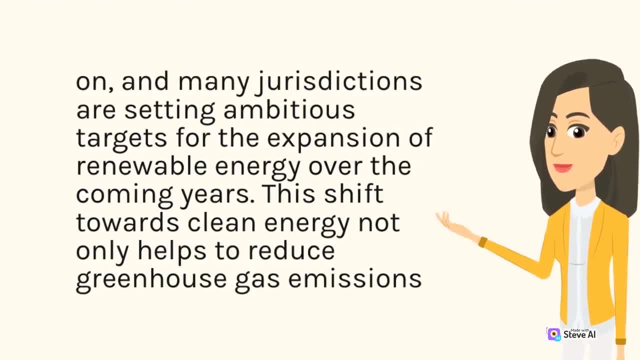 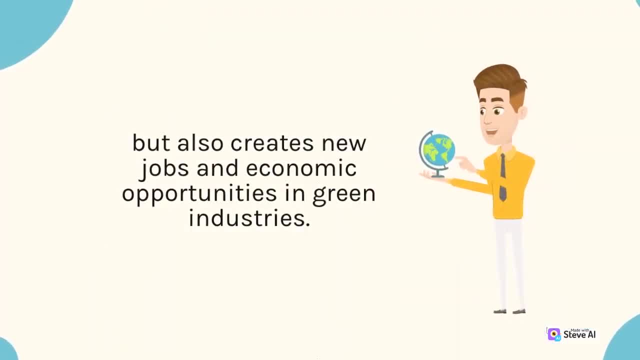 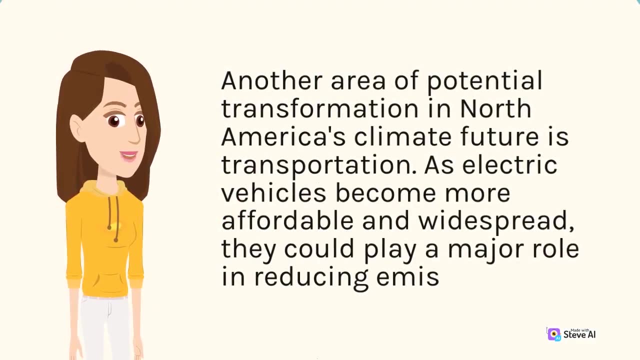 This shift towards clean energy not only helps to reduce greenhouse gas emissions, but also creates new jobs and economic opportunities in green industries. Another area of potential transformation in North America's climate future is transportation. As electric vehicles become more affordable and widespread, they could play a major role. 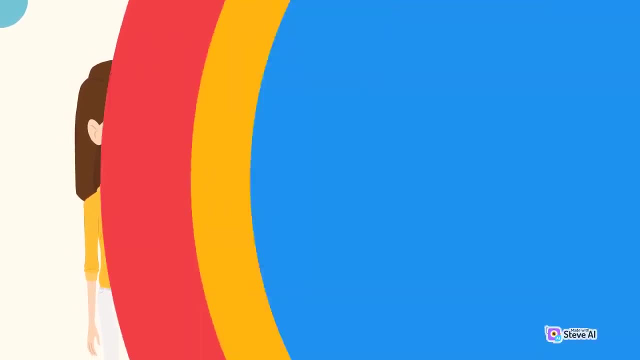 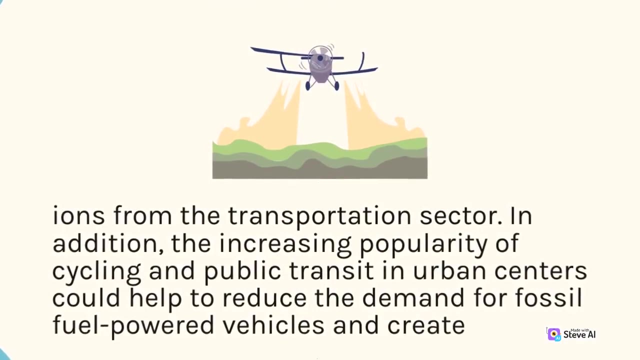 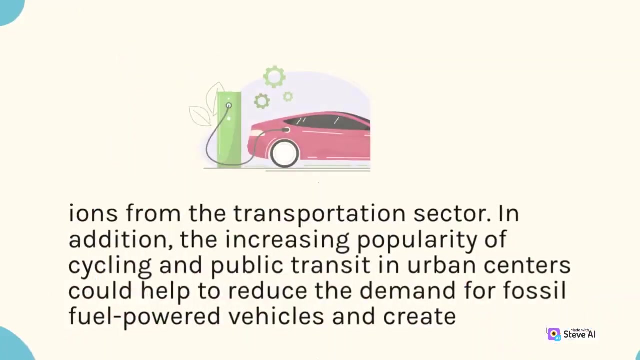 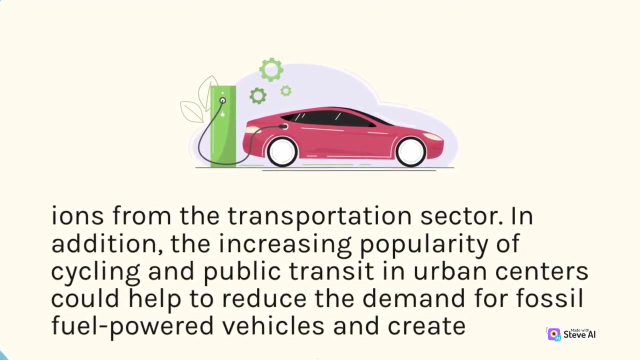 in reducing emiss Ions from the transportation sector. In addition, the increasing popularity of cycling in public transit and urban centers could help to reduce the demand for fossil fuel powered vehicles and create Ions from the transportation sector. In addition, the increasing popularity of cycling in public transit and urban centers could help to reduce the demand. 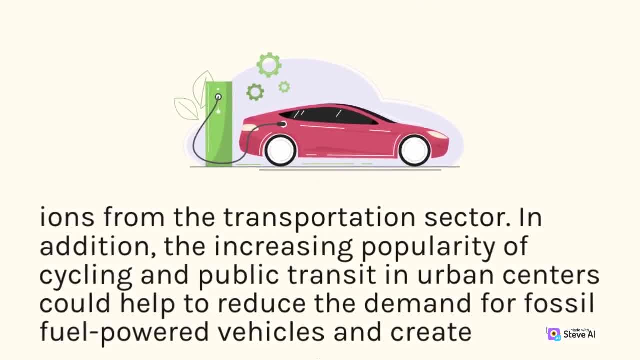 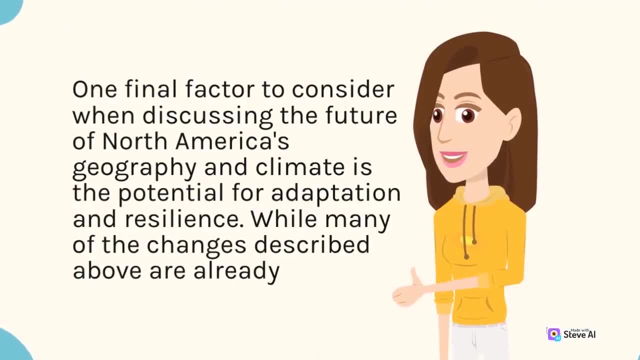 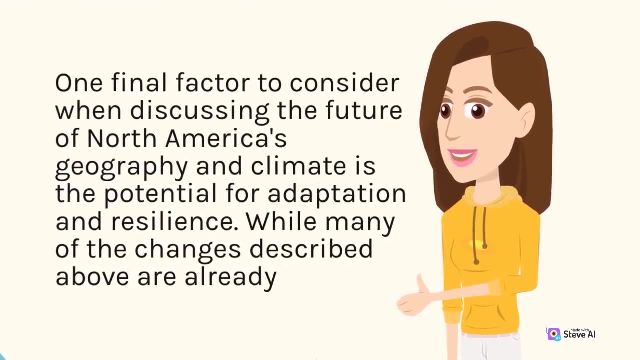 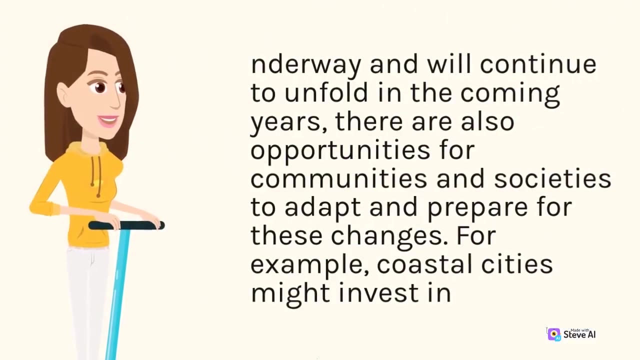 for fossil fuel powered vehicles and create Or sustainable and equitable transport systems. One final factor to consider when discussing the future of North America's geography and climate is the potential for adaptation and resilience. While many of the changes described above are already Underway and will continue to unfold in the coming years, there are also opportunities. 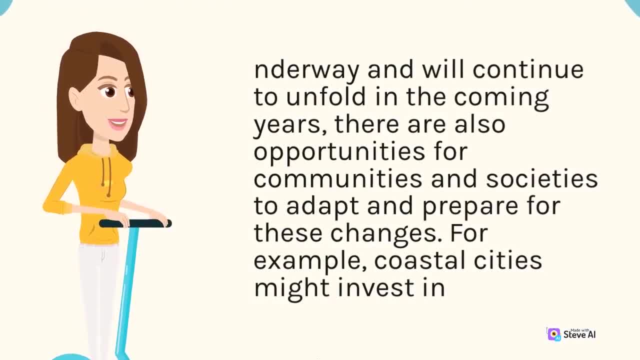 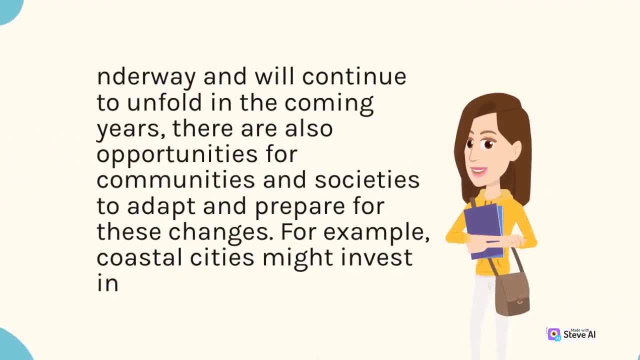 for communities and societies to adapt and prepare for these changes. For example, coastal cities might invest in Seawalls and other protective infrastructure to mitigate the risks of sea level rise and storm surges. Farmers might adopt new crops and water management practices to cope with changing climate. 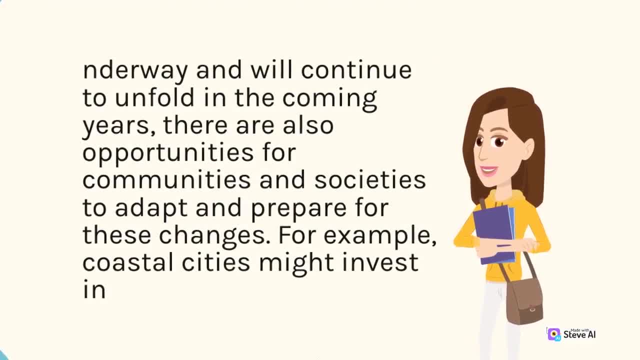 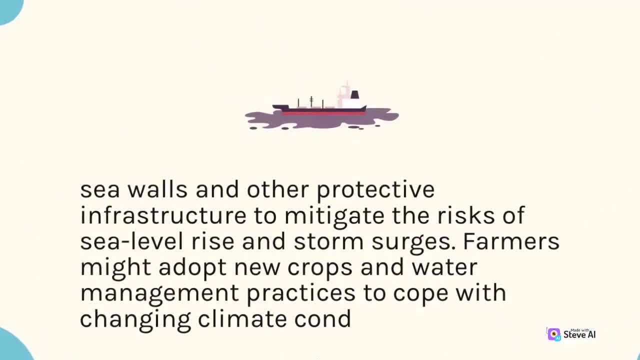 cond. Ultimately, the future of Asia could olurs to. you're waiting for that graph behind the greenangled city where I'm looking at. wie is far. My idea for the future of North America is eye, audience and physical neighbors. As you can see in North Americanièrement has the result a. 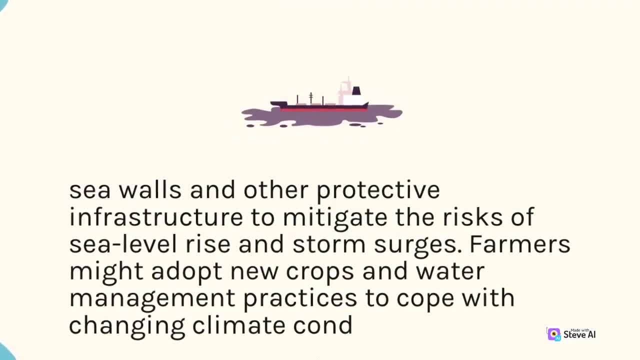 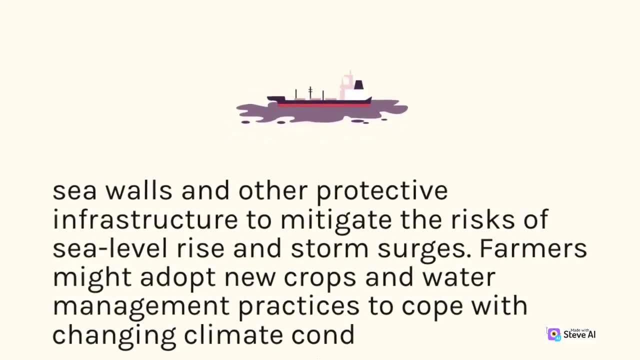 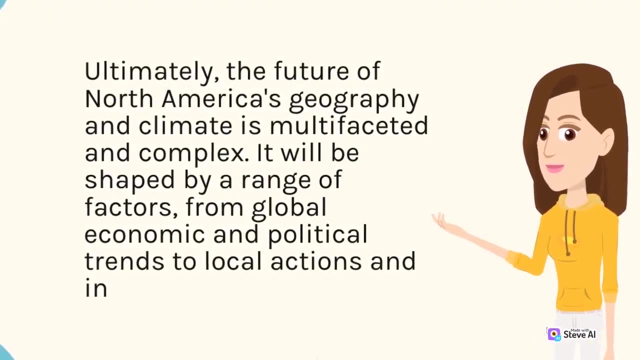 If this also me way, the new of the ặt at than the. The future of North America's geography and climate is multifaceted and complex. It will be shaped by a range of factors, from global economic and political trends to local actions and in. 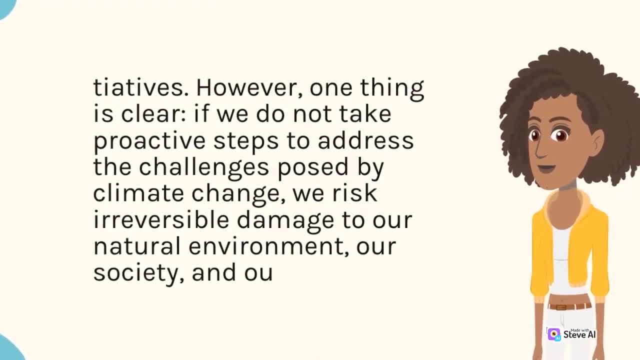 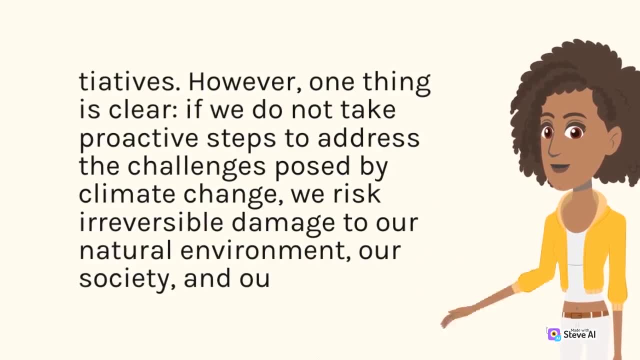 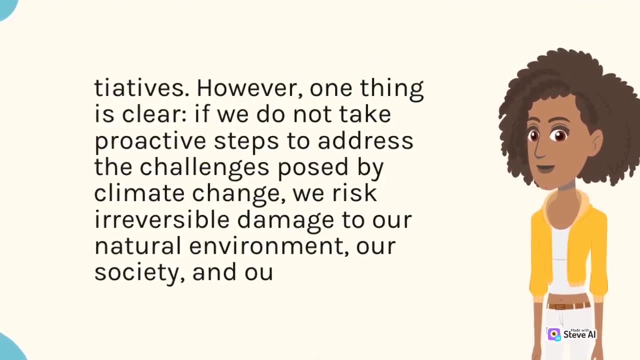 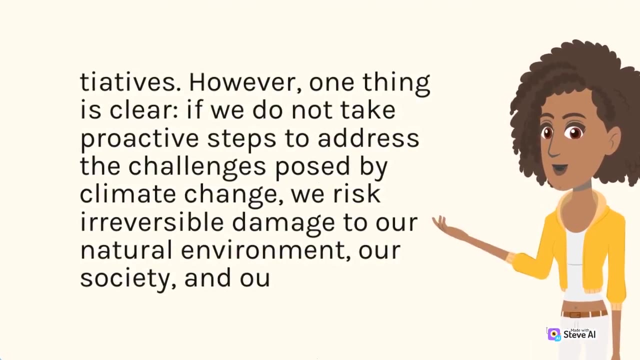 Shit-ives. However, one thing is clear: if we do not take proactive steps to address the challenges posed by climate change, we risk irreversible damage to our natural environment, our society and ew Shit-ives. However, one thing is clear: if we do not take proactive steps to address the challenges posed by climate change, we risk irreversible damage to our natural environment, our society and ew. 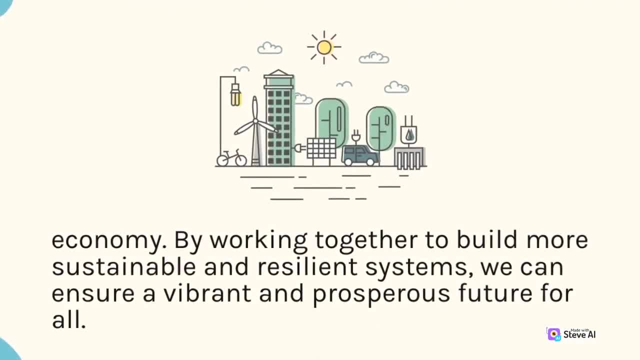 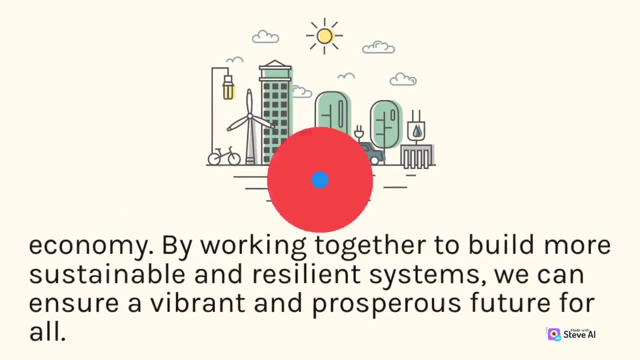 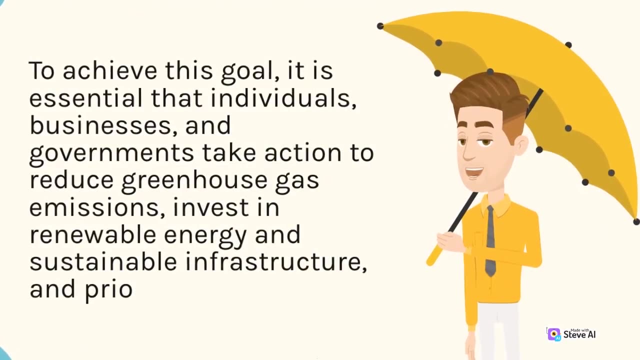 Economy. By working together to build more sustainable and resilient systems, we can ensure a vibrant and prosperous future for all. To achieve this goal, it is essential that individuals, businesses and governments take action to reduce greenhouse gas emissions, invest in renewable energy and sustainable infrastructure and pre-o. 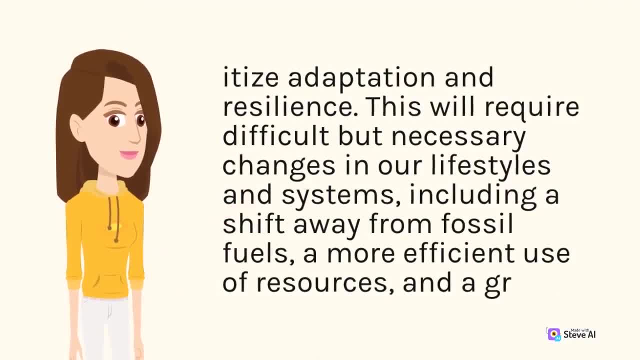 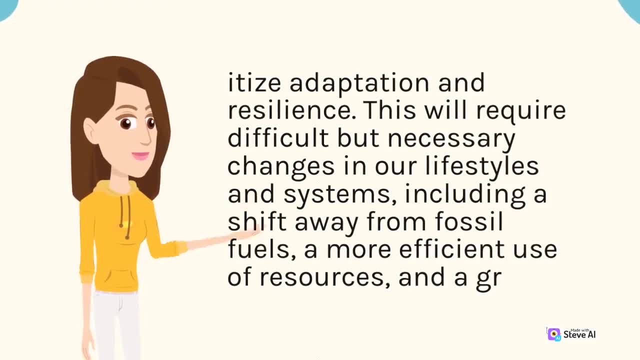 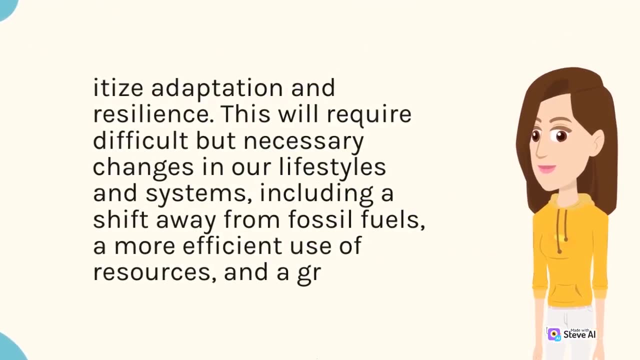 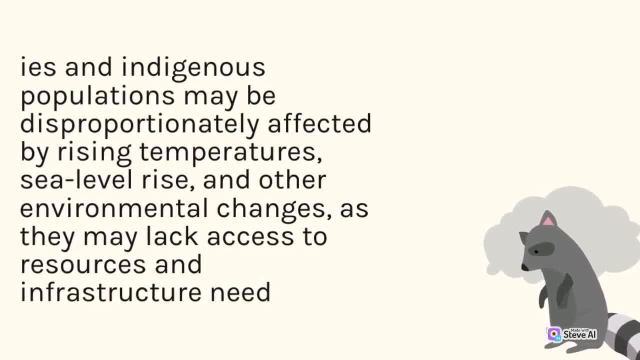 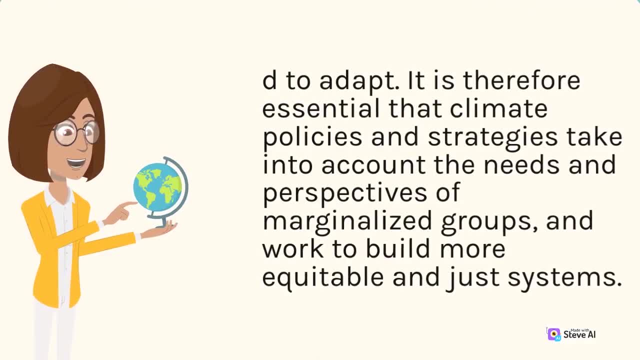 It ties adaptation and resilience. This will require difficult but necessary changes in our lifestyles and systems, including a GR. as they may lack access to resources and infrastructure need d To adapt. It is therefore essential that climate policies and strategies take into account the needs and perspectives of marginalized groups and work to build more equitable and just 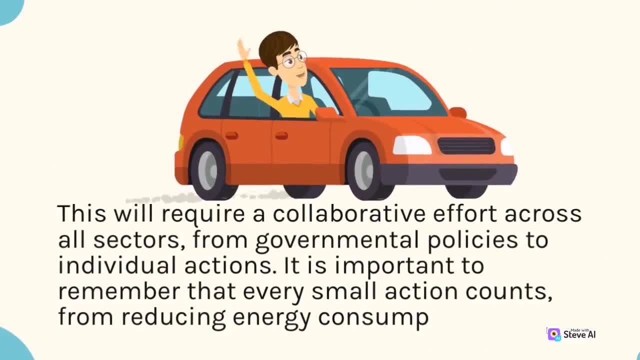 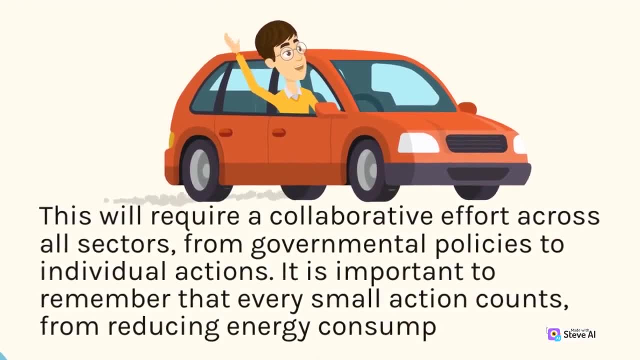 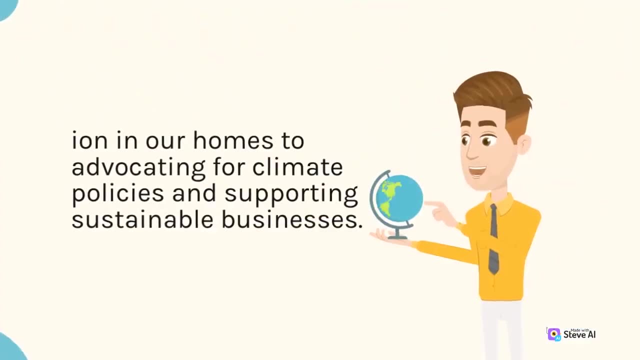 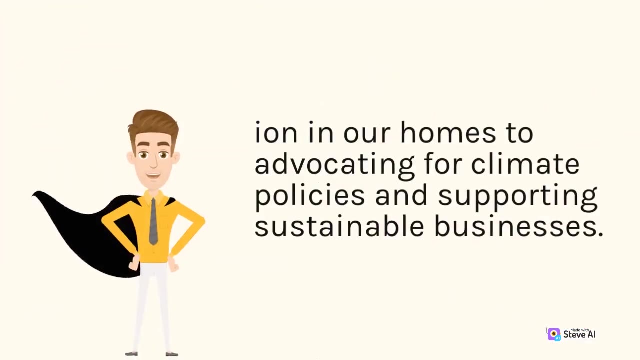 systems. This will require a collaborative effort across all sectors, from governmental policies to individual actions. It is important to remember that every small action counts, from reducing energy consump. ion in our homes to advocating for climate policies and supporting sustainable businesses. Ion in our homes to advocating for climate policies and supporting sustainable. 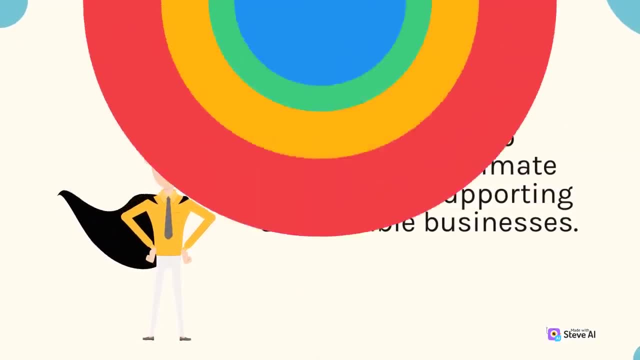 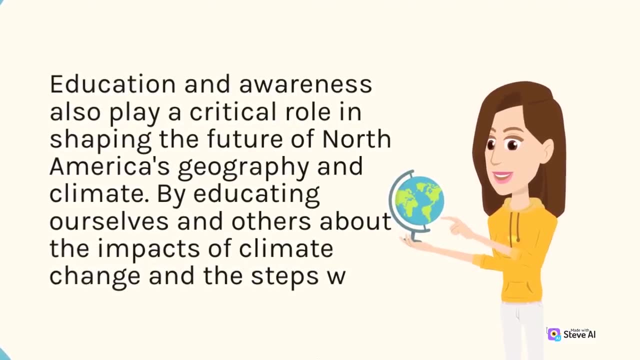 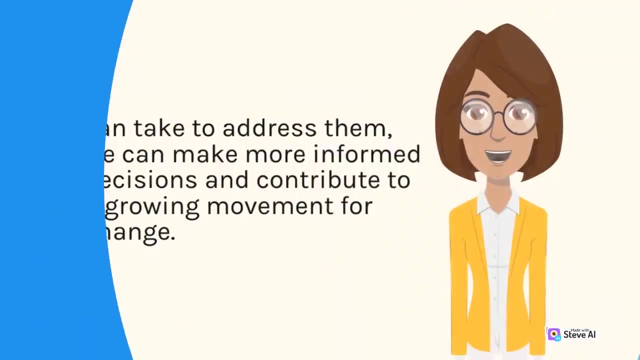 businesses. Education and awareness also play a critical role in shaping the future of North America's geography and climate. By educating ourselves and others about the impacts of climate change and the steps w? d Can take to address them, we can make more informed decisions and contribute to a growing movement for change. 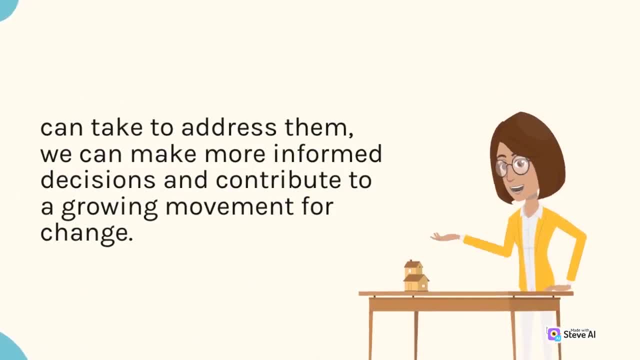 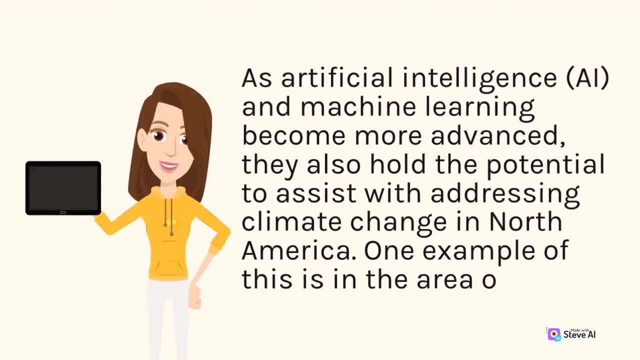 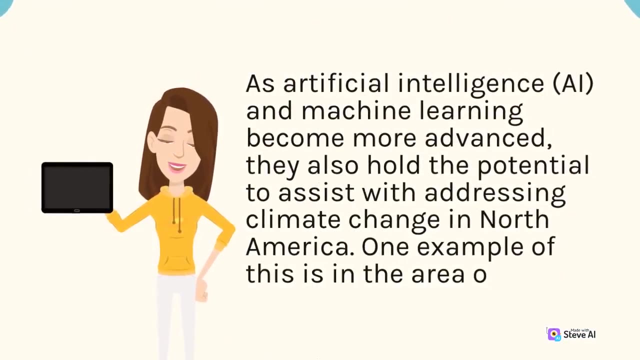 d Can take to address them. we can make more informed decisions and contribute to a growing movement for change. As artificial intelligence, AI and machine learning become more advanced, they also hold the potential to assist with addressing climate change in North America. One example of this is in the area O. 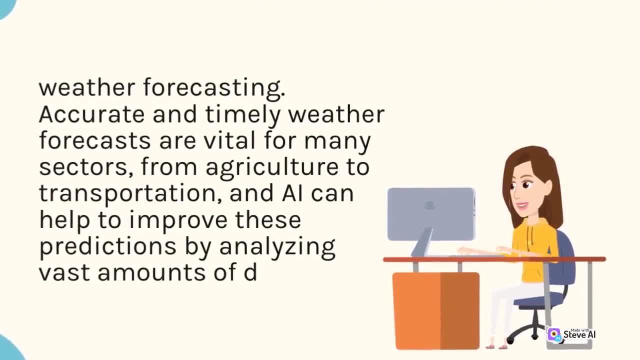 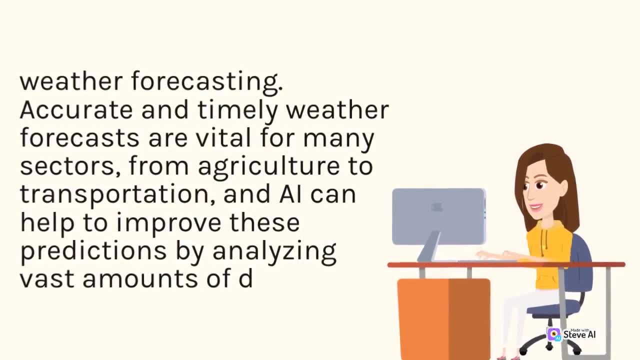 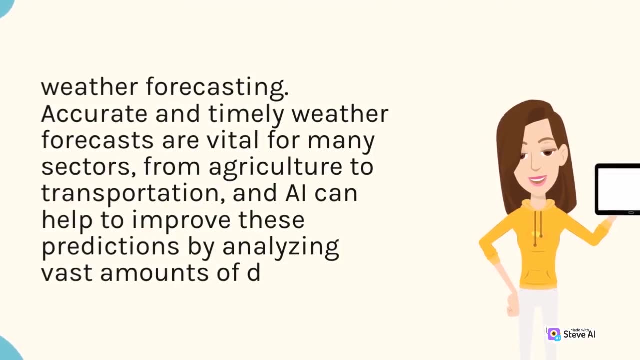 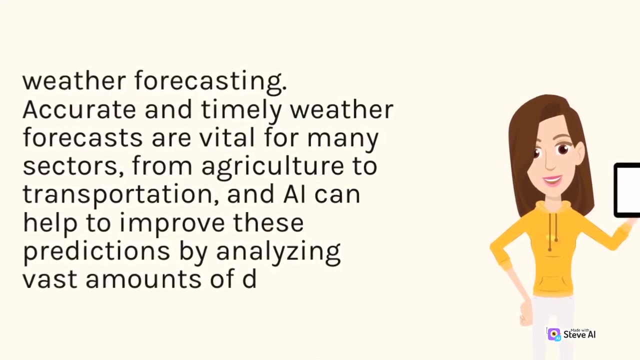 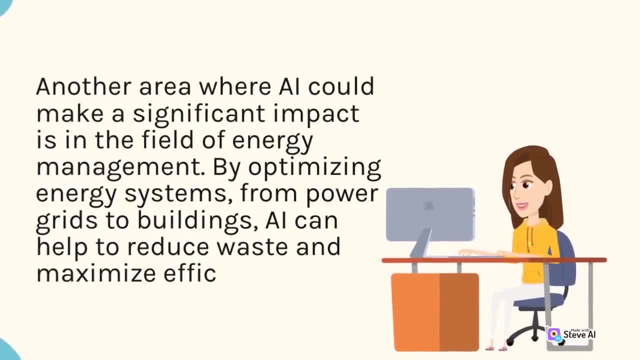 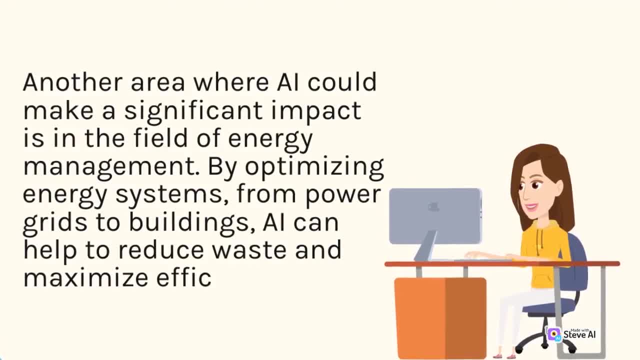 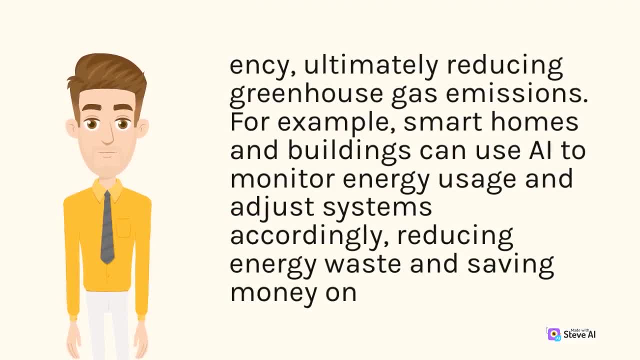 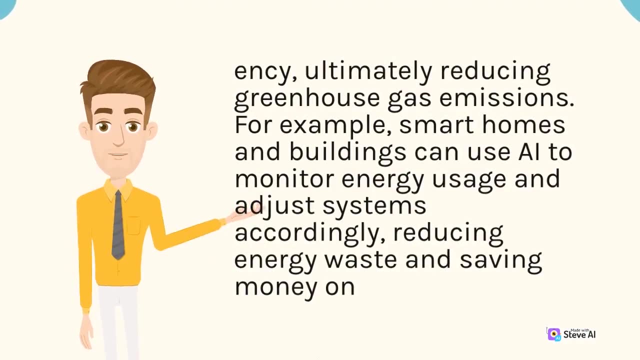 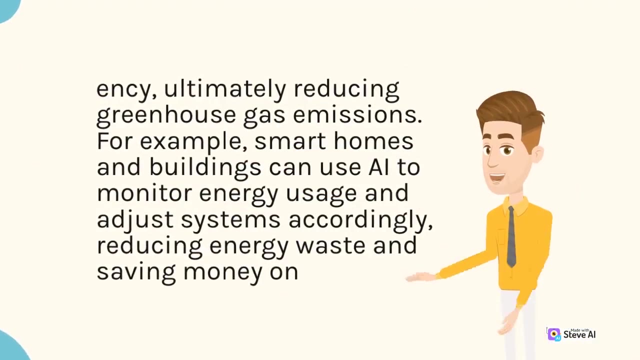 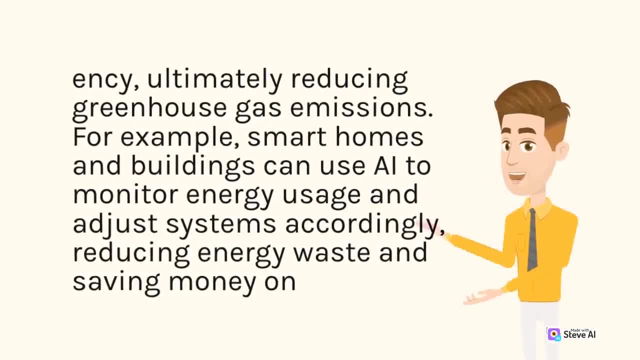 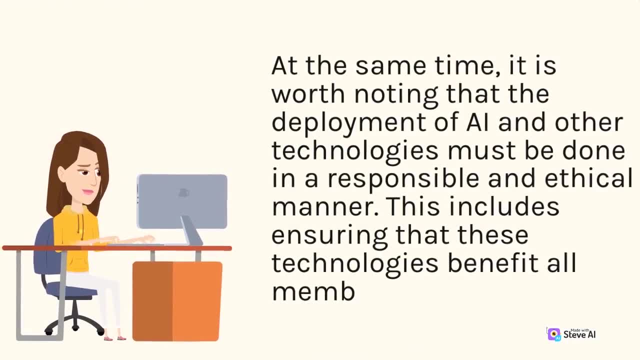 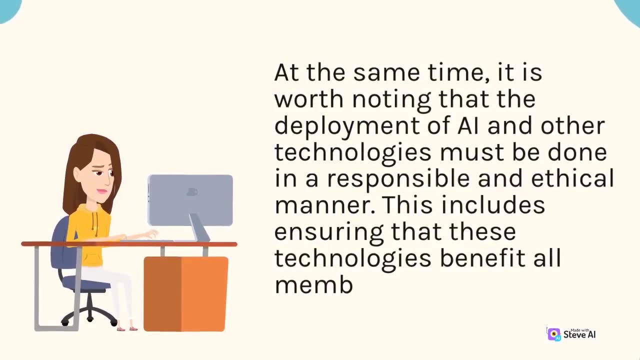 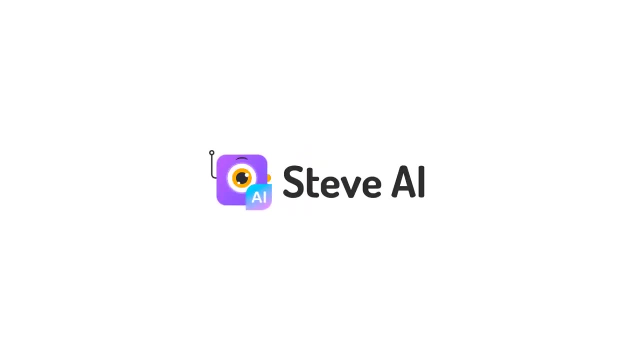 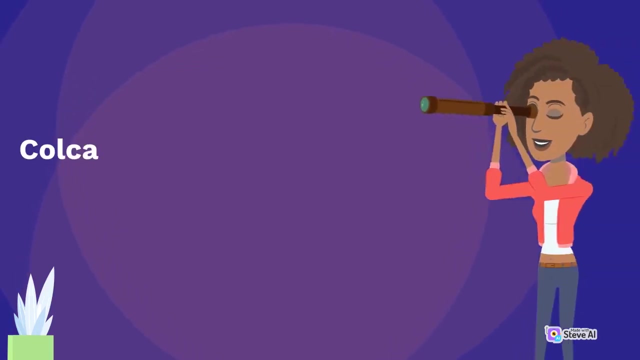 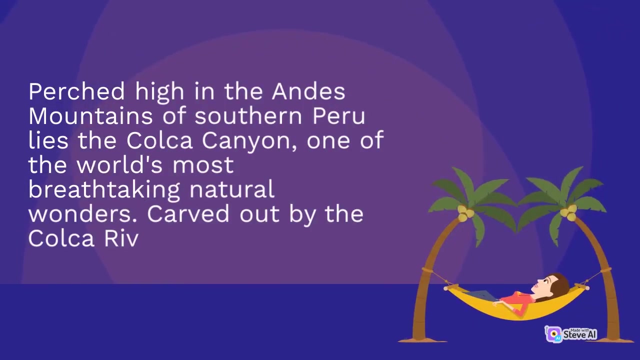 Ta and identifying patterns that human forecasters may make Ta and identifying patterns that human forecasters may make Kalka Canyon one of the deepest canyons in the world. Perched high in the Andes Mountains of southern Peru lies the Kalka Canyon, one of the world's most breathtaking natural wonders. 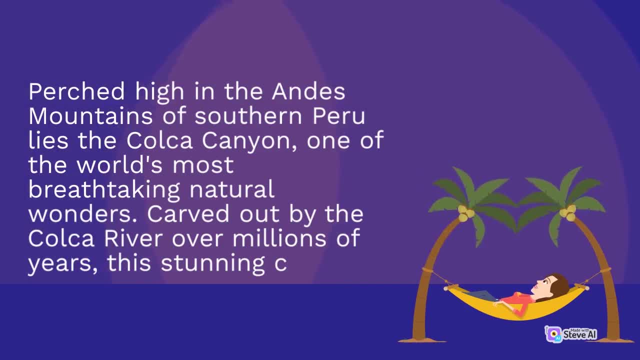 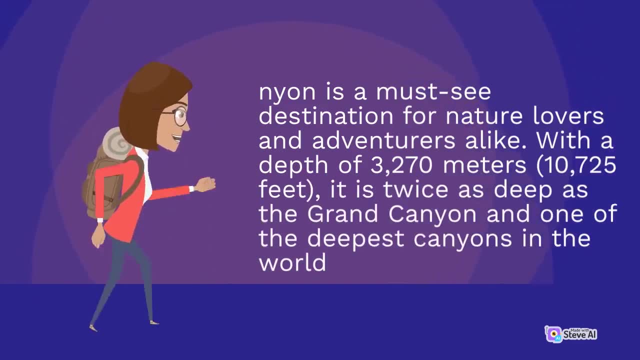 Carved out by the Kalka River over millions of years, this stunning sea Neon is a must-see destination for nature lovers and adventurers alike. With a depth of 3,270 meters- 10,725 feet, it is twice as deep as the Grand Canyon and one of the deepest canyons in the world. 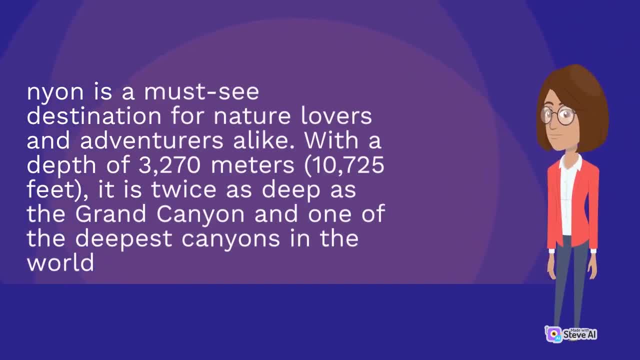 Neon is a must-see destination for nature lovers and adventurers alike. With a depth of 3,270 meters- 10,725 feet, it is twice as deep as the Grand Canyon and one of the deepest canyons in the world. 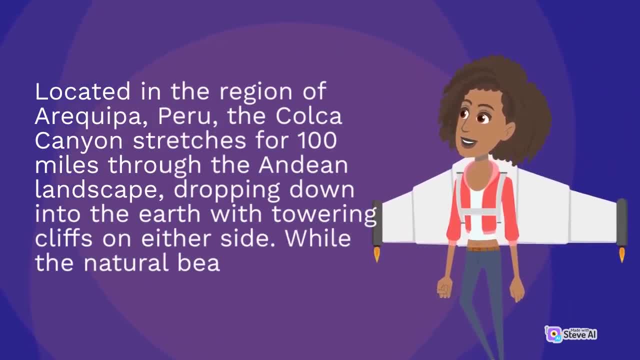 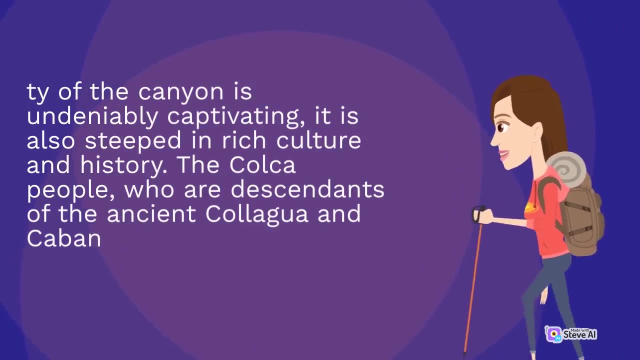 Located in the region of Arequipa, Peru, the Kalka Canyon stretches for 100 miles through the Andean landscape, dropping down into the earth, with towering cliffs on either side. While the natural B tie of the canyon is undeniably captivating, it is also steeped in rich culture and history. 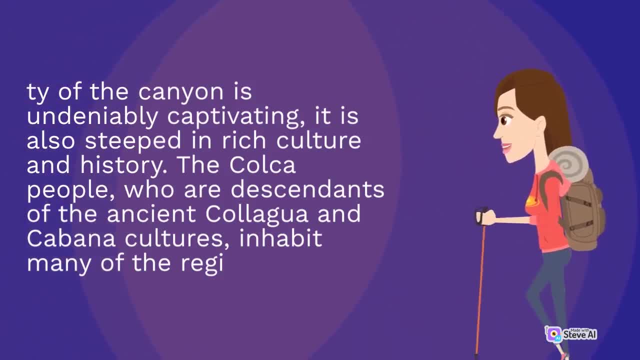 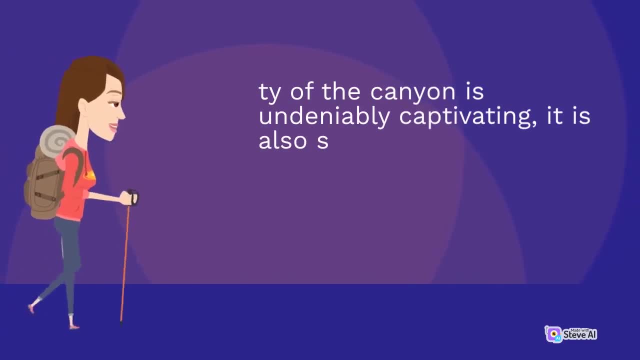 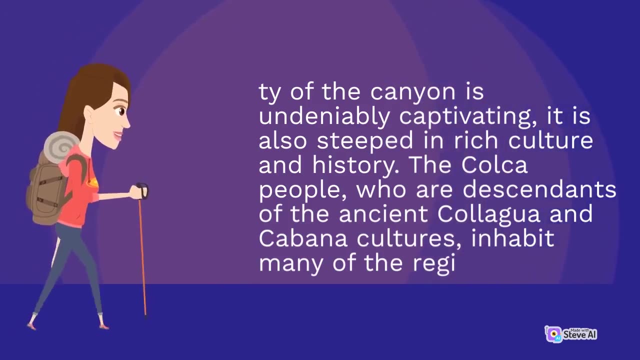 The Kalka people, who are descendants of the ancient Kalagua and Cabana cultures, inhabit many of the Regi. The Kalka people, who are descendants of the ancient Kalagua and Cabana cultures, inhabit many of the Regi. 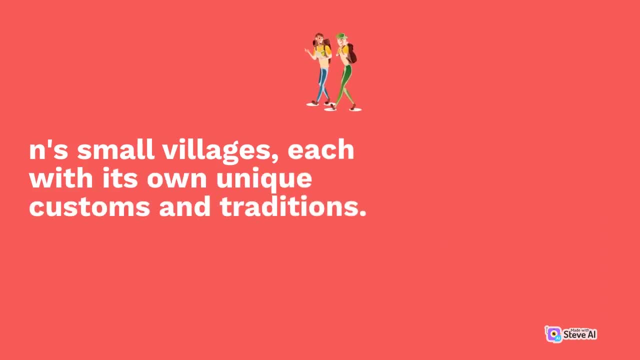 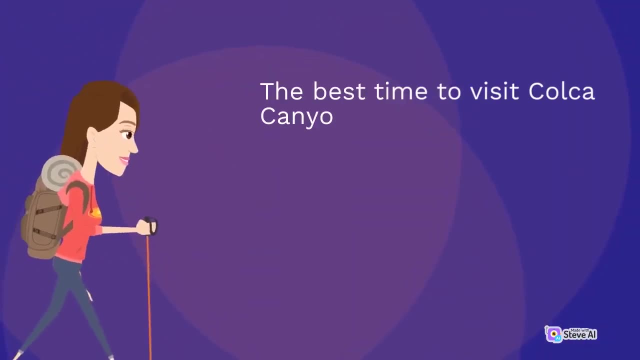 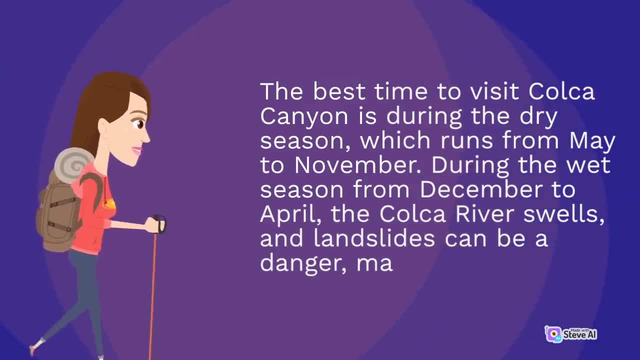 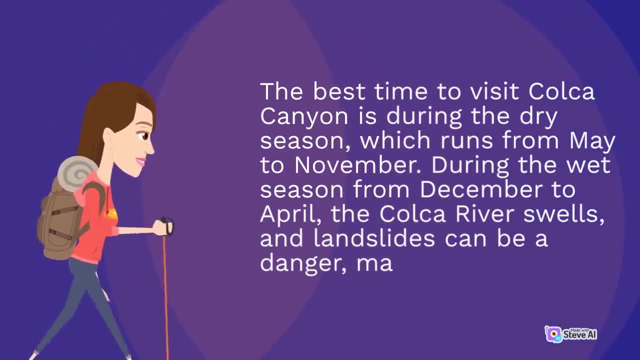 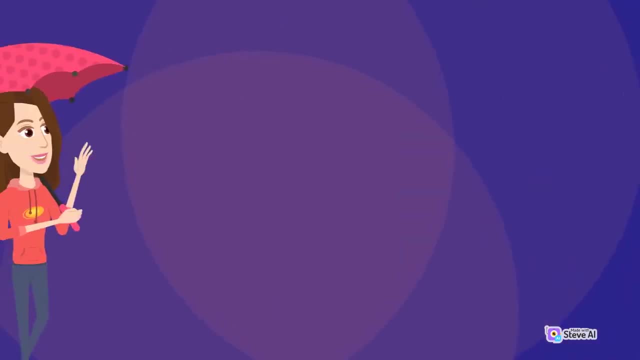 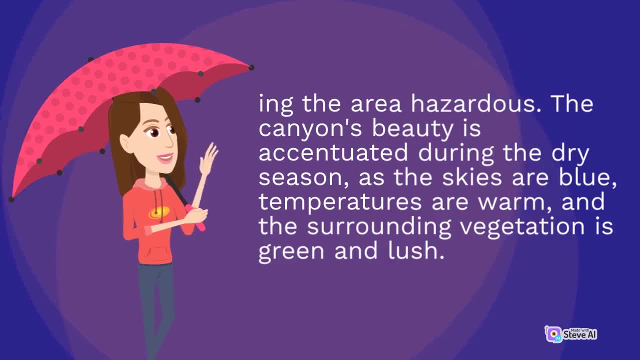 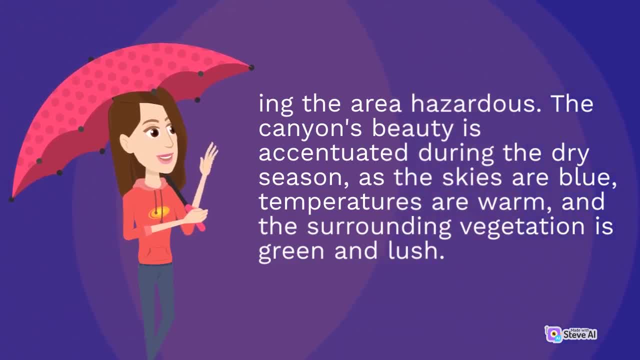 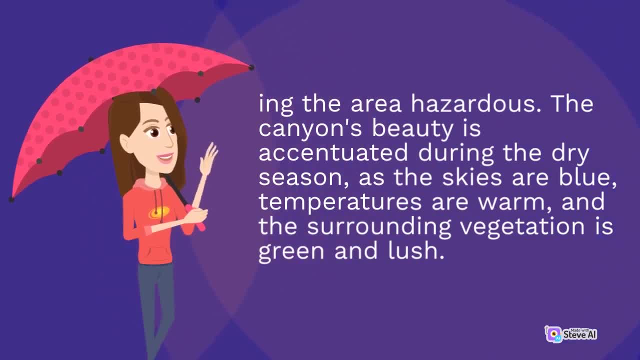 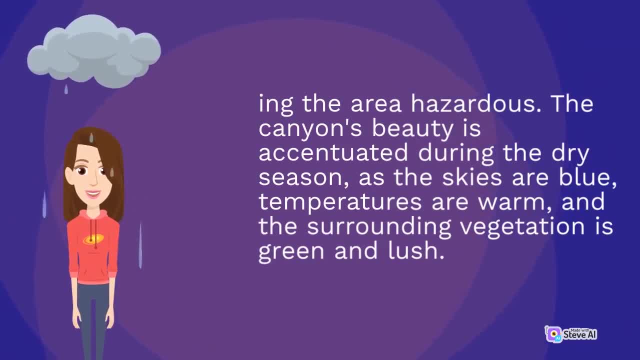 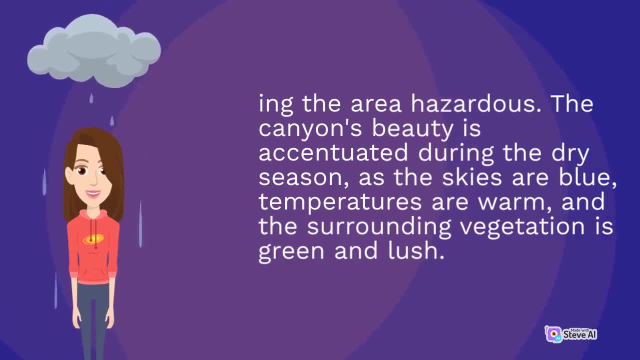 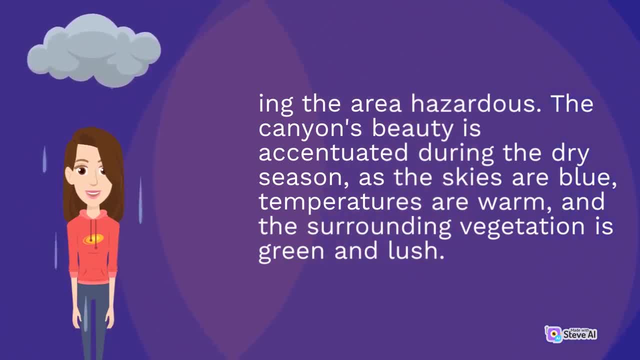 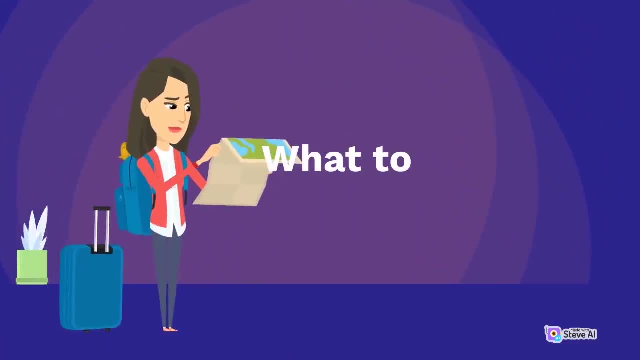 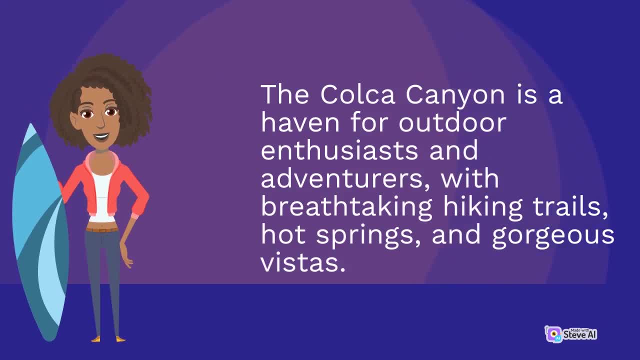 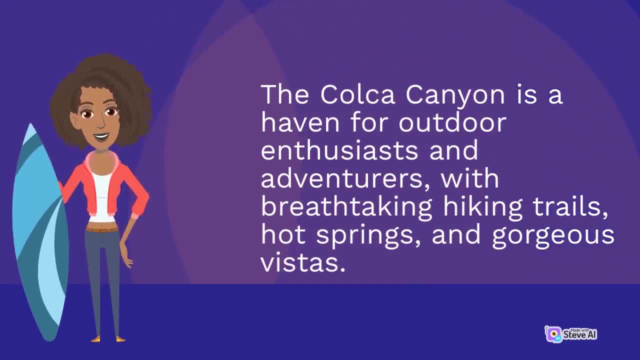 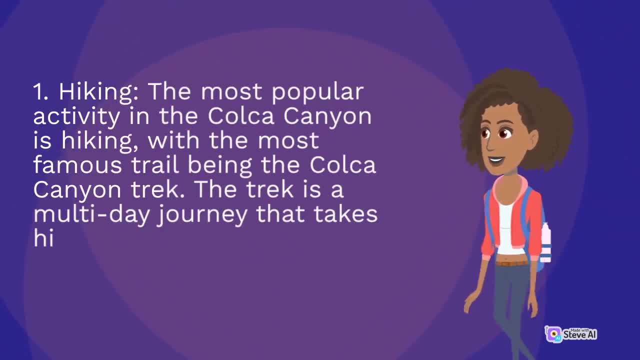 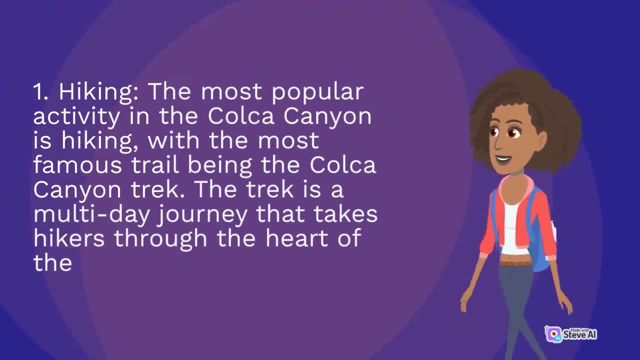 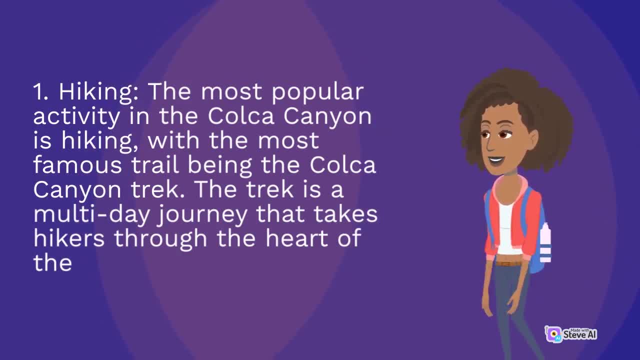 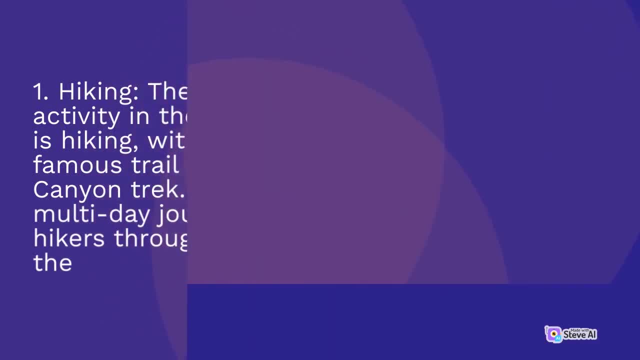 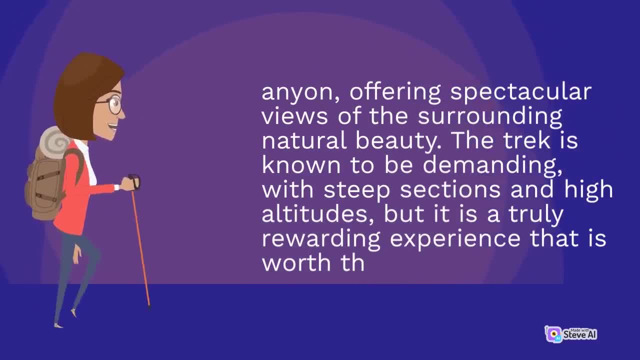 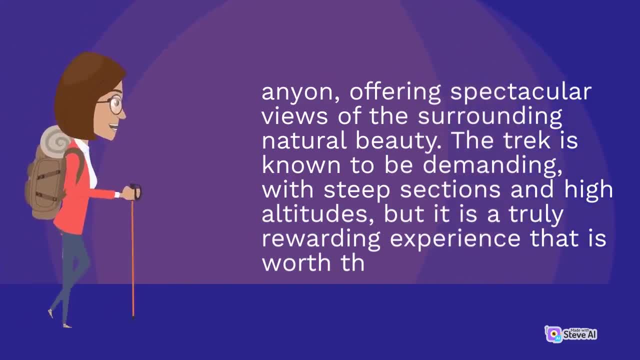 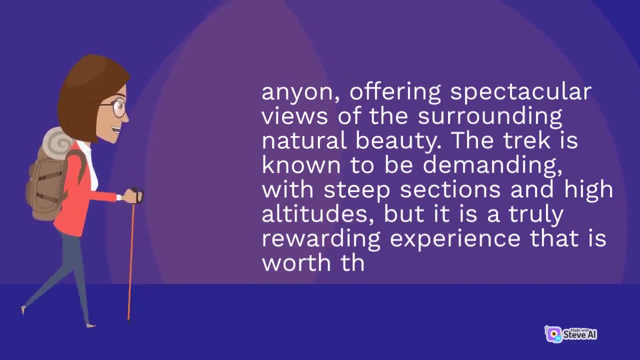 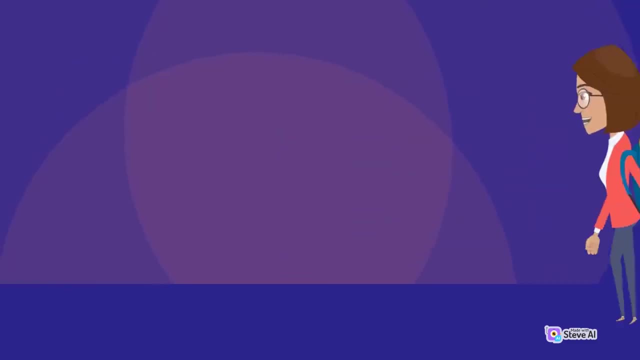 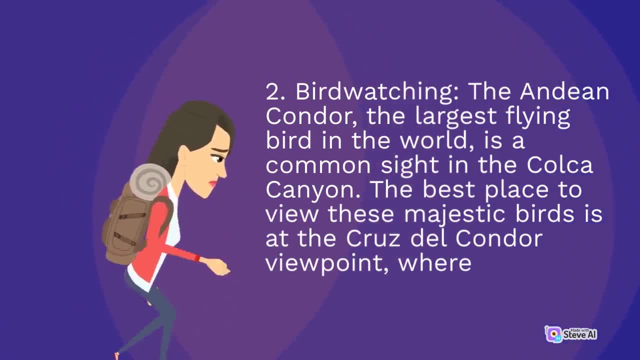 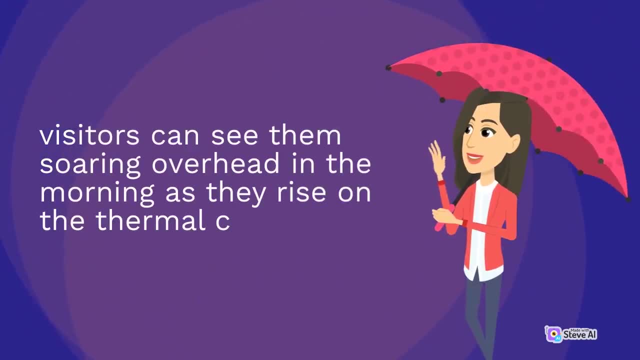 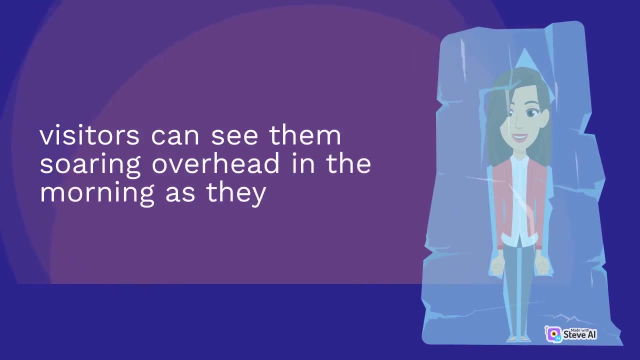 The best place to view these majestic birds is at the Cruz del Condor viewpoint, Where Visitors can see them soaring overhead in the morning as they rise on the thermal currents. Visitors can see them soaring overhead in the morning as they rise on the thermal currents. 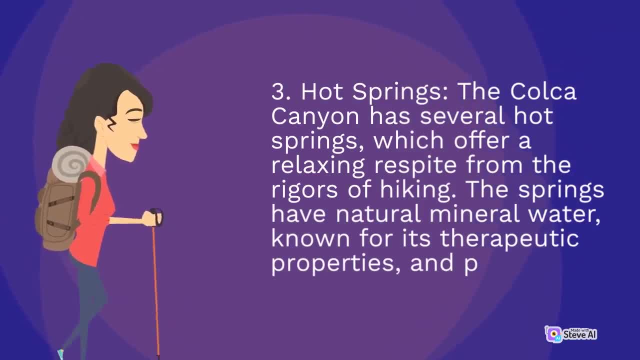 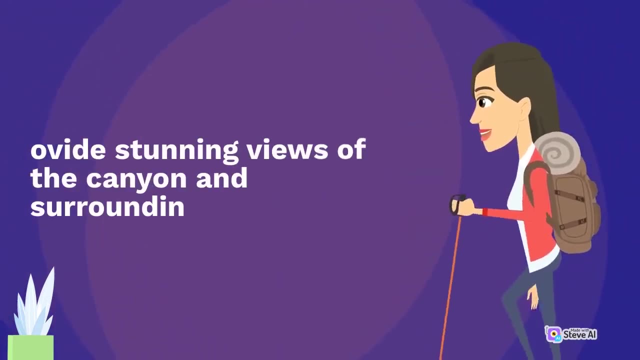 3. Hot Springs. The Kalka Canyon has several hot springs which offer a relaxing respite from the rigors of hiking. The springs have natural mineral water, known for its therapeutic properties, and p Ovidie, Stunning views of the canyon and surrounding landscape. 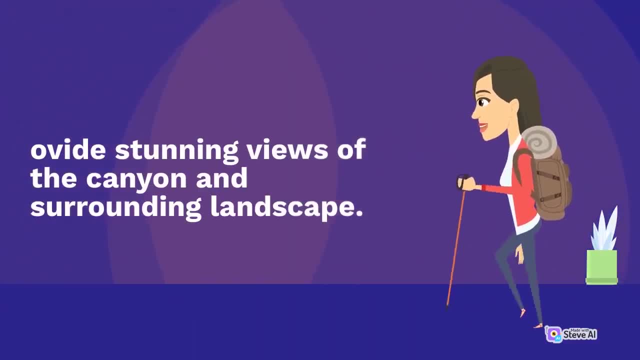 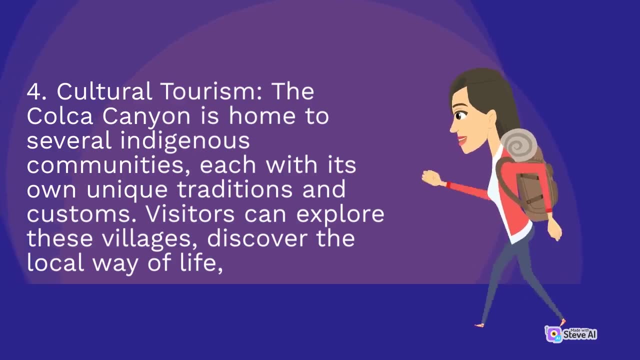 Ovidie, Stunning views of the canyon and surrounding landscape. 4. Cultural Tourism: The Kalka Canyon is home to several Indigenous communities, each with its own unique traditions and customs. Visitors can explore these villages, discover the local way of life ND immerse themselves in Andean culture. 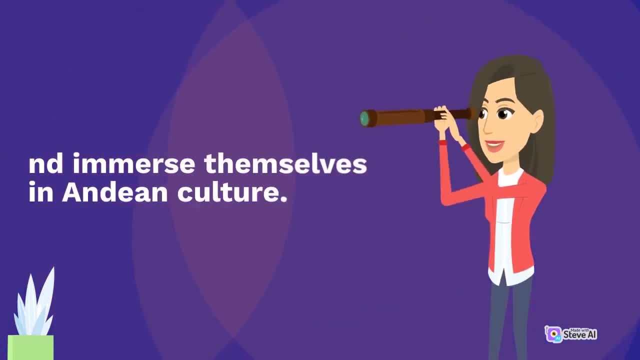 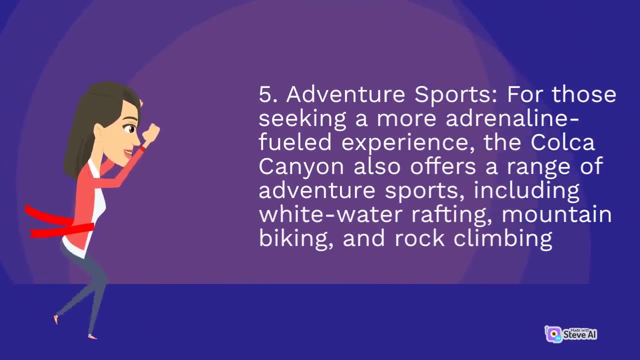 ND immerse themselves in Andean culture. 5. Adventure Sports: For those seeking a more adrenaline-fueled experience, the Kalka Canyon also offers a range of adventure sports, including whitewater rafting, mountain biking and rock climbing. 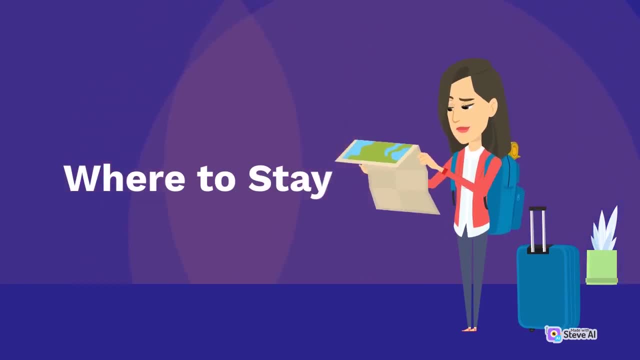 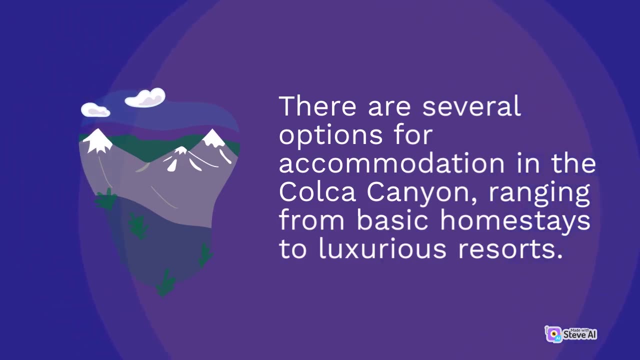 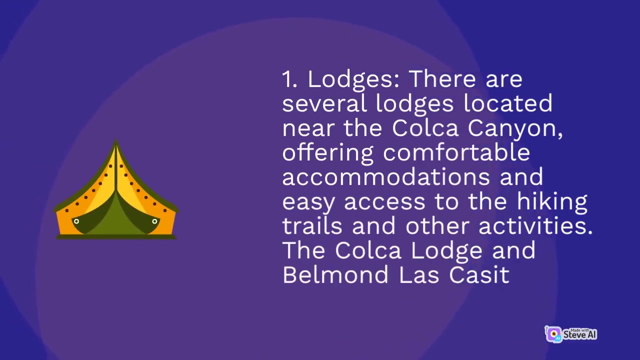 Where to Stay. There are several options for accommodation in the Kalka Canyon, ranging from basic homestays to luxurious resorts. 1. Lodges: There are several lodges located near the Kalka Canyon, offering comfortable accommodations and easy access to the hiking trails and other activities: The Kalka Lodge and Belmond Blas Casete. 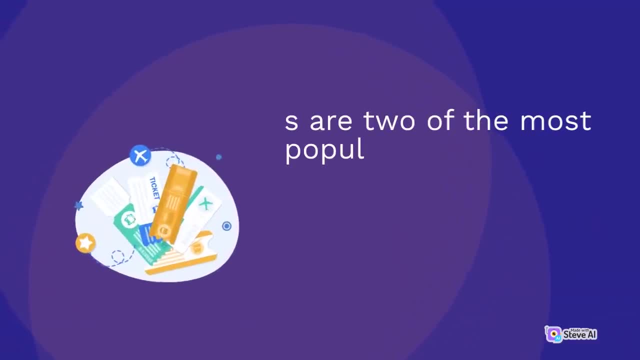 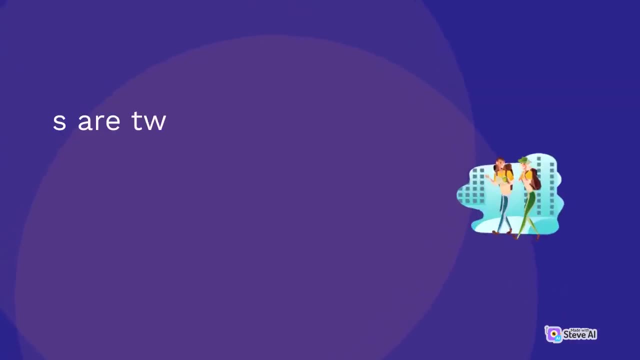 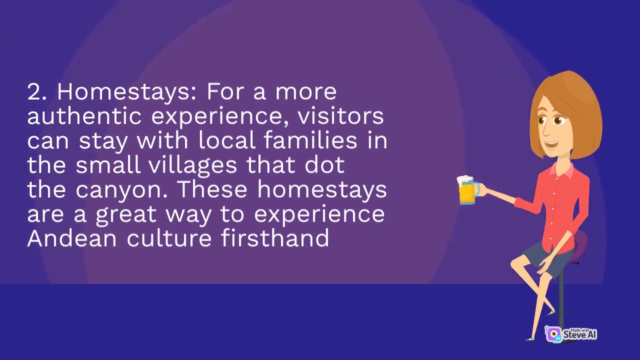 S are two of the most popular options, offering a range of amenities and services. 2. Homestays: For a more authentic experience, visitors can stay with local families in the small villages that dot the canyon. These homestays are a great way to experience Andean culture firsthand. 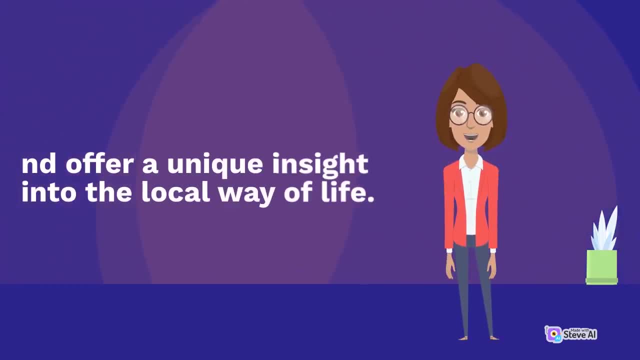 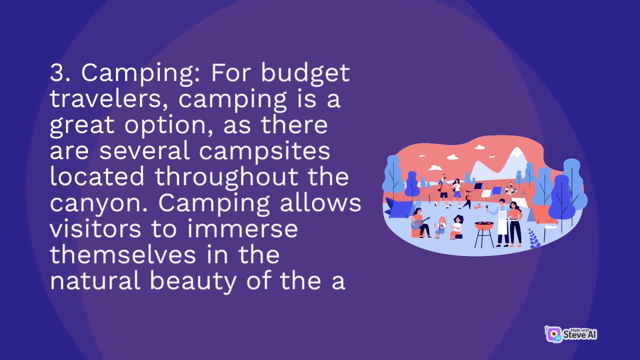 ND offer a unique insight into the local way of life. 3. Camping For budget travelers. camping is a great option as there are several campsites located throughout the canyon. Camping allows visitors to immerse themselves in the natural beauty of the A. 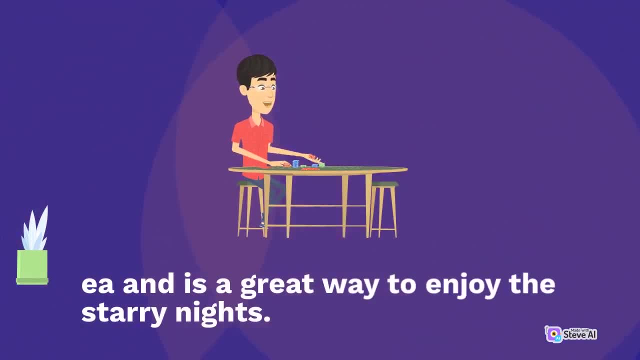 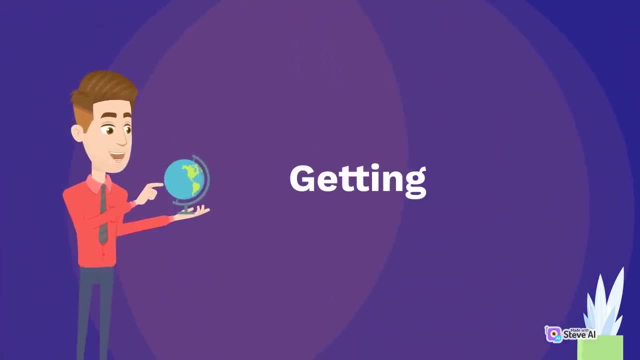 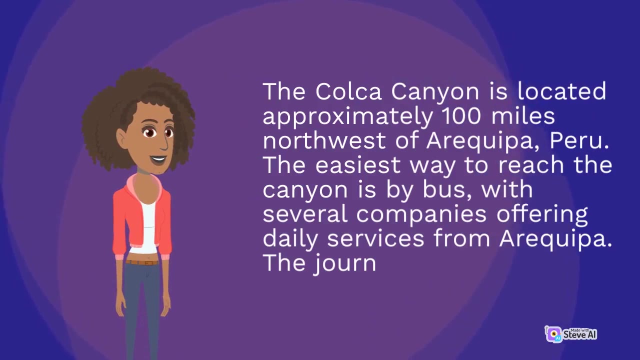 Ea and N is a great way to enjoy the starry nights. Getting There: The Calca Canyon is located approximately 100 miles northwest of Arequipa, Peru. The easiest way to reach the canyon is by bus, with several companies offering daily services from Arequipa. The Jern Wai takes approximately 4 hours, passing through stunning Andean landscapes and small towns. Alternatively, visitors can hire a private car or take a guided tour. The Calca Canyon is not only a remarkable natural wonder, but also a testament to the enduring cultural heritage of the Andean people. 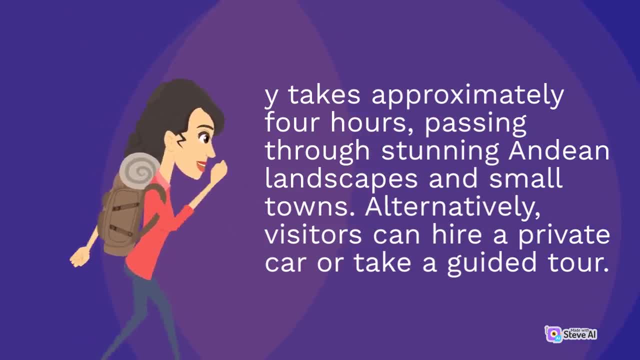 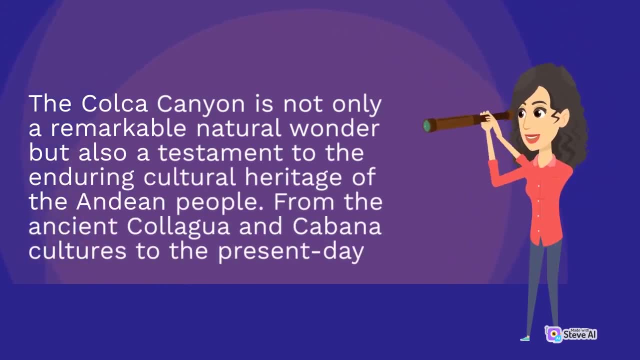 From the ancient Calagua and Cabana cultures to the present day Alcapipa. the region's most important cultural heritage is the indigenous culture of the Andean people. The Andean people have been the most important cultural heritage of the Andean people for centuries. 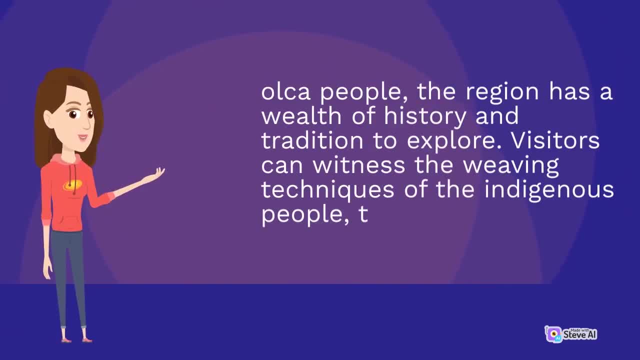 The Andean people have been the most important cultural heritage of the Andean people for centuries. The region has a wealth of history and tradition to explore. Visitors can witness the weaving techniques of the indigenous people. try traditional foods such as kui, guinea pig and li. 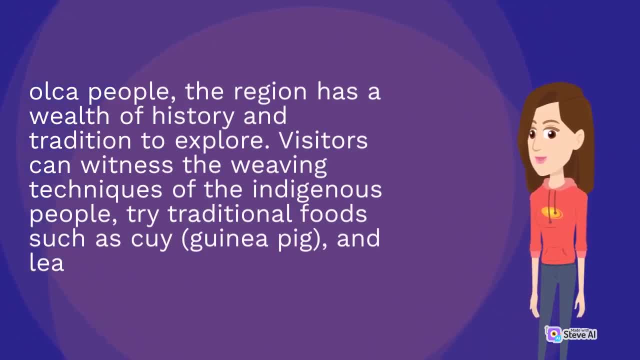 Alcapipa. the region has a wealth of history and tradition to explore. Visitors can witness the weaving techniques of the indigenous people, try traditional foods such as kui, guinea pig and li, And about the medicinal plants of the region. 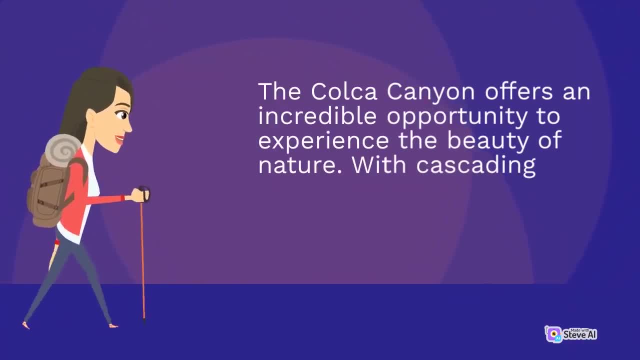 Visitors can witness the weaving techniques of the Andean people, try traditional foods such as kui guinea pig and li Alcapipa. the region has a wealth of history and tradition to explore. Visitors can witness the weaving techniques of the Andean people, try traditional foods such as kui guinea pig and li. 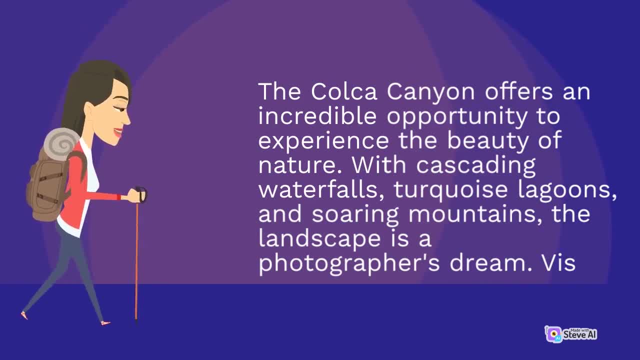 Alcapipa. the region has a wealth of history and tradition to explore. Visitors can witness the weaving techniques of the Andean people, try traditional foods such as kui, guinea pig and li Alcapipa. the region has a wealth of history and tradition to explore. 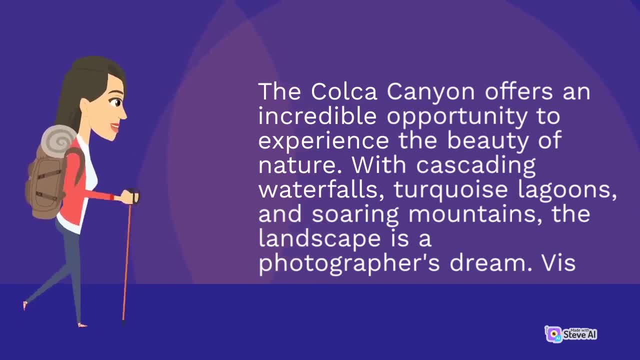 Visitors can witness the weaving techniques of the Andean people, try traditional foods such as kui guinea pig and li Alcapipa. the region has a wealth of history and tradition to explore. Visitors can witness the weaving techniques of the Andean people, try traditional foods such as kui guinea pig and li. 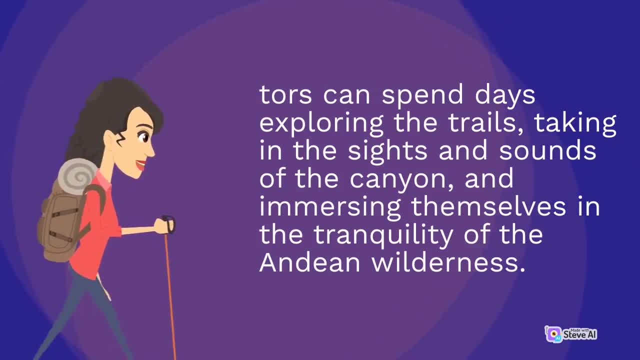 Alcapipa. the region has a wealth of history and tradition to explore. Visitors can witness the weaving techniques of the Andean people, try traditional foods such as kui, guinea pig and li Alcapipa. the region has a wealth of history and tradition to explore. 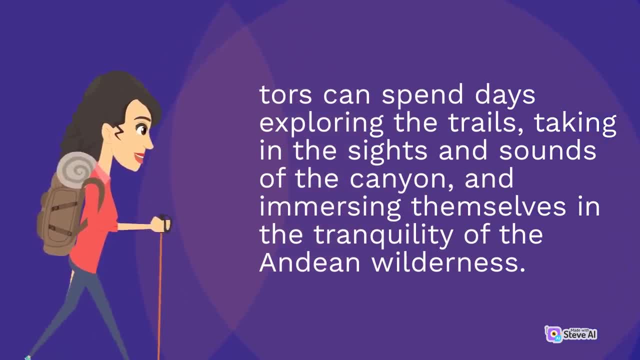 Visitors can witness the weaving techniques of the Andean people, try traditional foods such as kui guinea pig and li Alcapipa. the region has a wealth of history and tradition to explore. Visitors can witness the weaving techniques of the Andean people, try traditional foods such as kui guinea pig and li. 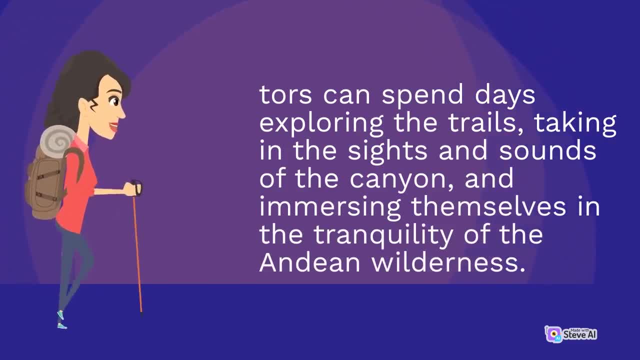 Alcapipa. the region has a wealth of history and tradition to explore. Visitors can witness the weaving techniques of the Andean people, try traditional foods such as kui, guinea pig and li Alcapipa. the region has a wealth of history and tradition to explore. 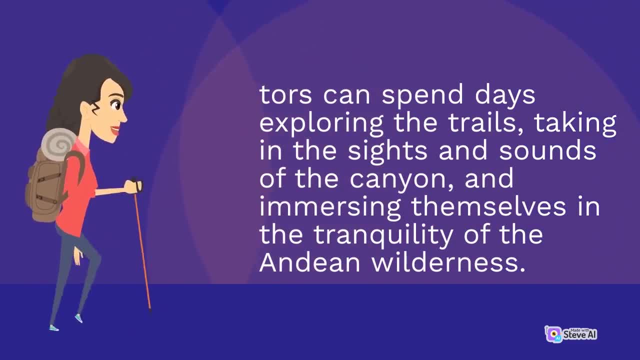 Visitors can witness the weaving techniques of the Andean people, try traditional foods such as kui guinea pig and li Alcapipa. the region has a wealth of history and tradition to explore. Visitors can witness the weaving techniques of the Andean people, try traditional foods such as kui guinea pig and li. 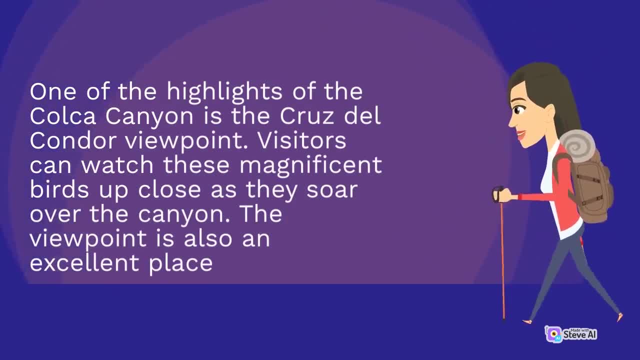 Alcapipa. the region has a wealth of history and tradition to explore. Visitors can witness the weaving techniques of the Andean people, try traditional foods such as kui, guinea pig and li Alcapipa. the region has a wealth of history and tradition to explore. 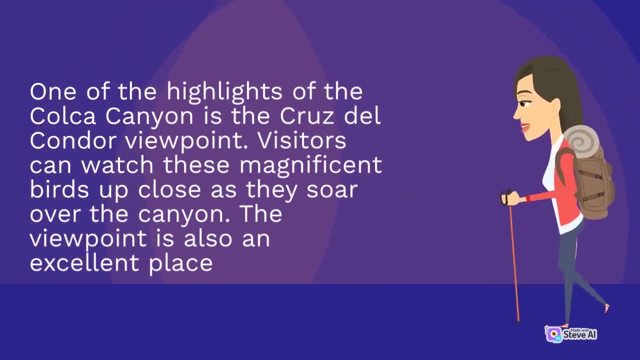 Visitors can witness the weaving techniques of the Andean people, try traditional foods such as kui guinea pig and li Alcapipa. the region has a wealth of history and tradition to explore. Visitors can witness the weaving techniques of the Andean people, try traditional foods such as kui guinea pig and li. 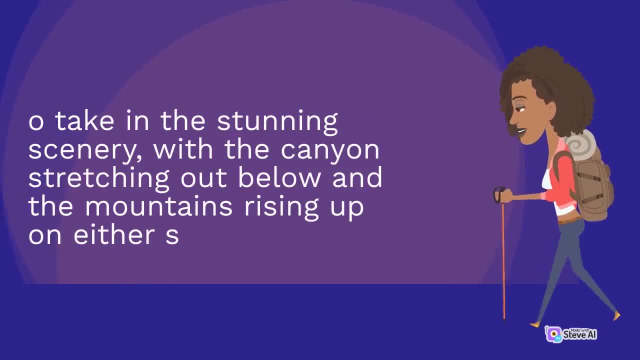 Alcapipa. the region has a wealth of history and tradition to explore. Visitors can witness the weaving techniques of the Andean people, try traditional foods such as kui, guinea pig and li Alcapipa. the region has a wealth of history and tradition to explore. 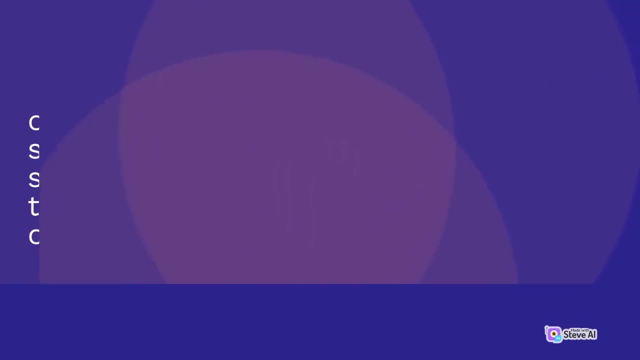 Visitors can witness the weaving techniques of the Andean people, try traditional foods such as kui guinea pig and li Alcapipa. the region has a wealth of history and tradition to explore. Visitors can witness the weaving techniques of the Andean people, try traditional foods such as kui guinea pig and li. 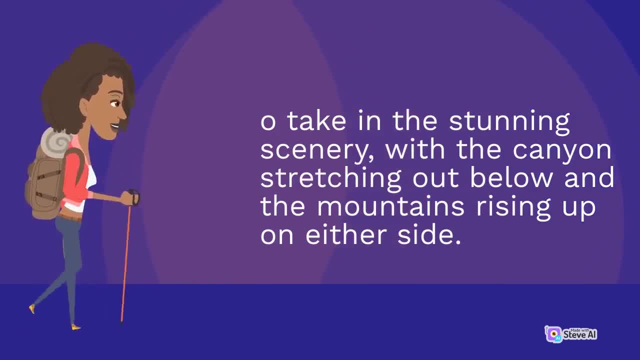 Alcapipa. the region has a wealth of history and tradition to explore. Visitors can witness the weaving techniques of the Andean people, try traditional foods such as kui, guinea pig and li Alcapipa. the region has a wealth of history and tradition to explore. 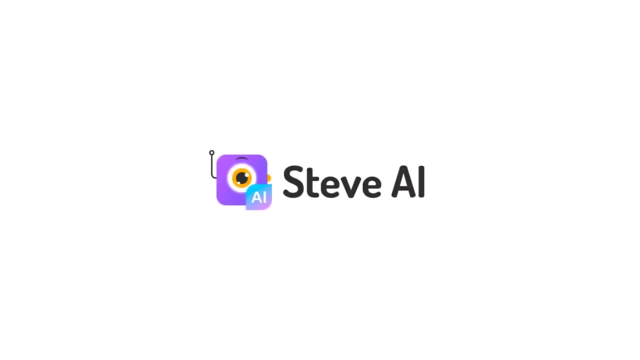 Visitors can witness the weaving techniques of the Andean people, try traditional foods such as kui guinea pig and li Alcapipa. the region has a wealth of history and tradition to explore. Visitors can witness the weaving techniques of the Andean people, try traditional foods such as kui guinea pig and li. 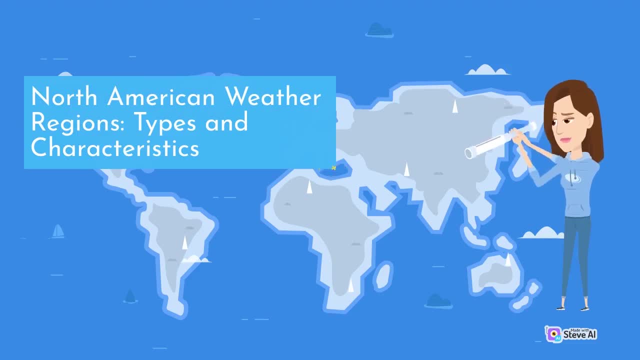 Alcapipa. the region has a wealth of history and tradition to explore. Visitors can witness the weaving techniques of the Andean people, try traditional foods such as kui, guinea pig and li Alcapipa. the region has a wealth of history and tradition to explore. 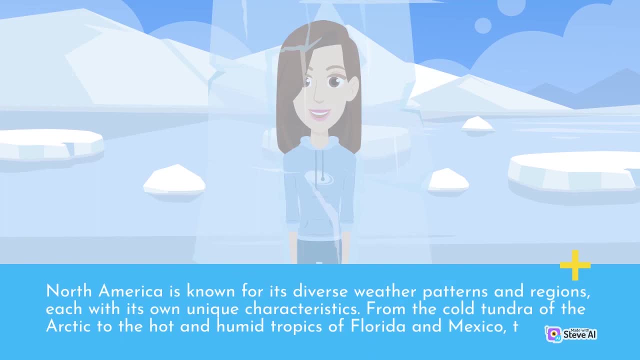 Visitors can witness the weaving techniques of the Andean people, try traditional foods such as kui guinea pig and li Alcapipa. the region has a wealth of history and tradition to explore. Visitors can witness the weaving techniques of the Andean people, try traditional foods such as kui guinea pig and li. 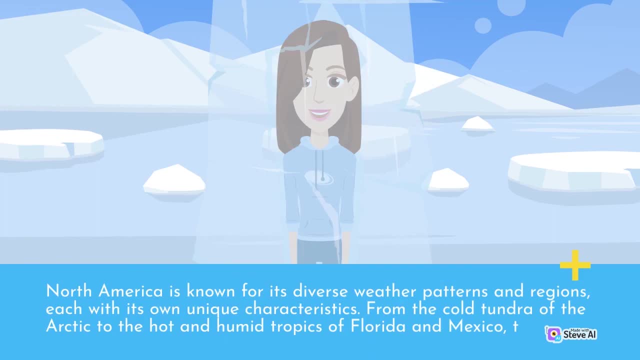 Alcapipa. the region has a wealth of history and tradition to explore. Visitors can witness the weaving techniques of the Andean people, try traditional foods such as kui, guinea pig and li Alcapipa. the region has a wealth of history and tradition to explore. 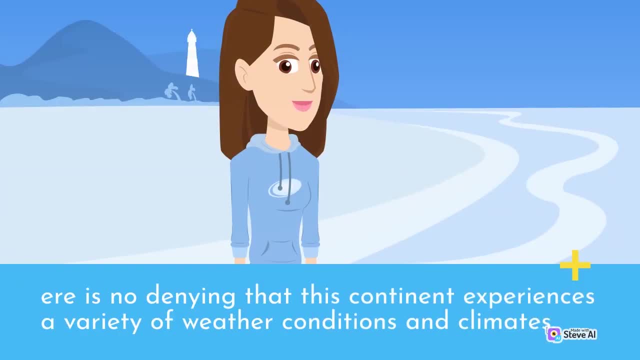 Visitors can witness the weaving techniques of the Andean people, try traditional foods such as kui guinea pig and li Alcapipa. the region has a wealth of history and tradition to explore. Visitors can witness the weaving techniques of the Andean people, try traditional foods such as kui guinea pig and li. 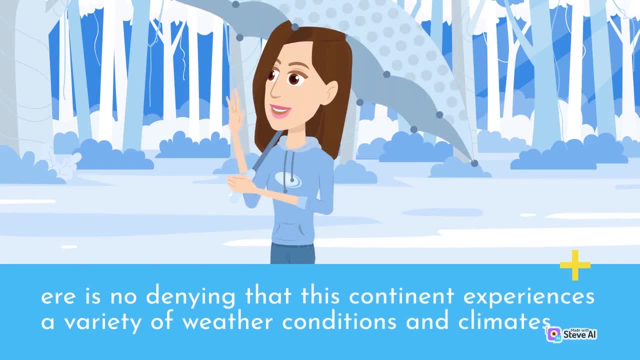 Alcapipa. the region has a wealth of history and tradition to explore. Visitors can witness the weaving techniques of the Andean people, try traditional foods such as kui, guinea pig and li Alcapipa. the region has a wealth of history and tradition to explore. 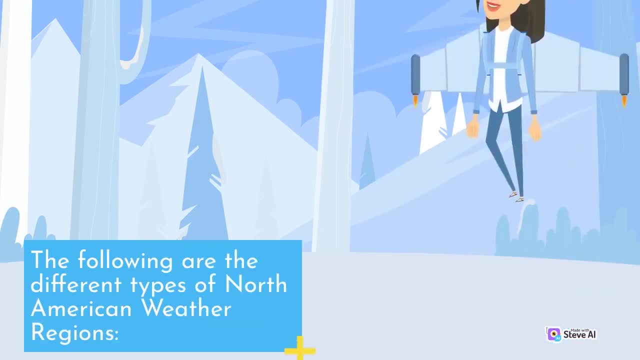 Visitors can witness the weaving techniques of the Andean people, try traditional foods such as kui guinea pig and li Alcapipa. the region has a wealth of history and tradition to explore. Visitors can witness the weaving techniques of the Andean people, try traditional foods such as kui guinea pig and li. 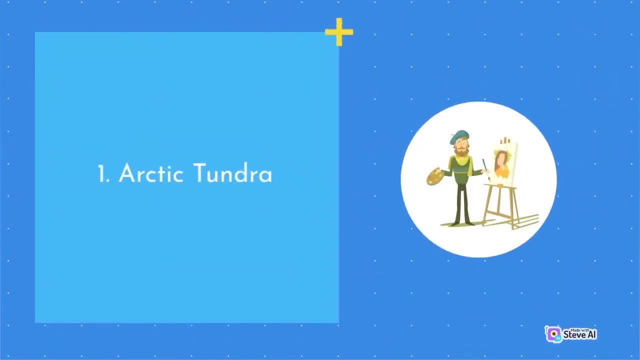 Alcapipa. the region has a wealth of history and tradition to explore. Visitors can witness the weaving techniques of the Andean people, try traditional foods such as kui, guinea pig and li Alcapipa. the region has a wealth of history and tradition to explore. 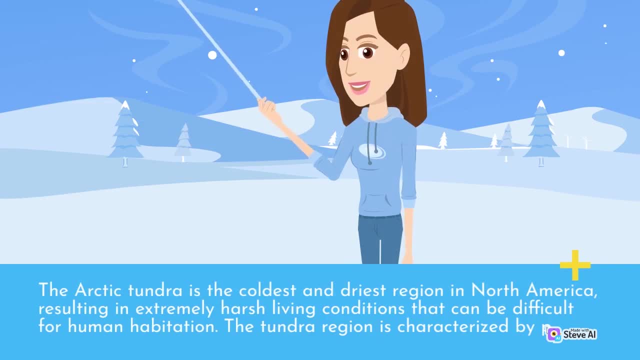 Visitors can witness the weaving techniques of the Andean people, try traditional foods such as kui guinea pig and li Alcapipa. the region has a wealth of history and tradition to explore. Visitors can witness the weaving techniques of the Andean people, try traditional foods such as kui guinea pig and li. 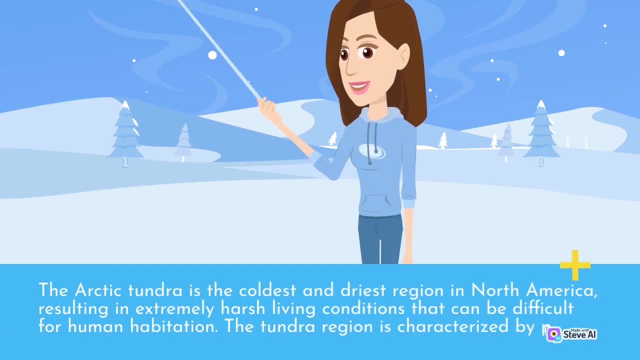 Alcapipa. the region has a wealth of history and tradition to explore. Visitors can witness the weaving techniques of the Andean people, try traditional foods such as kui, guinea pig and li Alcapipa. the region has a wealth of history and tradition to explore. 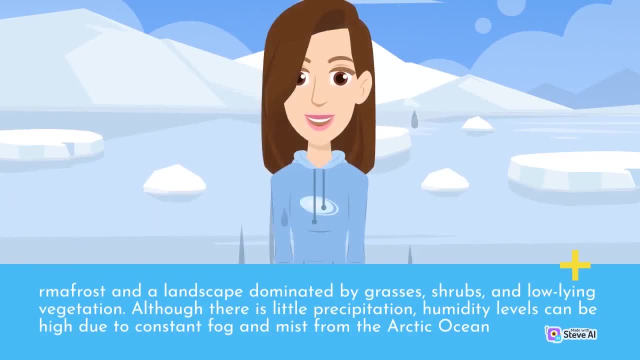 Visitors can witness the weaving techniques of the Andean people, try traditional foods such as kui guinea pig and li Alcapipa. the region has a wealth of history and tradition to explore. Visitors can witness the weaving techniques of the Andean people, try traditional foods such as kui guinea pig and li. 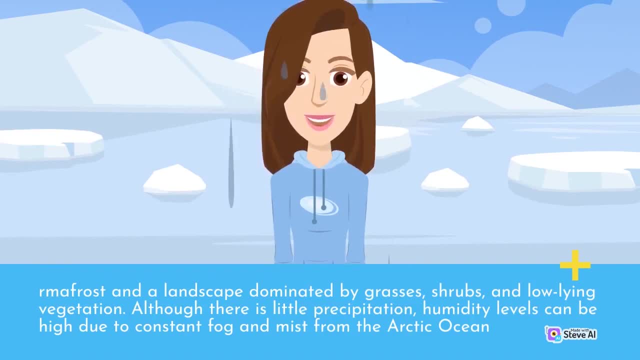 Alcapipa. the region has a wealth of history and tradition to explore. Visitors can witness the weaving techniques of the Andean people, try traditional foods such as kui, guinea pig and li Alcapipa. the region has a wealth of history and tradition to explore. 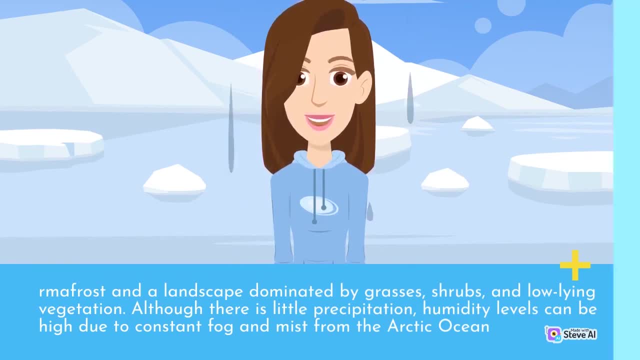 Visitors can witness the weaving techniques of the Andean people, try traditional foods such as kui guinea pig and li Alcapipa. the region has a wealth of history and tradition to explore. Visitors can witness the weaving techniques of the Andean people, try traditional foods such as kui guinea pig and li. 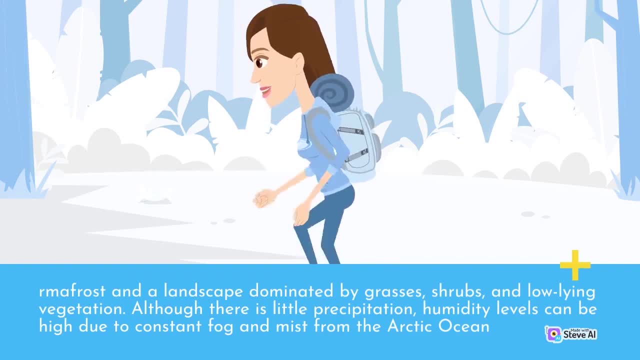 Alcapipa. the region has a wealth of history and tradition to explore. Visitors can witness the weaving techniques of the Andean people, try traditional foods such as kui, guinea pig and li Alcapipa. the region has a wealth of history and tradition to explore. 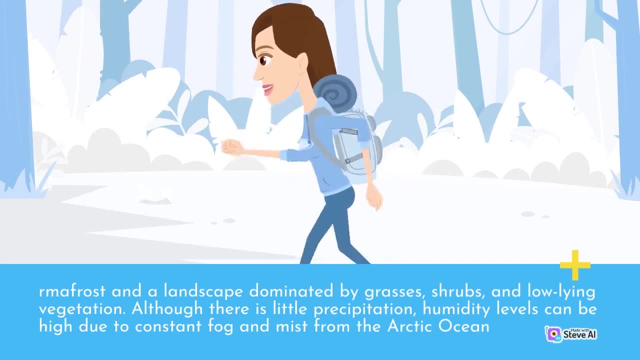 Visitors can witness the weaving techniques of the Andean people, try traditional foods such as kui guinea pig and li Alcapipa. the region has a wealth of history and tradition to explore. Visitors can witness the weaving techniques of the Andean people, try traditional foods such as kui guinea pig and li. 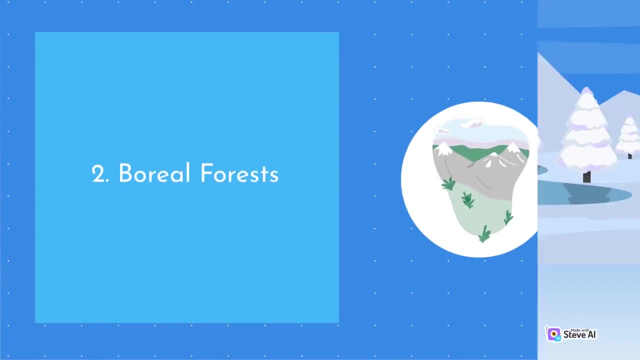 Alcapipa. the region has a wealth of history and tradition to explore. Visitors can witness the weaving techniques of the Andean people, try traditional foods such as kui, guinea pig and li Alcapipa. the region has a wealth of history and tradition to explore. 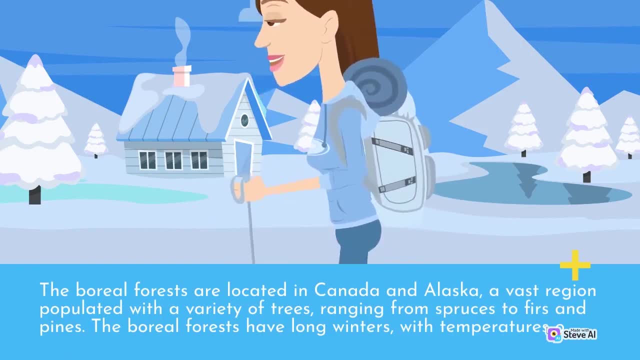 Visitors can witness the weaving techniques of the Andean people, try traditional foods such as kui guinea pig and li Alcapipa. the region has a wealth of history and tradition to explore. Visitors can witness the weaving techniques of the Andean people, try traditional foods such as kui guinea pig and li. 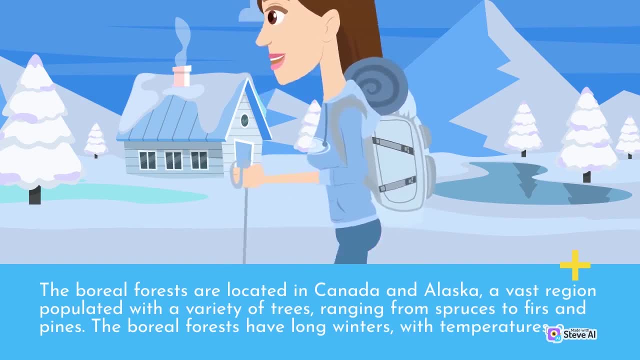 Alcapipa. the region has a wealth of history and tradition to explore. Visitors can witness the weaving techniques of the Andean people, try traditional foods such as kui, guinea pig and li Alcapipa. the region has a wealth of history and tradition to explore. 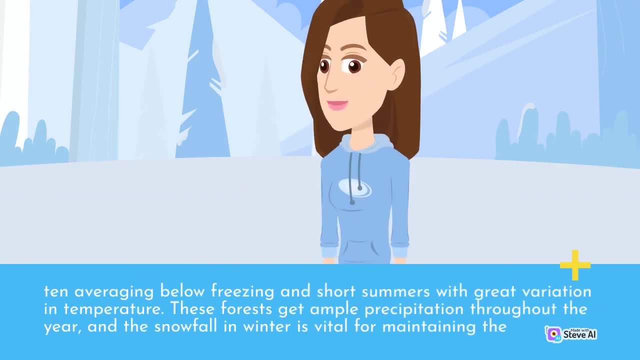 Visitors can witness the weaving techniques of the Andean people, try traditional foods such as kui guinea pig and li Alcapipa. the region has a wealth of history and tradition to explore. Visitors can witness the weaving techniques of the Andean people, try traditional foods such as kui guinea pig and li. 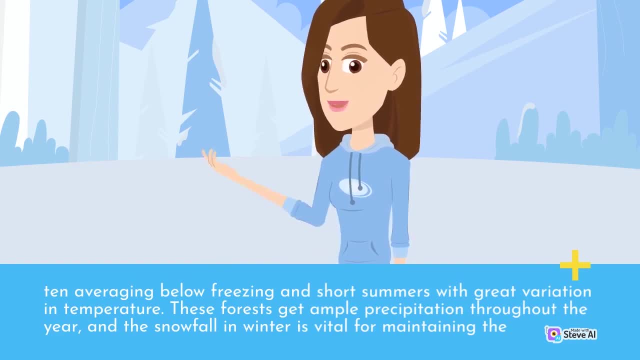 Alcapipa. the region has a wealth of history and tradition to explore. Visitors can witness the weaving techniques of the Andean people, try traditional foods such as kui, guinea pig and li Alcapipa. the region has a wealth of history and tradition to explore. 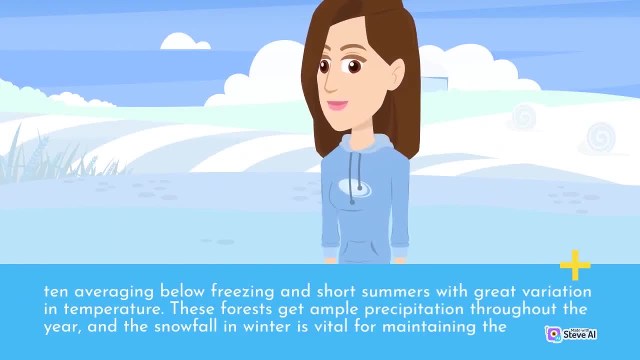 Visitors can witness the weaving techniques of the Andean people, try traditional foods such as kui guinea pig and li Alcapipa. the region has a wealth of history and tradition to explore. Visitors can witness the weaving techniques of the Andean people, try traditional foods such as kui guinea pig and li. 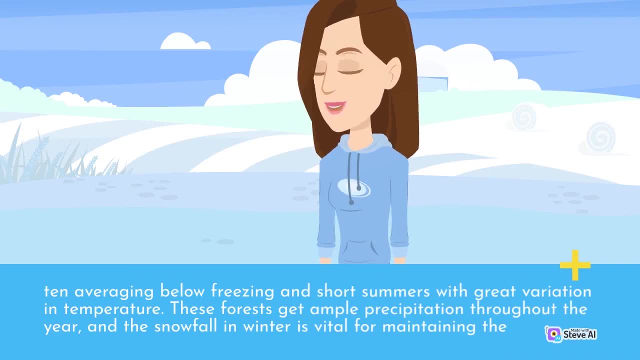 Alcapipa. the region has a wealth of history and tradition to explore. Visitors can witness the weaving techniques of the Andean people, try traditional foods such as kui, guinea pig and li Alcapipa. the region has a wealth of history and tradition to explore. 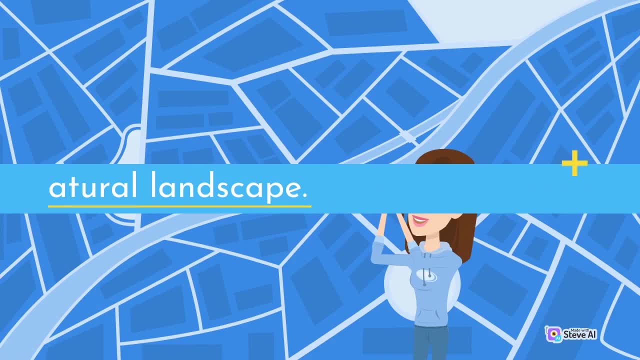 Visitors can witness the weaving techniques of the Andean people, try traditional foods such as kui guinea pig and li Alcapipa. the region has a wealth of history and tradition to explore. Visitors can witness the weaving techniques of the Andean people, try traditional foods such as kui guinea pig and li. 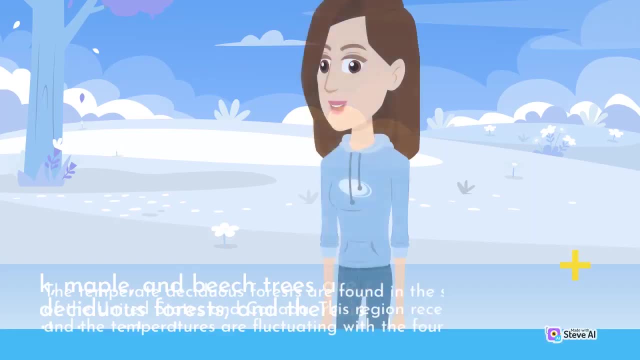 Alcapipa. the region has a wealth of history and tradition to explore. Visitors can witness the weaving techniques of the Andean people, try traditional foods such as kui, guinea pig and li Alcapipa. the region has a wealth of history and tradition to explore. 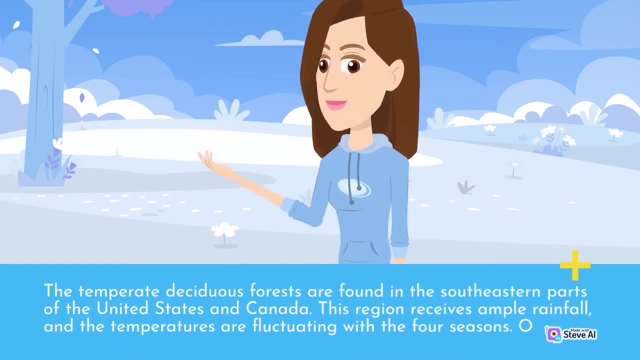 Visitors can witness the weaving techniques of the Andean people, try traditional foods such as kui guinea pig and li Alcapipa. the region has a wealth of history and tradition to explore. Visitors can witness the weaving techniques of the Andean people, try traditional foods such as kui guinea pig and li. 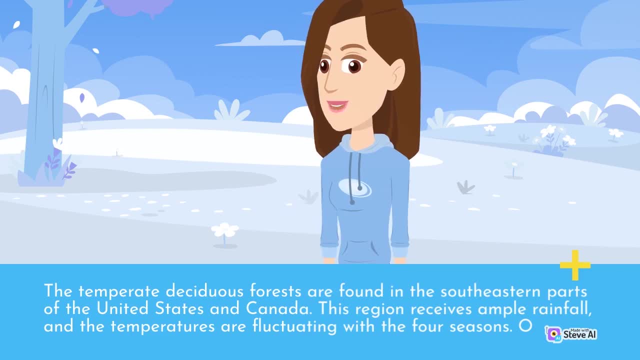 Alcapipa. the region has a wealth of history and tradition to explore. Visitors can witness the weaving techniques of the Andean people, try traditional foods such as kui, guinea pig and li Alcapipa. the region has a wealth of history and tradition to explore. 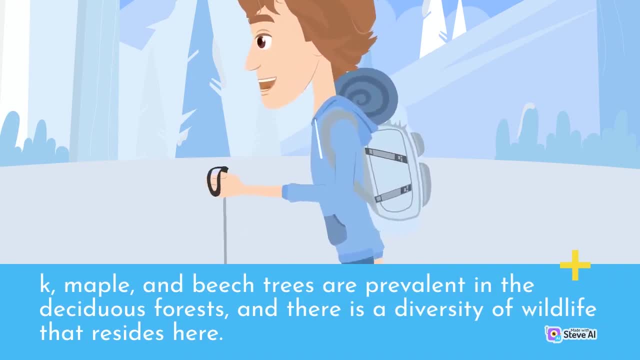 Visitors can witness the weaving techniques of the Andean people, try traditional foods such as kui guinea pig and li Alcapipa. the region has a wealth of history and tradition to explore. Visitors can witness the weaving techniques of the Andean people, try traditional foods such as kui guinea pig and li. 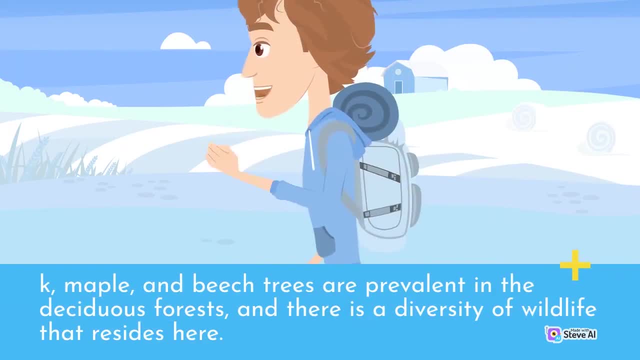 Alcapipa. the region has a wealth of history and tradition to explore. Visitors can witness the weaving techniques of the Andean people, try traditional foods such as kui, guinea pig and li Alcapipa. the region has a wealth of history and tradition to explore. 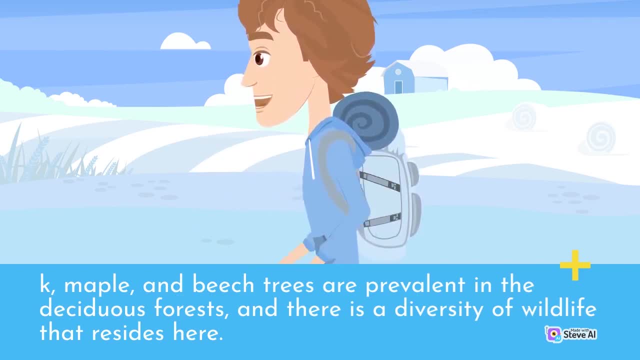 Visitors can witness the weaving techniques of the Andean people, try traditional foods such as kui guinea pig and li Alcapipa. the region has a wealth of history and tradition to explore. Visitors can witness the weaving techniques of the Andean people, try traditional foods such as kui guinea pig and li. 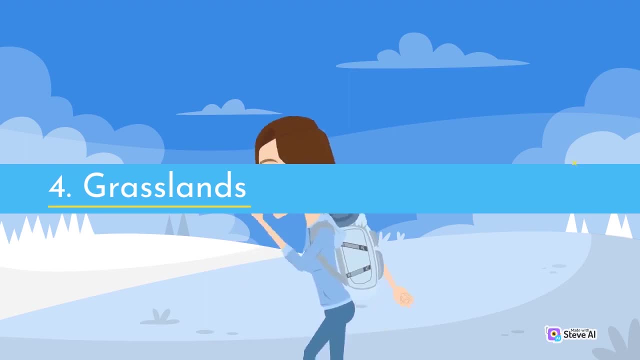 Alcapipa. the region has a wealth of history and tradition to explore. Visitors can witness the weaving techniques of the Andean people, try traditional foods such as kui, guinea pig and li Alcapipa. the region has a wealth of history and tradition to explore. 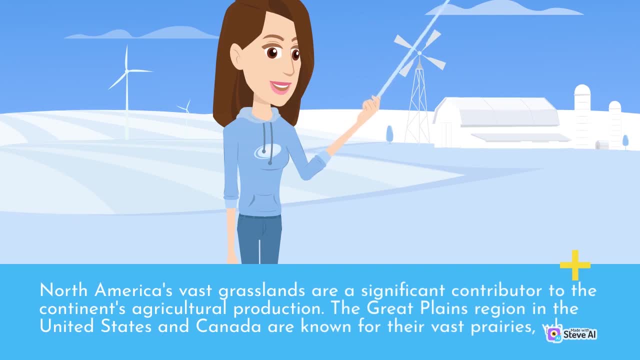 Visitors can witness the weaving techniques of the Andean people, try traditional foods such as kui guinea pig and li Alcapipa. the region has a wealth of history and tradition to explore. Visitors can witness the weaving techniques of the Andean people, try traditional foods such as kui guinea pig and li. 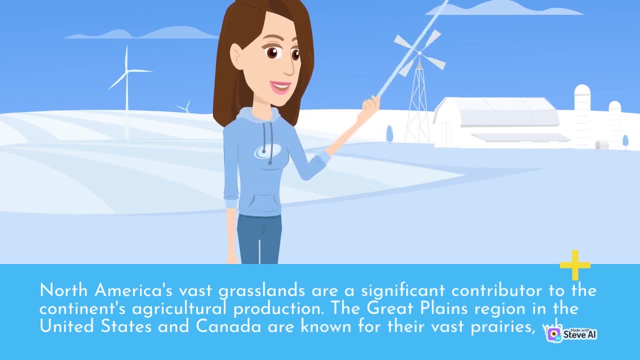 Alcapipa. the region has a wealth of history and tradition to explore. Visitors can witness the weaving techniques of the Andean people, try traditional foods such as kui, guinea pig and li Alcapipa. the region has a wealth of history and tradition to explore. 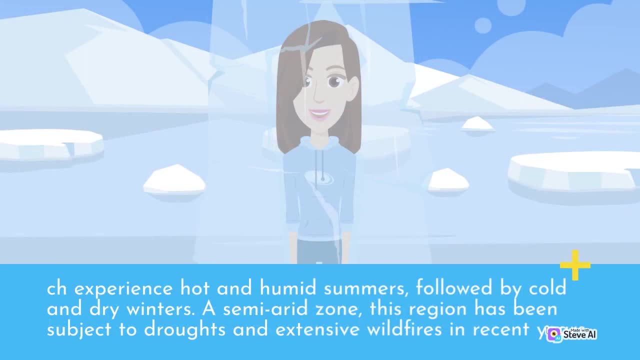 Visitors can witness the weaving techniques of the Andean people, try traditional foods such as kui guinea pig and li Alcapipa. the region has a wealth of history and tradition to explore. Visitors can witness the weaving techniques of the Andean people, try traditional foods such as kui guinea pig and li. 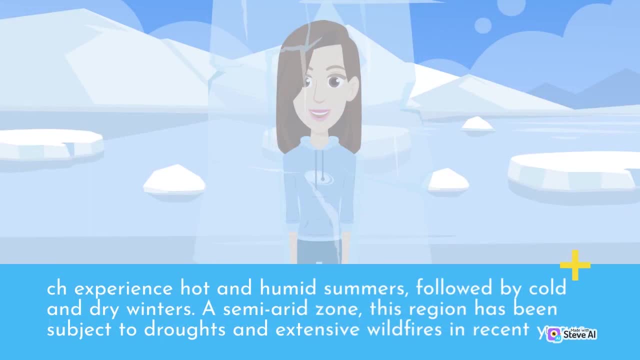 Alcapipa. the region has a wealth of history and tradition to explore droughts and extensive wildfires in recent years. See each experience hot and humid summers followed by cold and dry winters. A semi-arid zone, this region has been subject to droughts and extensive wildfires in recent. 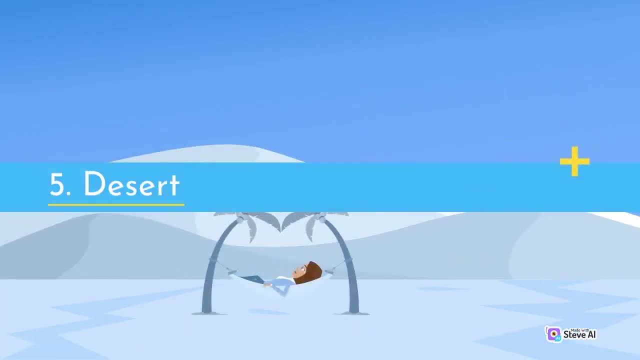 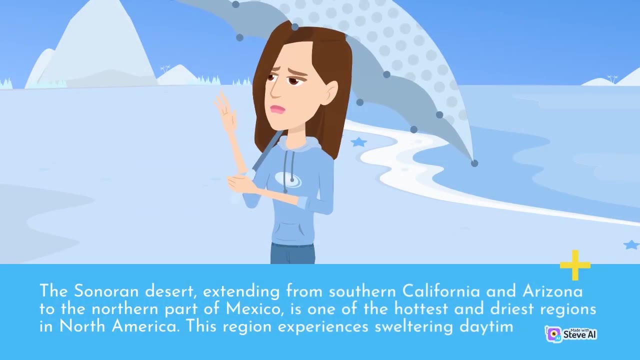 years. 5. Desert: The Sonoran Desert, extending from southern California and Arizona to the northern part of Mexico, is one of the hottest and driest regions in North America. This region experiences sweltering daytime temperatures which can reach above 100 degrees. 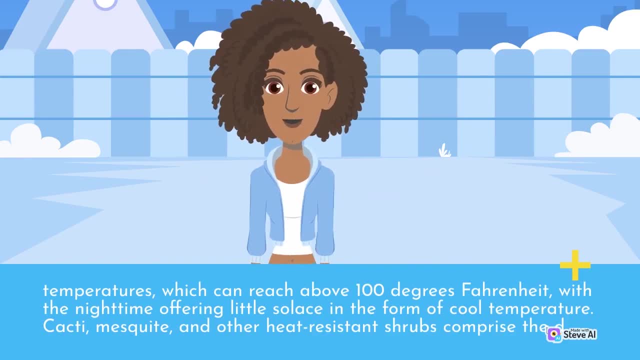 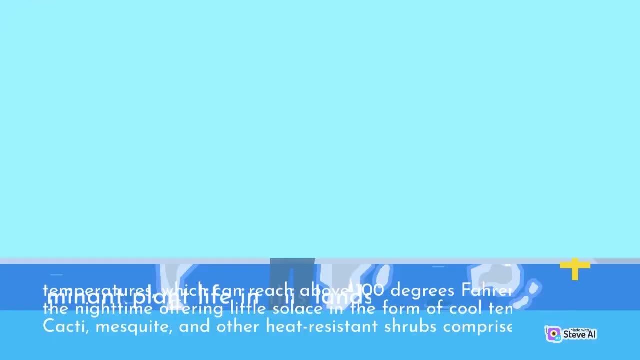 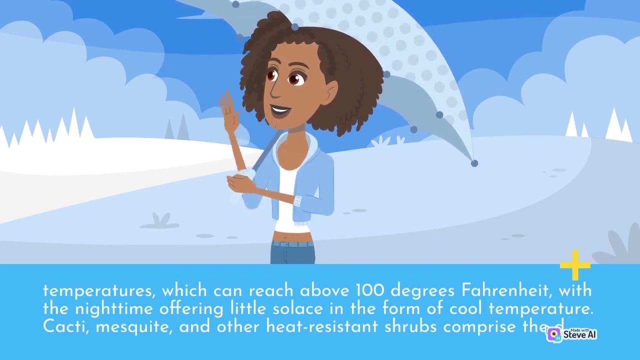 Fahrenheit, with a nighttime offering little solace in the form of cool temperature. Cacti, mesquite and other heat-resistant shrubs comprise the D Temperatures, which can reach above 100 degrees Fahrenheit, with a nighttime offering little solace in the form of cool temperature. 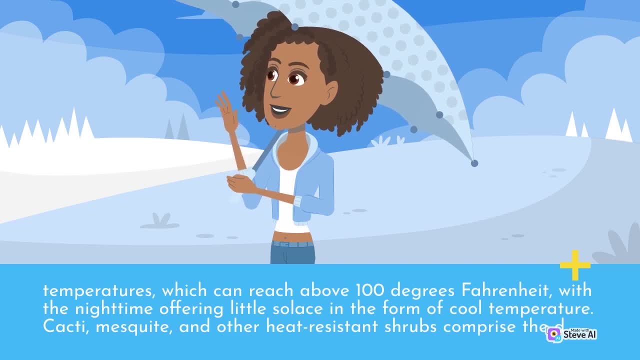 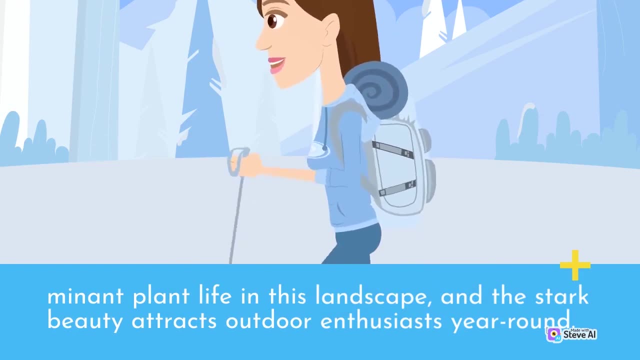 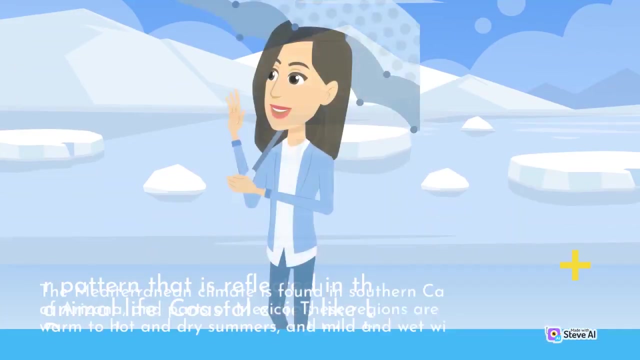 Cacti, mesquite and other heat-resistant shrubs comprise the D Men implant life in this landscape and this dark beauty attracts outdoor enthusiasts year-round. 6. Mediterranean: The Mediterranean climate is found in southern California, some parts of Arizona and parts. 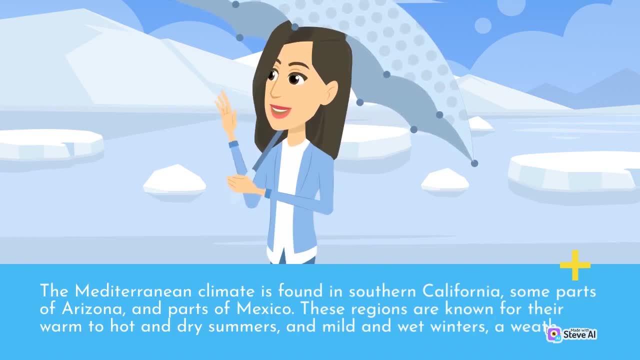 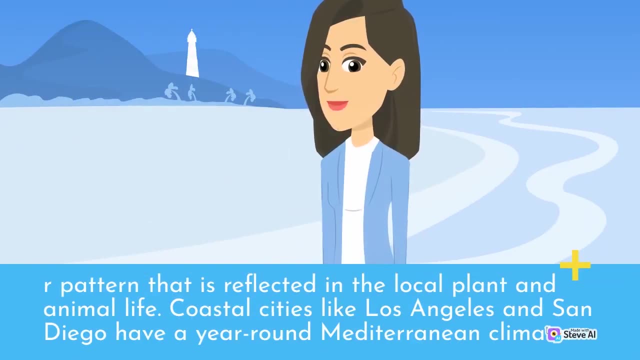 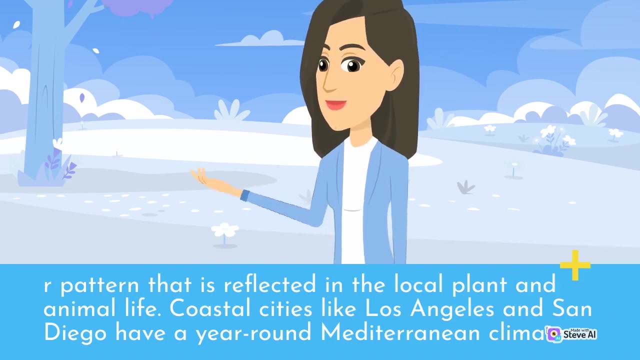 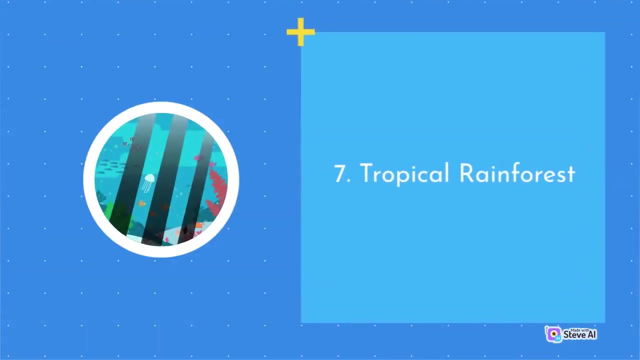 of Mexico. These regions are known for their warm to hot and dry summers and mild and wet winters, And the weather, with the pushing waves of trees, creates a pleasantlements for cool and fresh weather. 7. Tropical Rainforest Located primarily in Mexico and Central America. atheists are fishers who have been actively. 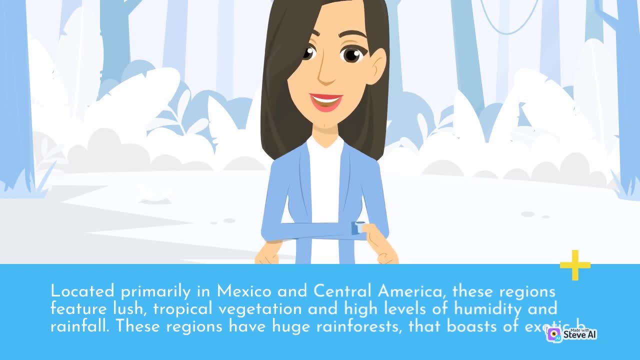 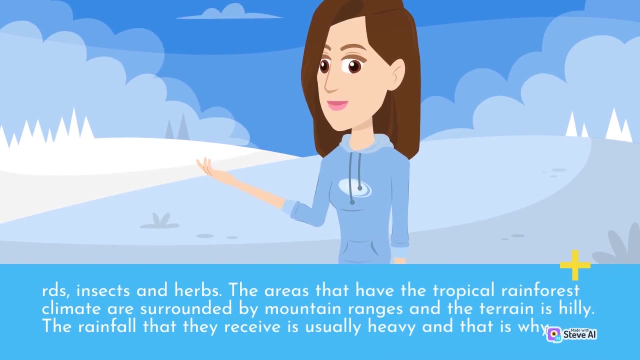 attracted to the cath生活. These regions feature lush tropical vegetation and high levels of humidity and rainfall. These regions have huge rainforests that boast of exotic bee, RDS, Insects and Herbs. The areas that have the tropical rainforest climate are surrounded by mountain ranges and the terrain is hilly. The rainfall that they receive is usually heavy, and that is why RDS Insects and Herbs. The areas that have the tropical rainforest climate are surrounded by mountain ranges and the terrain is hilly. The rainfall that they receive is usually 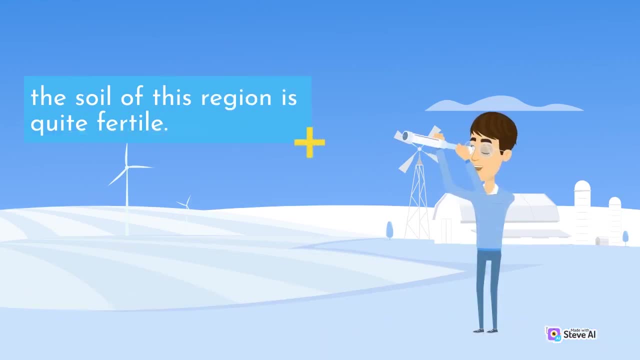 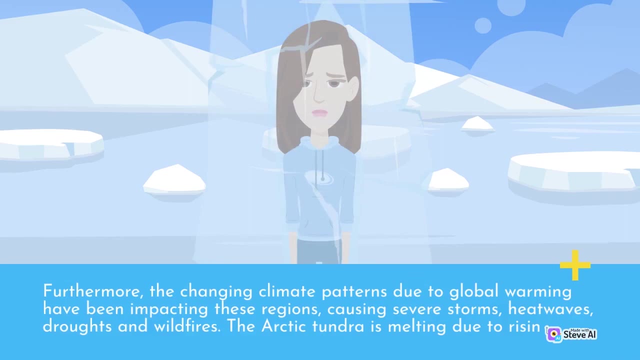 heavy, and that is why The soil of this region is quite fertile. Furthermore, the changing climate patterns due to global warming have been impacting these regions, causing severe storms, heat waves, droughts and wildfires. The Arctic tundra is melting due to 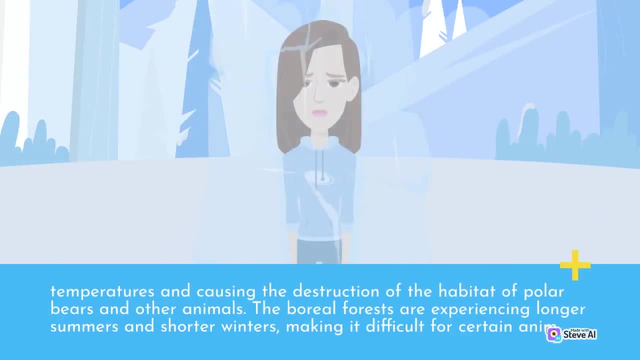 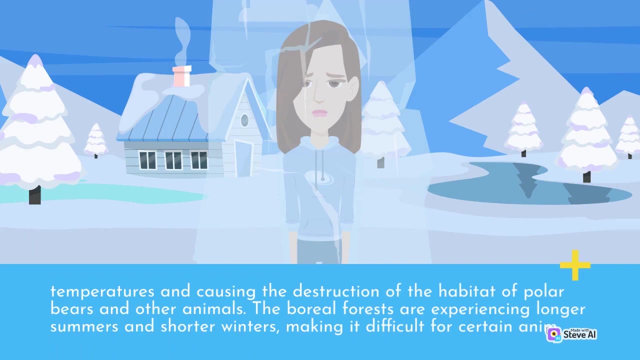 rising temperatures and causing the destruction of the habitat of polar bears and other animals. The boreal forests are experiencing longer summers and shorter winters, making it difficult for certain aneem Temperatures and causing the destruction of the habitat of polar bears and other animals. The boreal forests are experiencing longer summers and shorter winters. 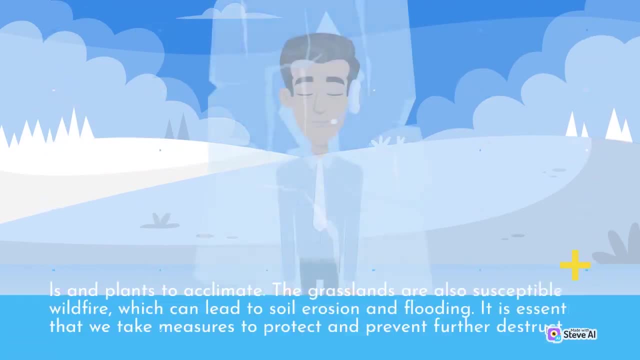 making it difficult for certain aneem LS and Plants to Acclimate. The grasslands are also susceptible to wildfire, which can lead to soil erosion and flooding. It is essential, however, that we take measures to protect and prevent further destruct. 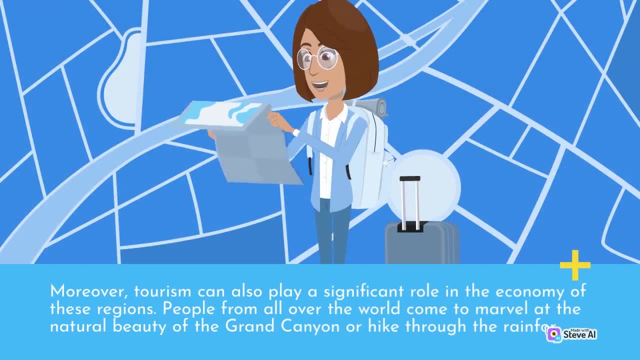 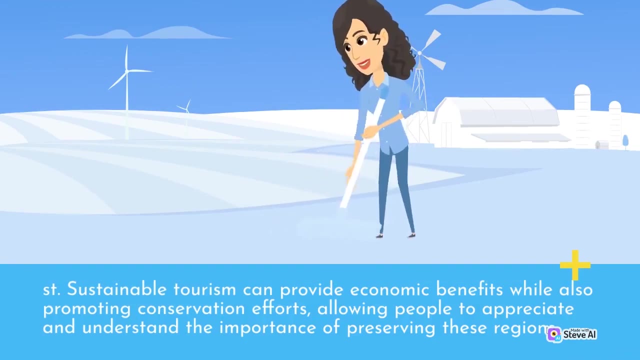 Moreover, tourism can also play a significant role in the economy of these regions. People from all over the world come to marvel at the natural beauty of the Grand Canyon or hike through the rainforest Street. sustainable tourism can provide economic benefits while also promoting conservation efforts. 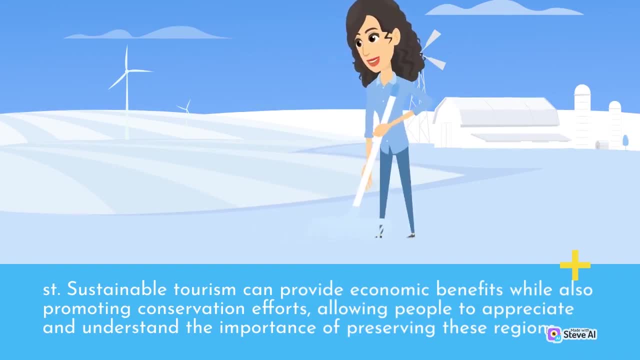 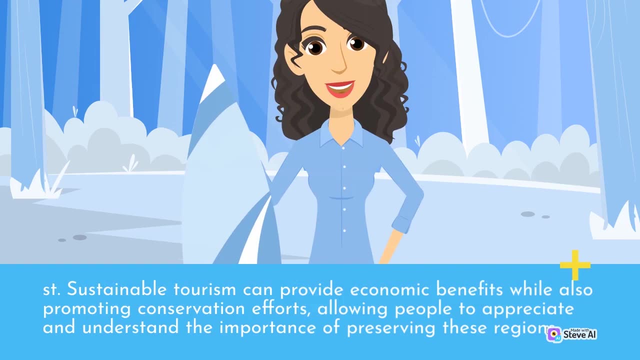 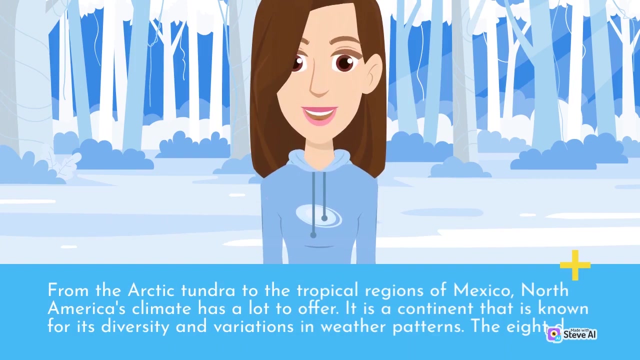 allowing people to appreciate and understand the importance of preserving these regions. Street sustainable tourism can provide economic benefits while also promoting conservation efforts, allowing people to appreciate and understand the importance of preserving these regions. From the Arctic tundra to the tropical regions of Mexico, North America's climate has a lot to 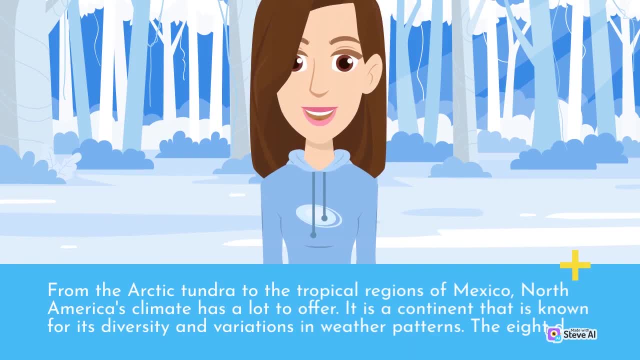 offer. It is a continent that is known for its diversity in variations in weather patterns. The 8D FL. 1500. 500. 150. 150. 100. 300. 200. 100. 1500.. 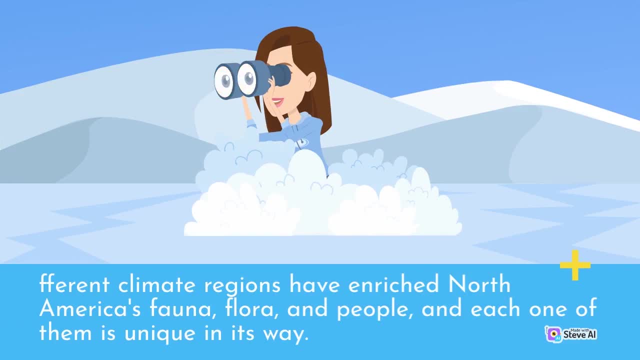 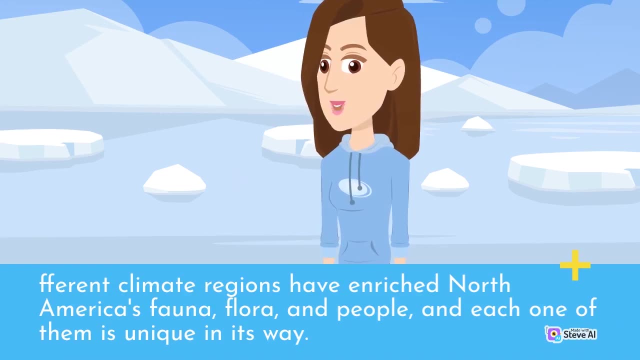 200.. 400.. enriched North America's fauna, flora and people, and each one of them is unique in its way. Current climate regions have enriched North America's fauna, flora and people, and each one of them is unique in its way. 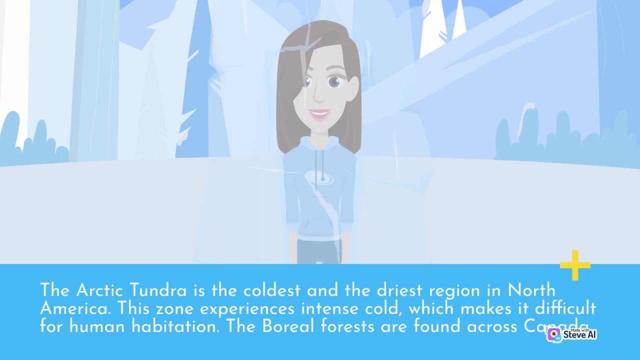 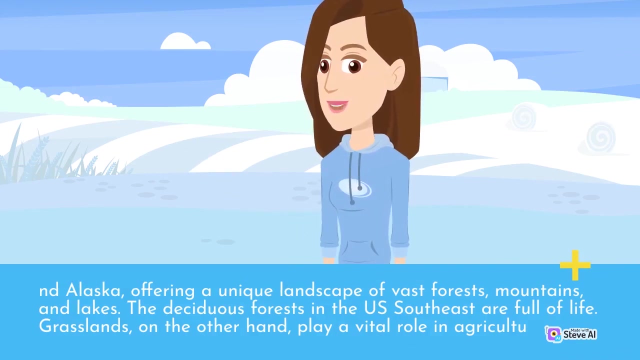 The Arctic tundra is the coldest and the driest region in North America. This zone experiences intense cold which makes it difficult for human habitation. The boreal forests are found across Canada, ND, Alaska, offering a unique landscape of vast forests, mountains and lakes. 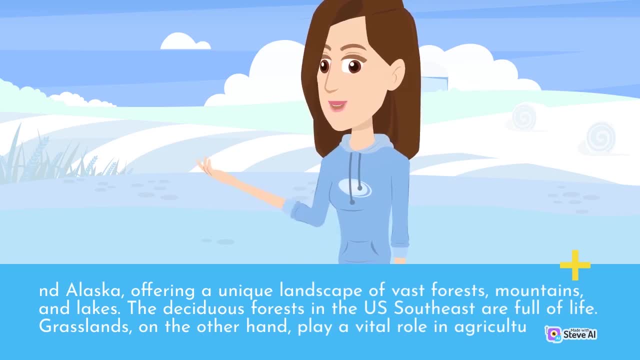 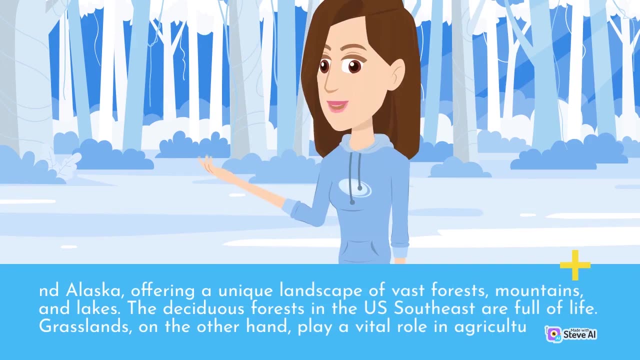 The deciduous forests in the US Southeast are full of life. Grasslands, on the other hand, play a vital role in agriculture. ND Alaska, offering a unique landscape of vast forests, mountains and lakes. The deciduous forests in the US Southeast are full of life. 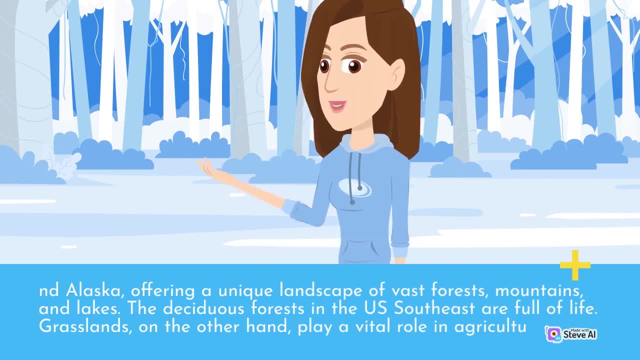 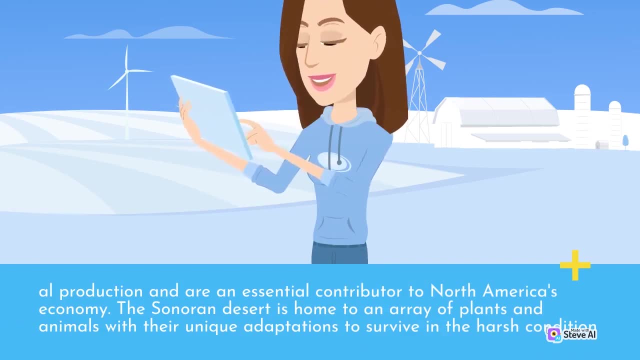 Grasslands, on the other hand, play a vital role in agriculture. Kiwo Pigeons, on the other hand, play a vital role in agriculture, Owl production and are an essential contributor to North America's economy. The Sonoran Desert is home to an array of plants and animals with their unique adaptations to survive in the harsh condition. 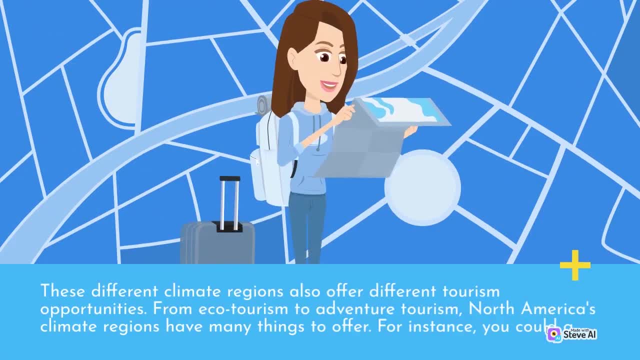 These different climate regions also offer different tourism opportunities, From ecotourism to adventure tourism. North America's climate regions have many things to offer, For instance, Yukuji. On the other hand, Zipun overview field located in Caracas, beings of a sensitive Torres的 F counselor. 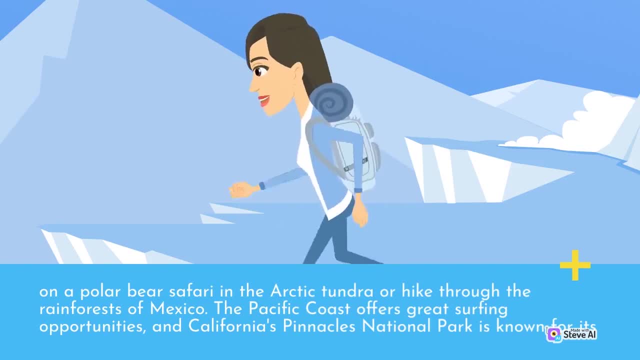 a polar bear safari in the Arctic tundra or hike through the rainforests of Mexico. The Pacific coast offers great surfing opportunities and California's Pinnacles National Park is known for its. On a polar bear safari in the Arctic tundra or hike through the. 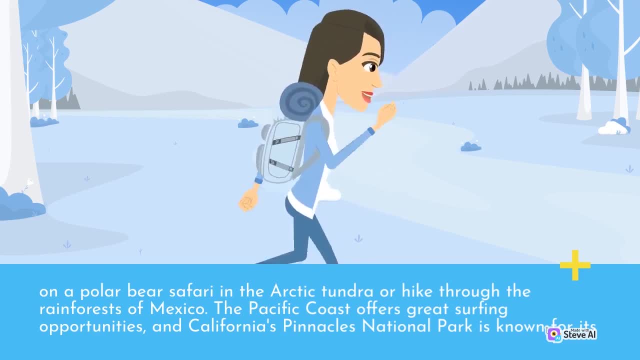 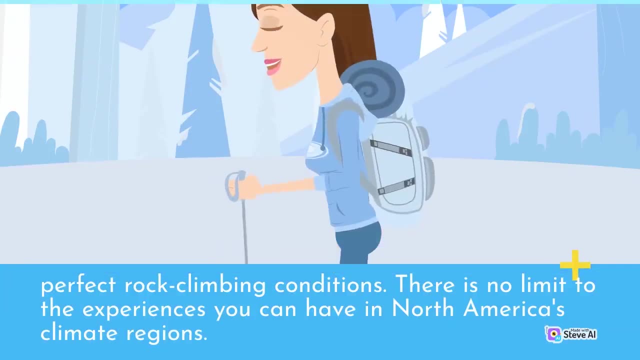 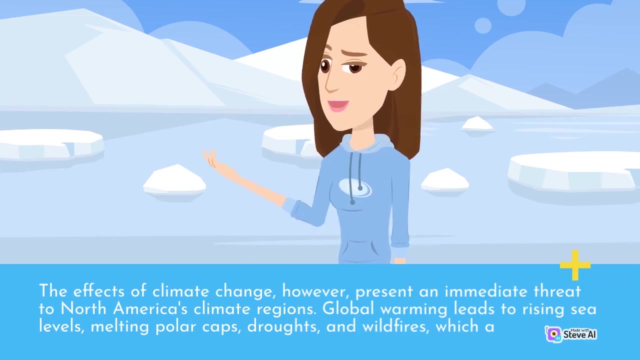 rainforests of Mexico. The Pacific coast offers great surfing opportunities, and California's Pinnacles National Park is known for its Perfect rock climbing conditions. There is no limit to the experiences you can have in North America's climate regions. The effects of climate change, however, present an immediate threat to North America's climate. 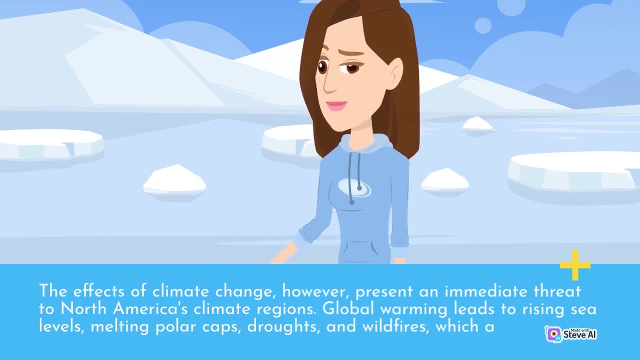 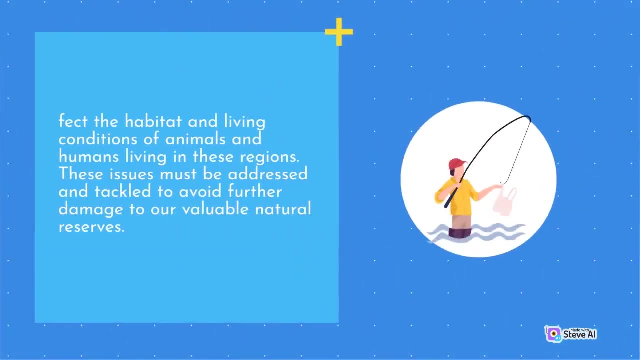 regions. Global warming leads to rising sea levels, melting polar caps, droughts and wildfires, which a FECT the habitat and living conditions of animals and humans living in these regions. These issues must be addressed and tackled to avoid further damage to our 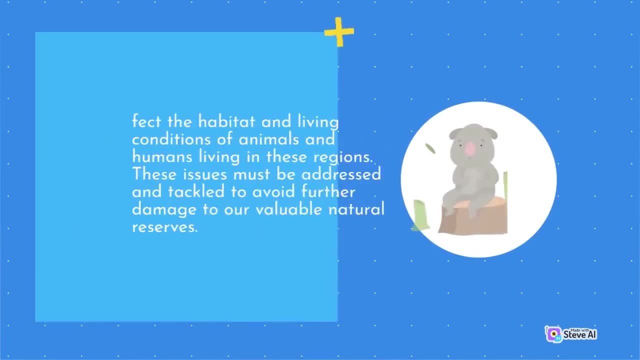 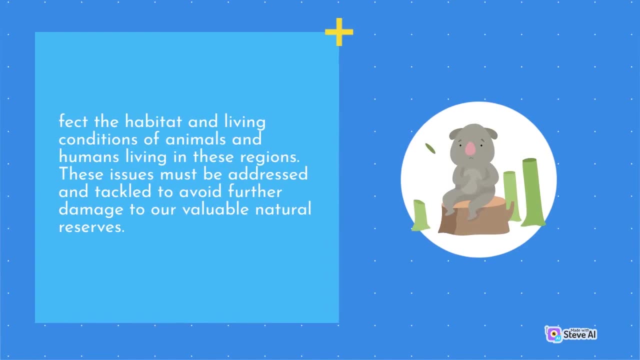 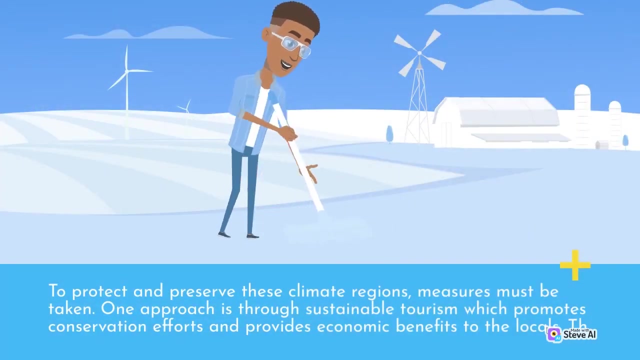 values and the environment VECT the habitat and living conditions of animals and humans living in these regions. These issues must be addressed and tackled to avoid further damage to our valuable natural reserves. To protect and preserve these climate regions, measures must be taken. 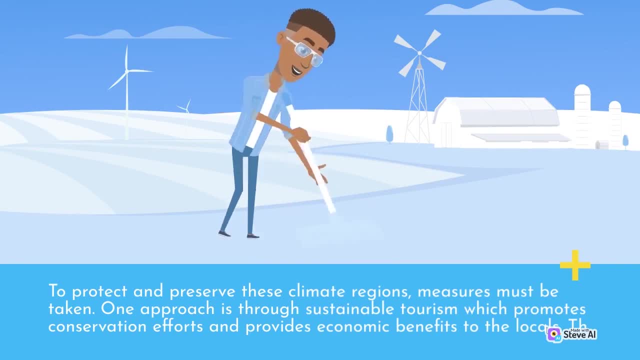 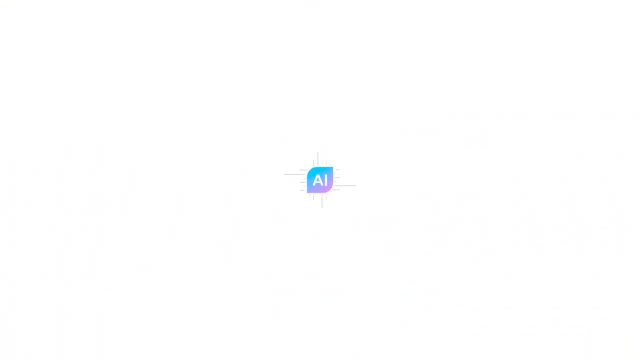 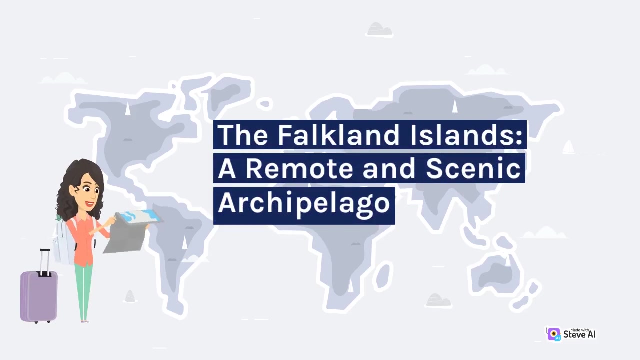 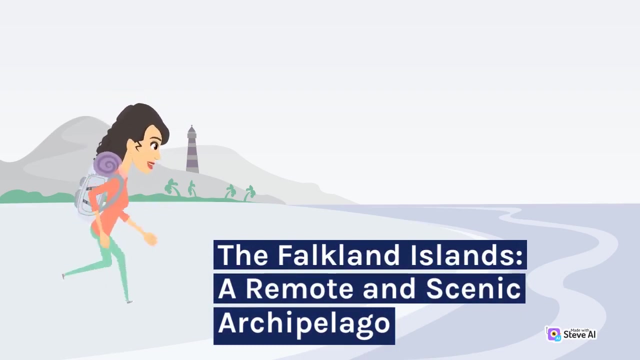 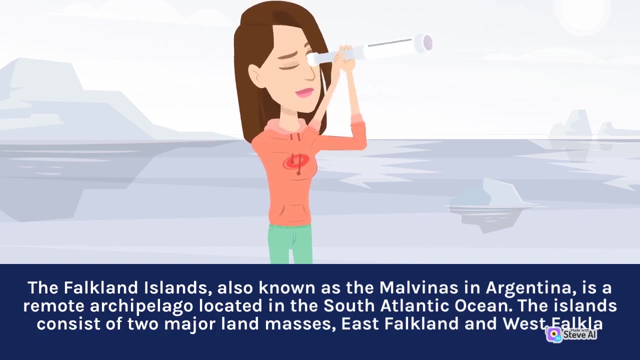 One approach is through sustainable tourism, which promotes conservation efforts and provides economic benefits to the locals. TH: The Falkland Islands: a remote and scenic archipelago. The Falkland Islands, a remote and scenic archipelago. The Falkland Islands, also known as the Malvinas in Argentina, is a remote archipelago located in the South Atlantic Ocean. 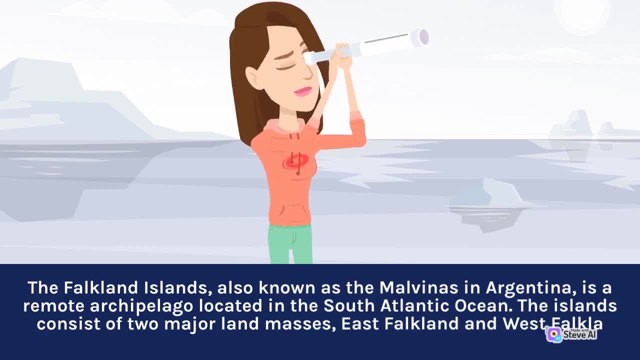 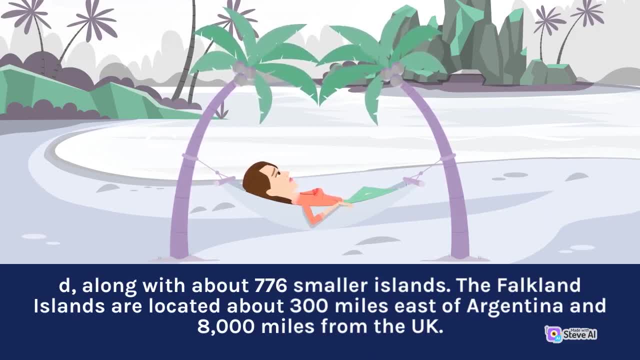 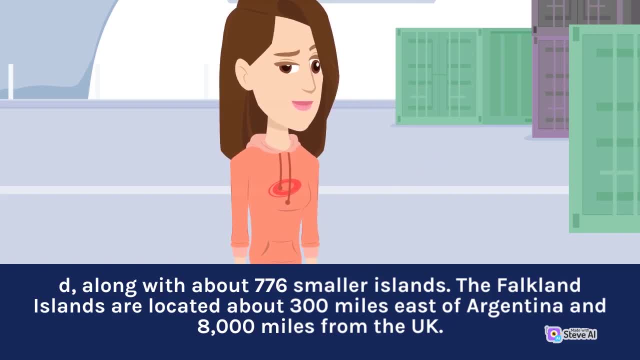 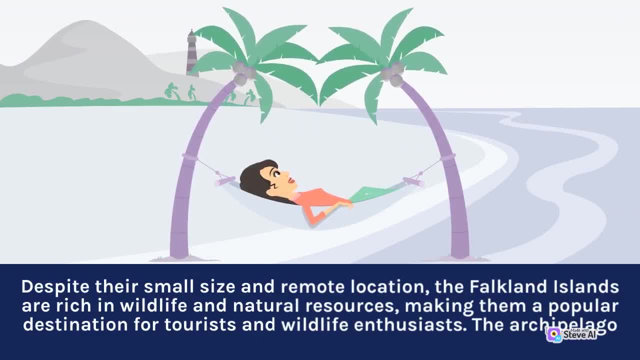 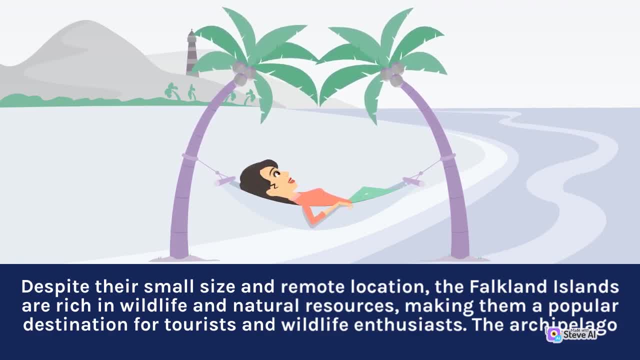 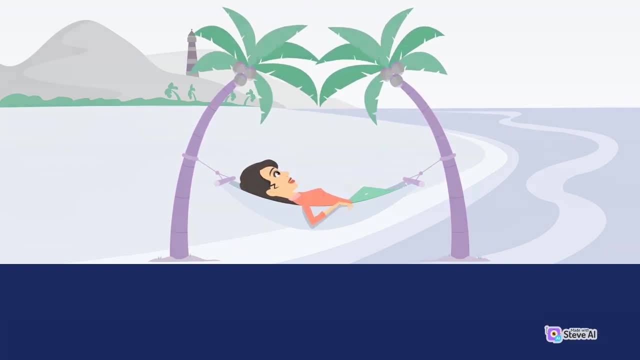 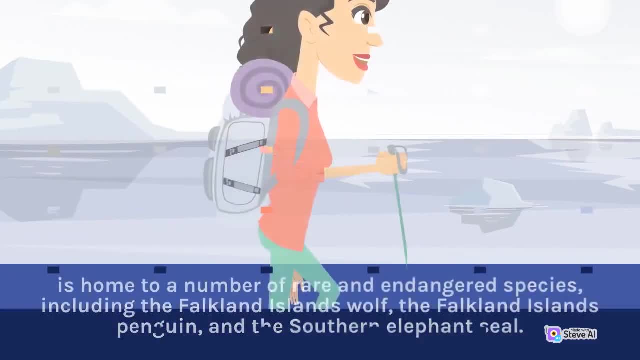 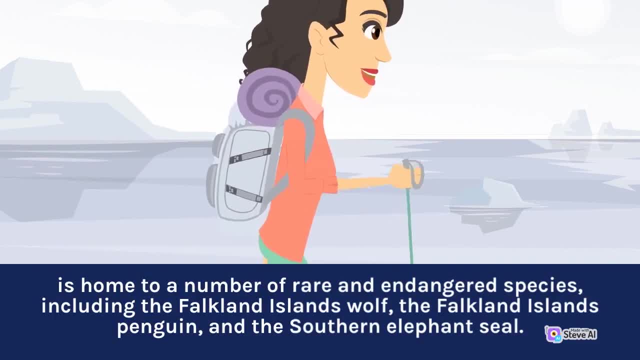 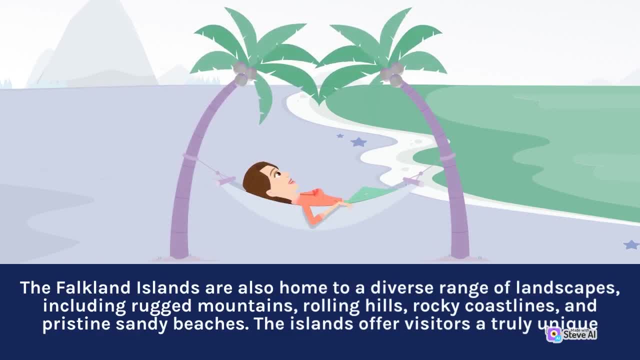 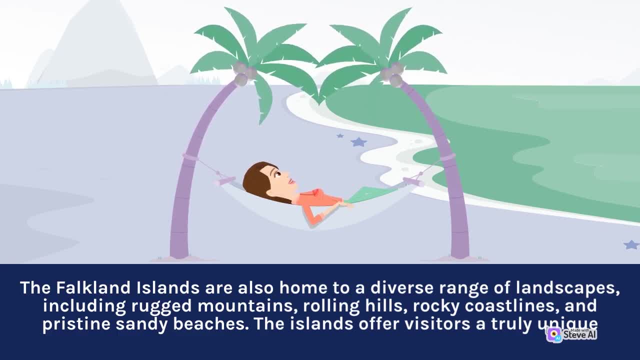 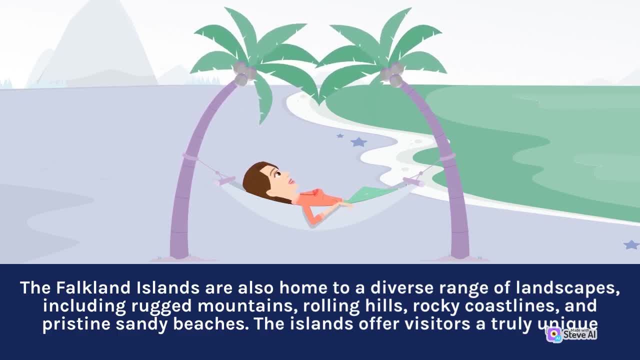 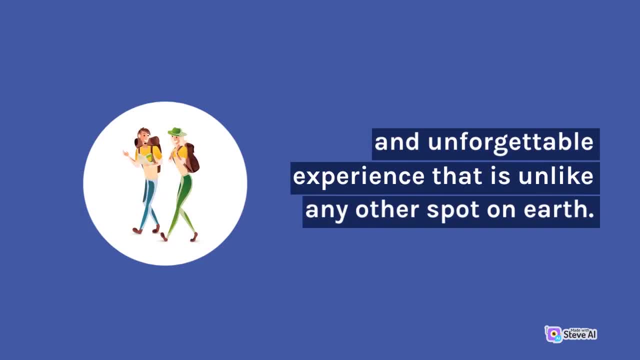 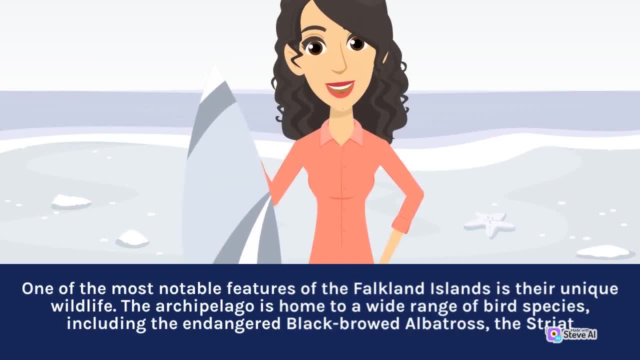 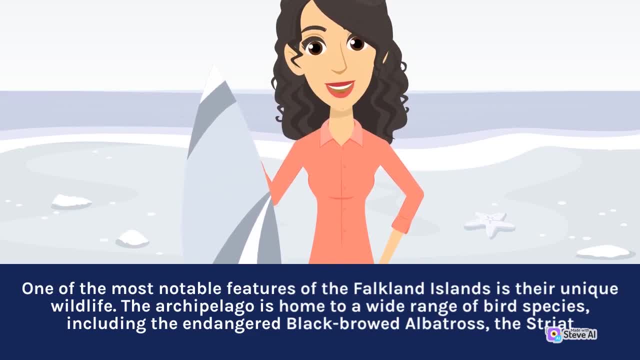 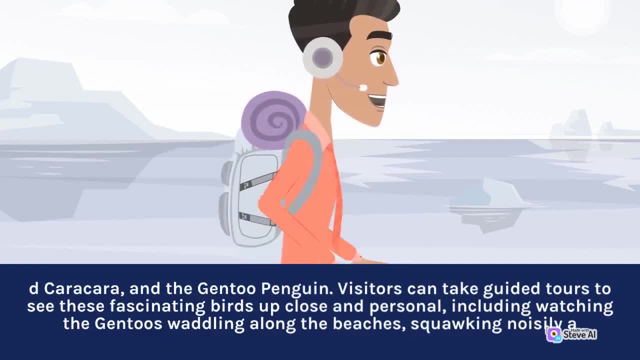 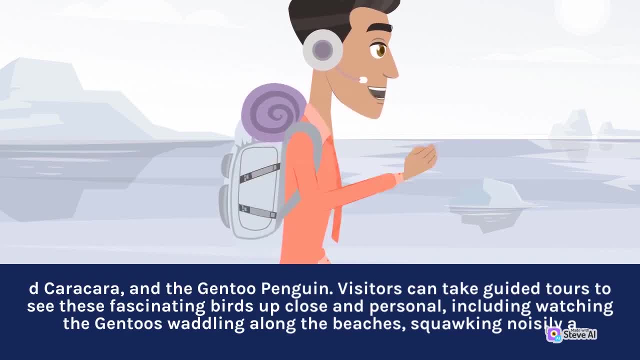 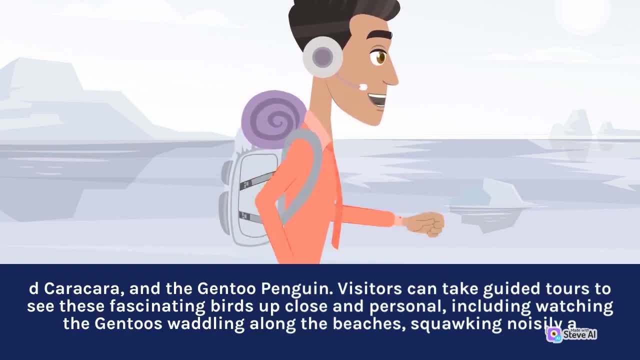 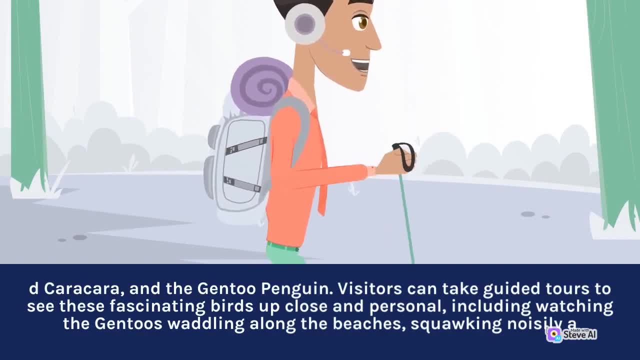 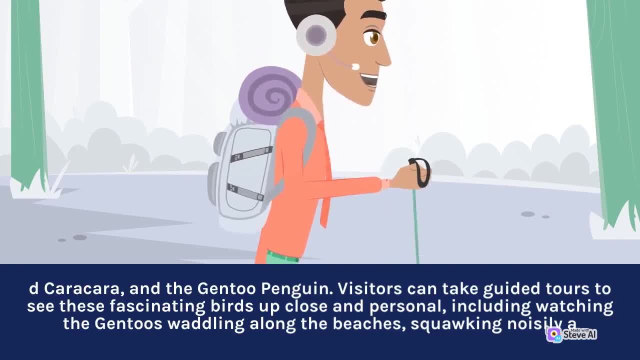 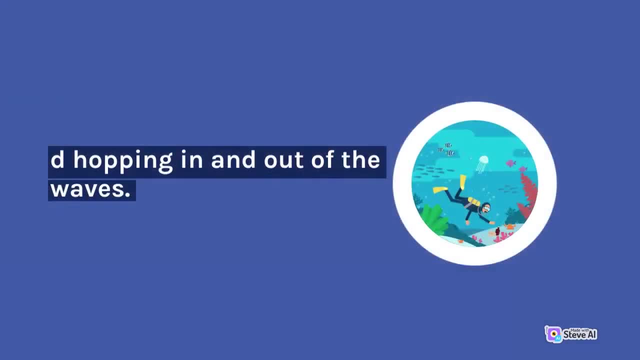 The islands consist of two major landmasses: East Falkland and West Falkland. The islands consist of two major landmasses: East Falkland and West Falkland. The islands are also home to a number of marine mammals. The islands are also home to a number of marine mammals. 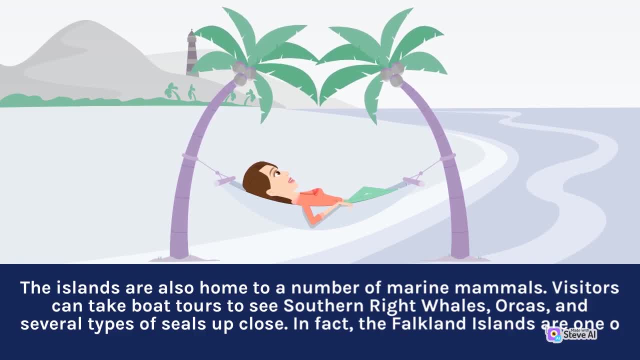 Visitors can take boat tours to see southern right whales, orcas and several types of seals up close. Visitors can take boat tours to see southern right whales, orcas and several types of seals up close. Visitors can take boat tours to see southern right whales, orcas and several types of seals up close. 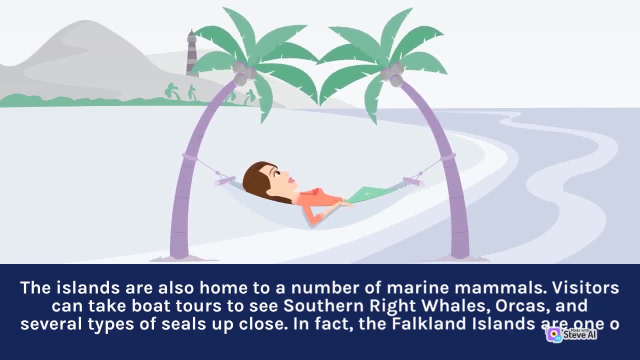 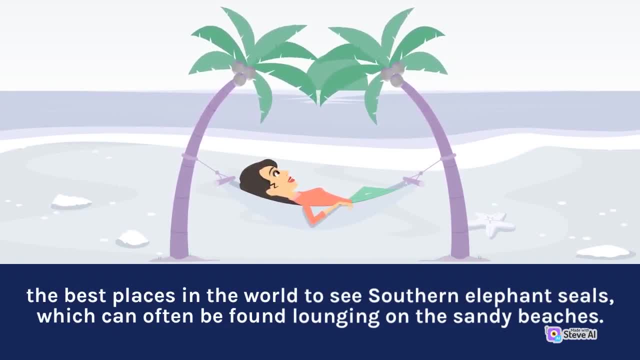 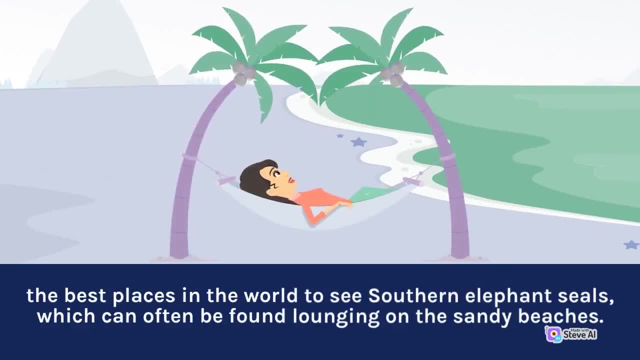 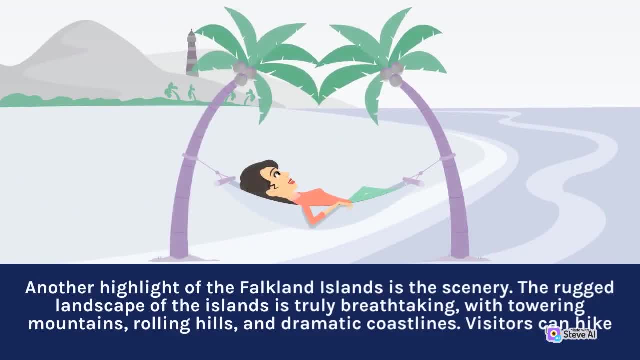 The best places in the world to see southern elephant seals, which can often be found lounging on the sandy beaches. Another highlight of the Falkland Islands is the scenery. Another highlight of the Falkland Islands is the scenery. The rugged landscape of the islands is truly breathtaking, with towering mountains, rolling hills and dramatic coastlines. 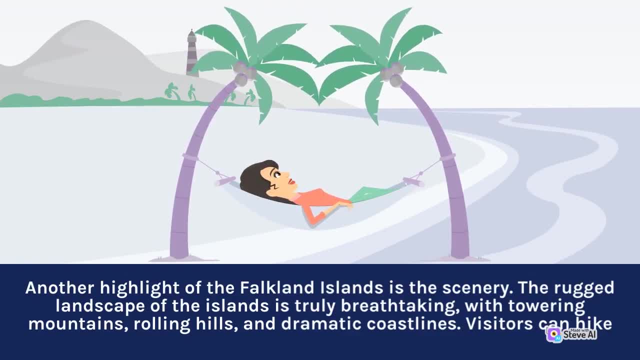 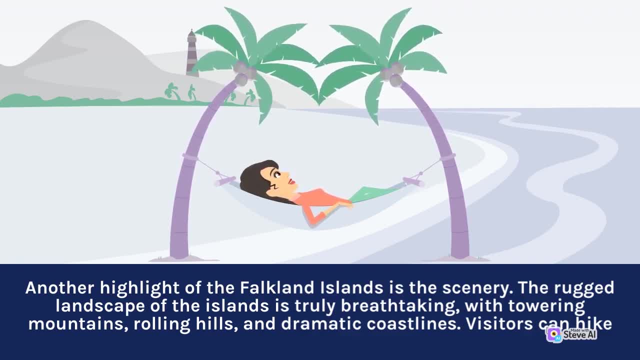 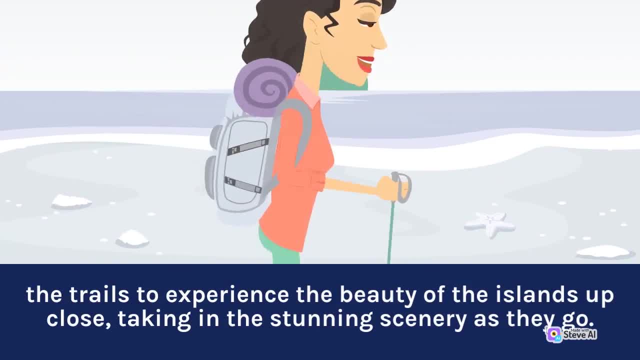 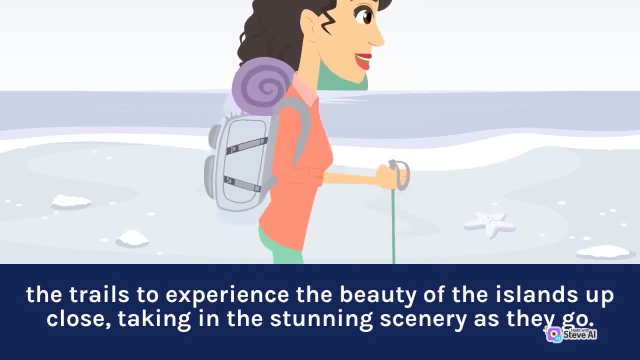 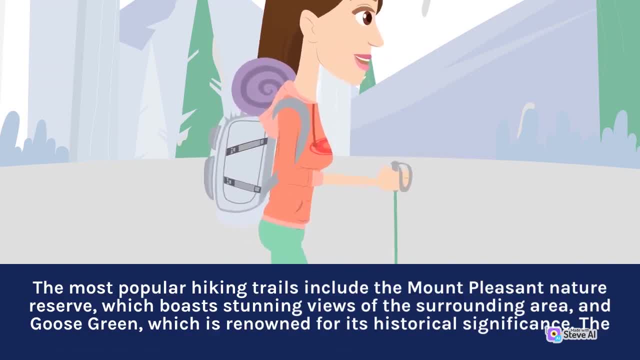 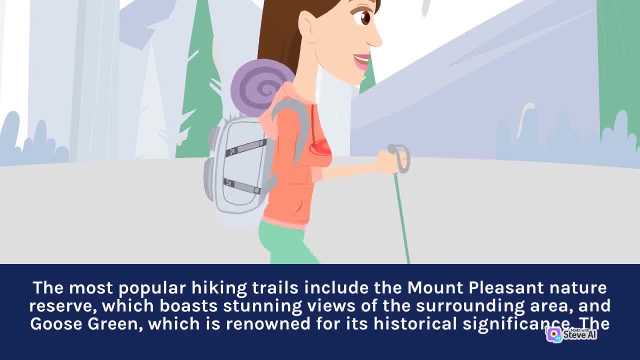 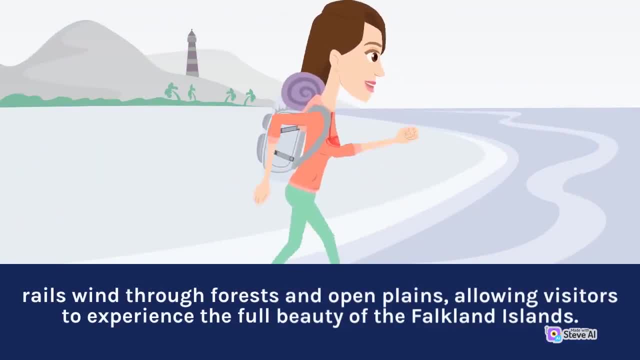 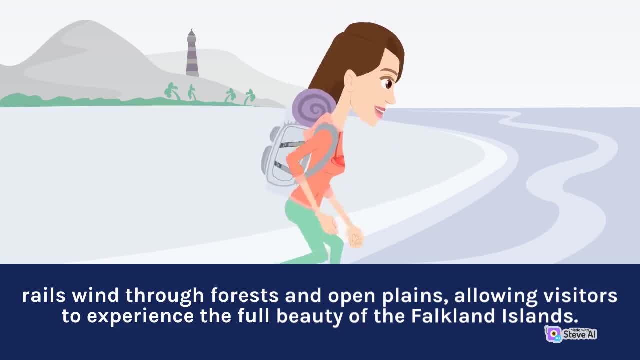 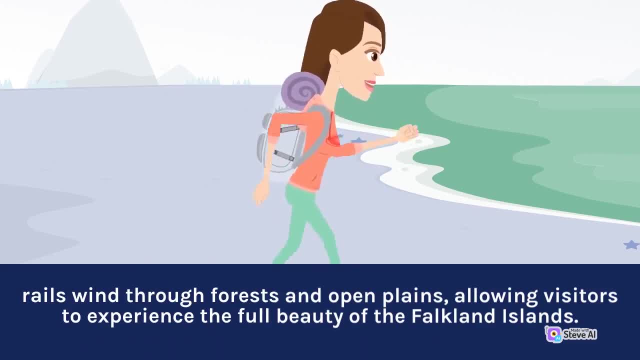 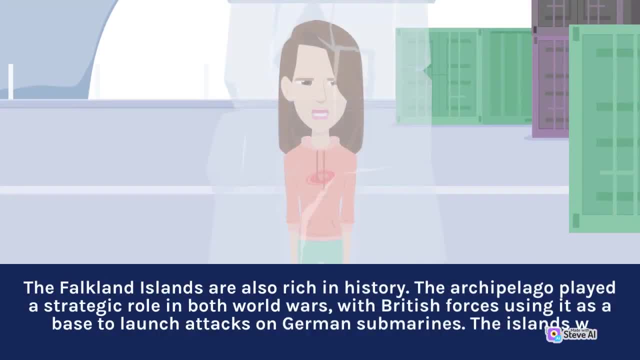 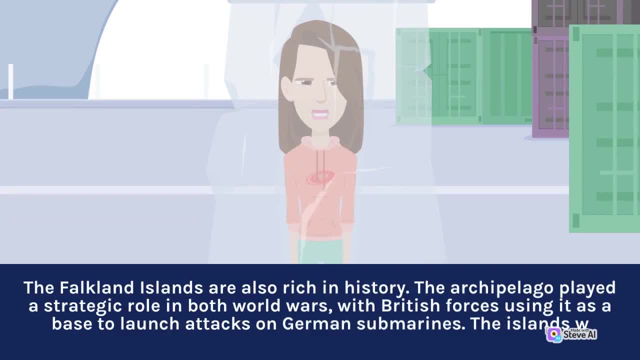 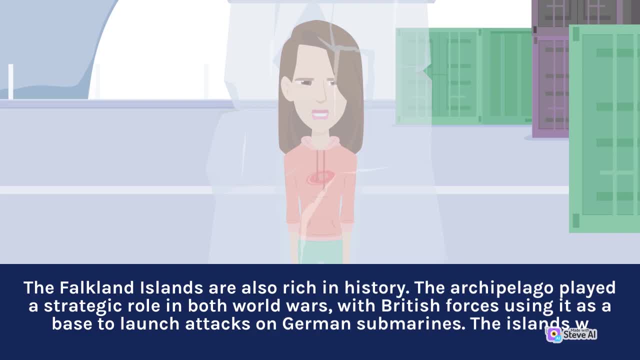 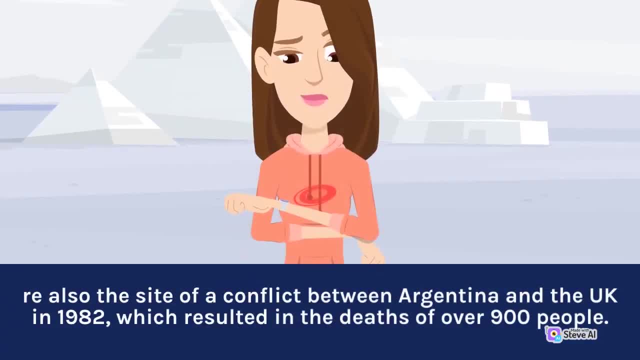 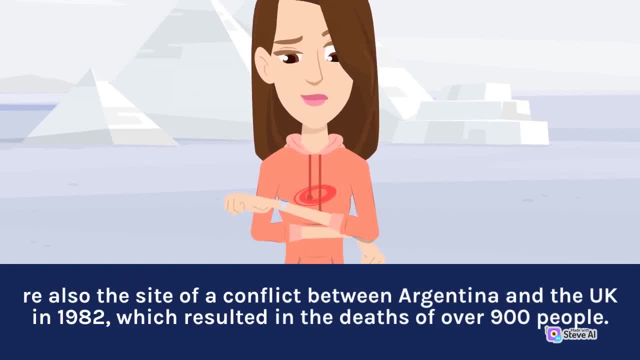 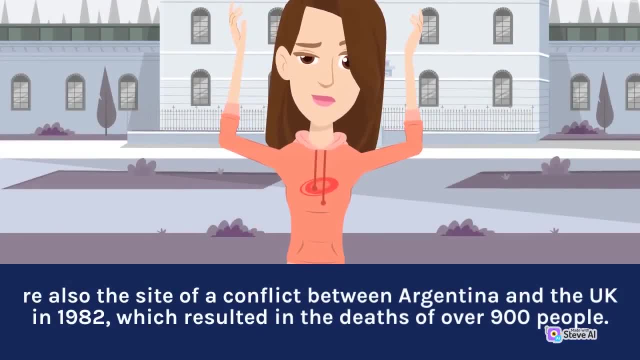 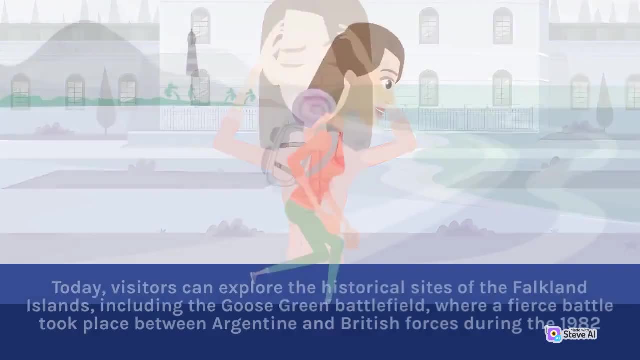 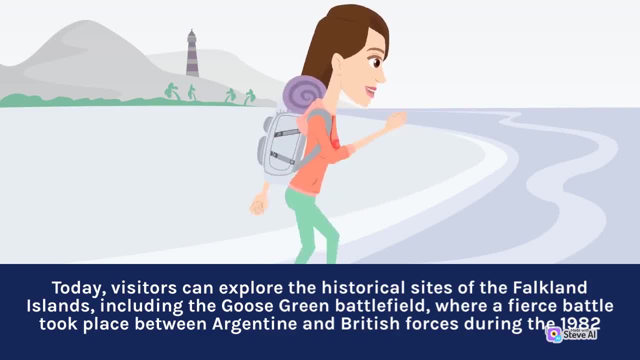 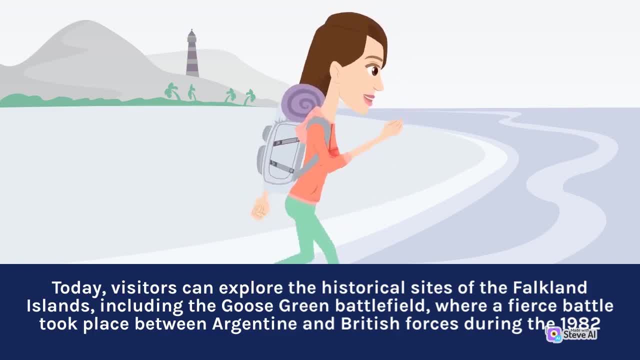 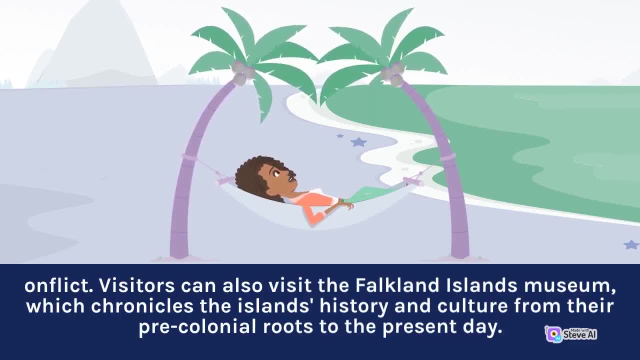 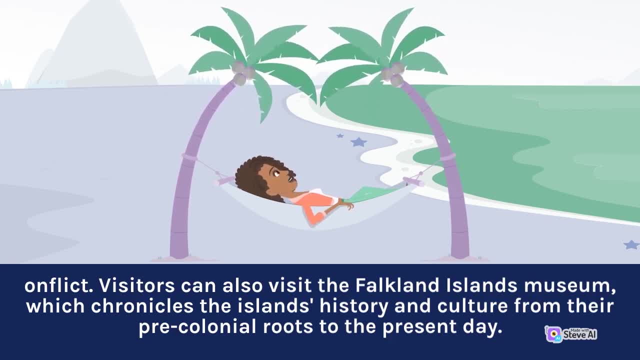 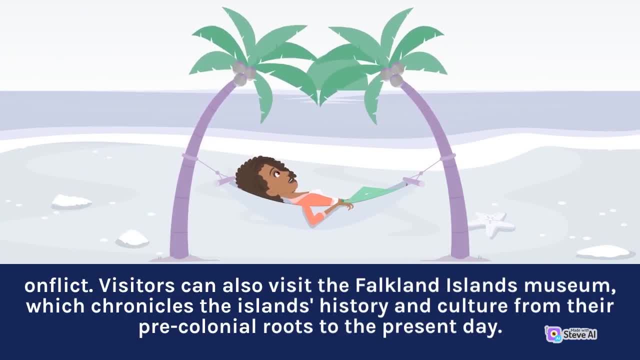 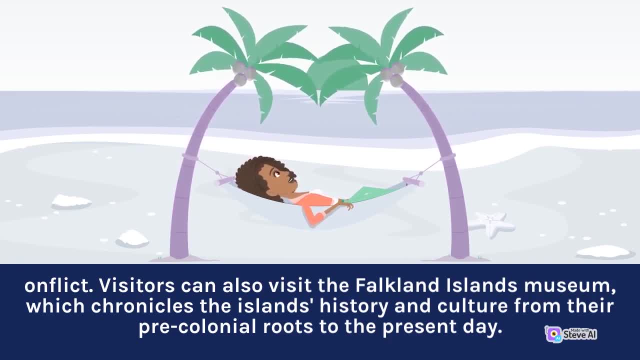 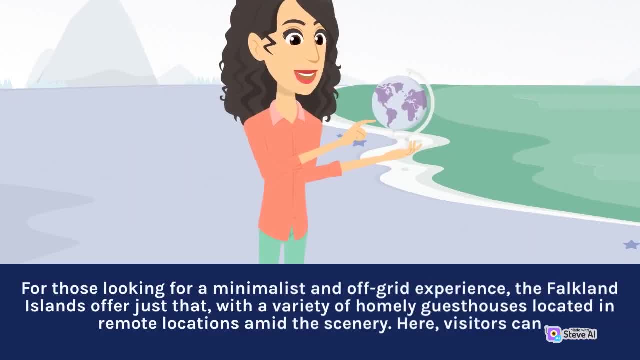 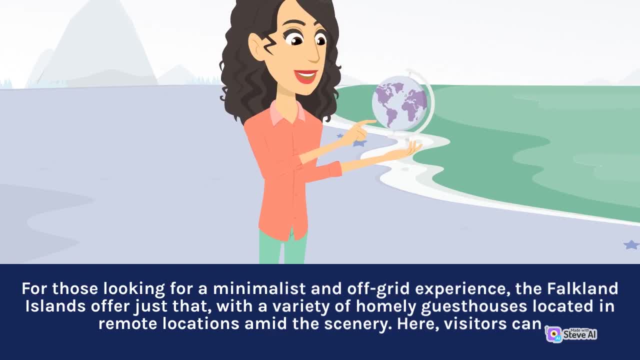 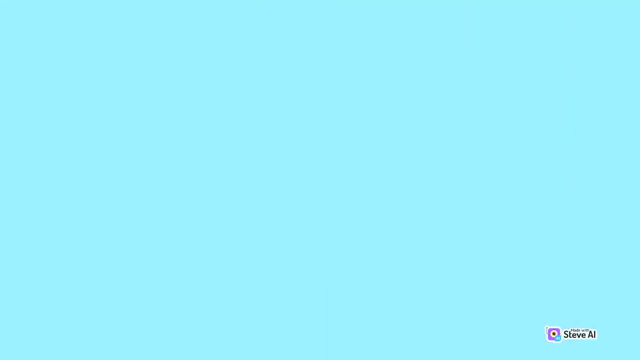 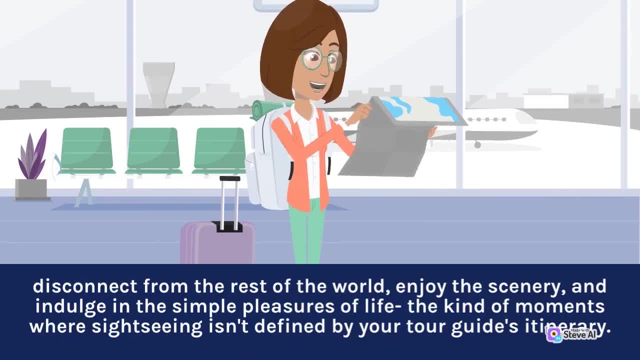 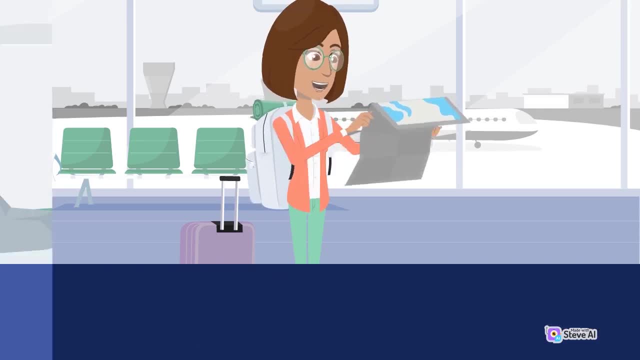 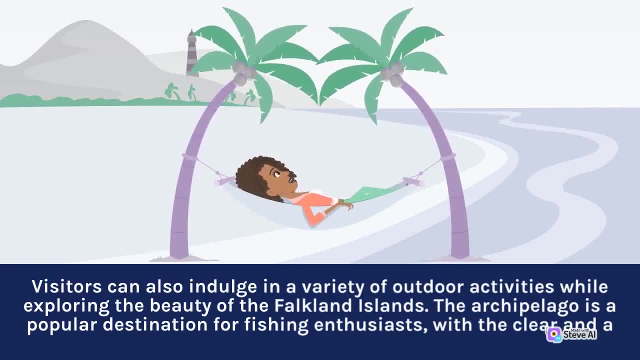 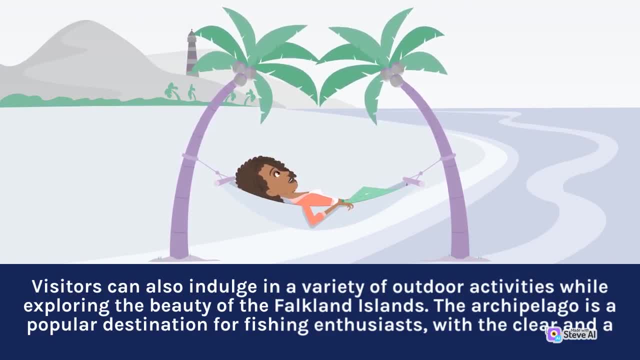 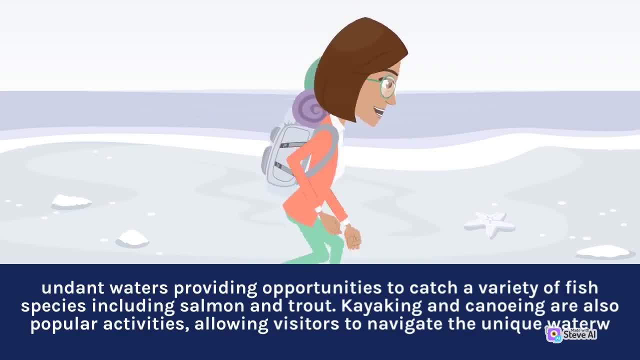 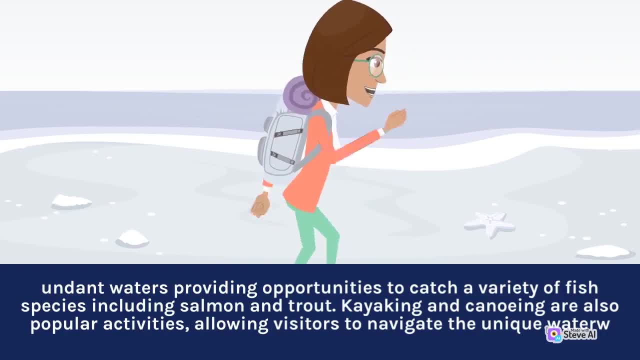 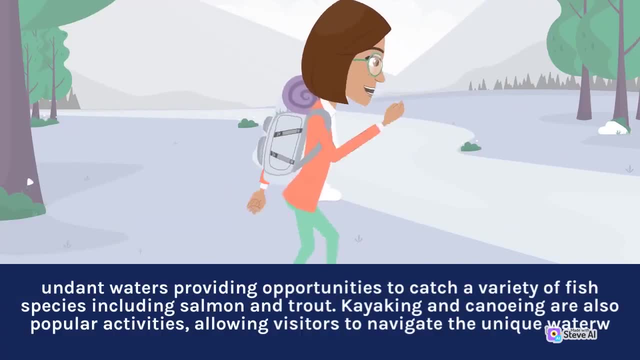 The trails to experience the beauty of the islands up close, taking in the stunning scenery as they go. The trails to experience the beauty of the islands up close, taking in the stunning scenery as they go, allowing visitors to navigate the unique water- Undant waters- providing opportunities to catch a variety of fish species, including salmon. and. 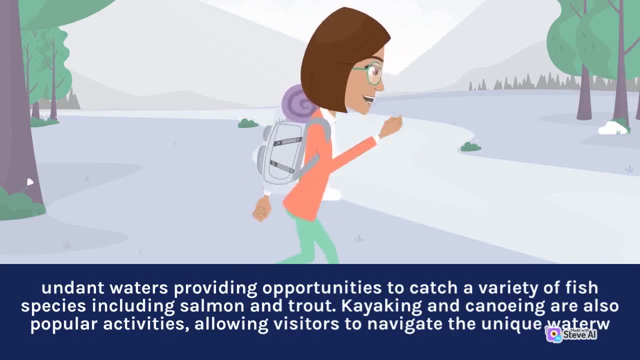 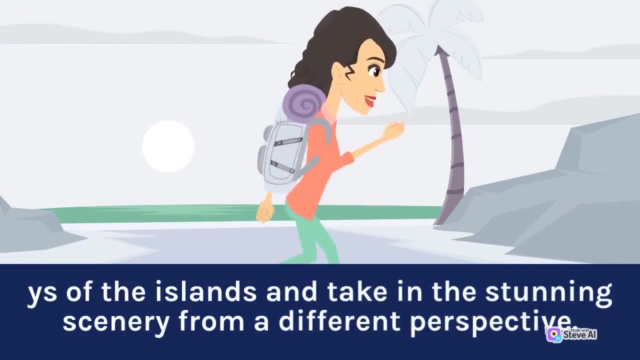 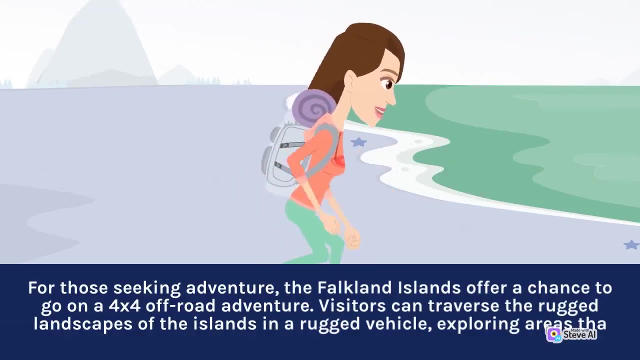 trout Kayaking and canoeing are also popular activities, allowing visitors to navigate the unique water Ease of the islands and take in the stunning scenery from a different perspective. For those seeking adventure, the Falkland Islands offer a chance to go on a four-by-four. 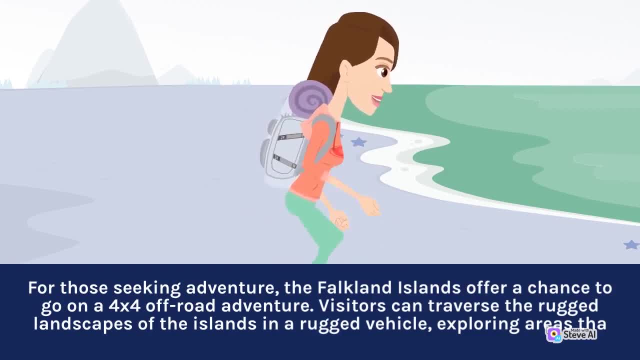 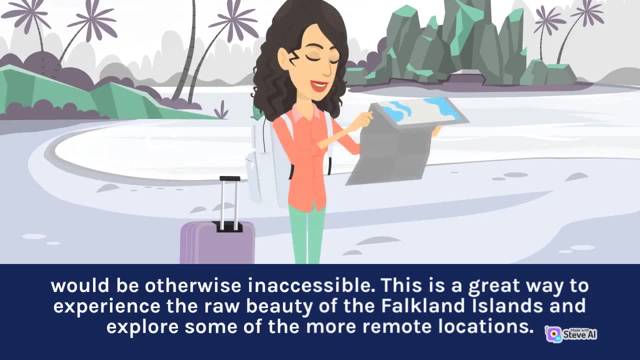 off-road adventure. Visitors can traverse the rugged landscapes of the islands in a rugged vehicle, exploring areas that would be otherwise inaccessible. This is a great way to experience the raw beauty of the Falkland Islands and explore some of the more remote locations Would be otherwise inaccessible. 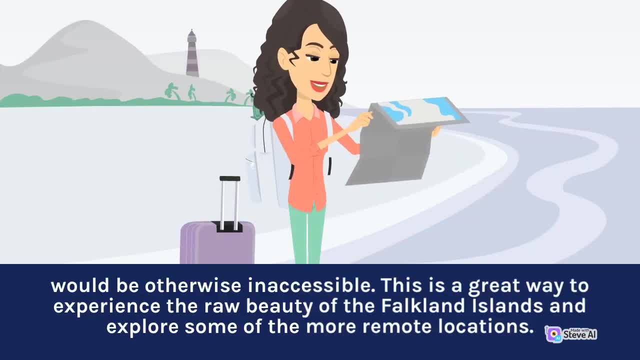 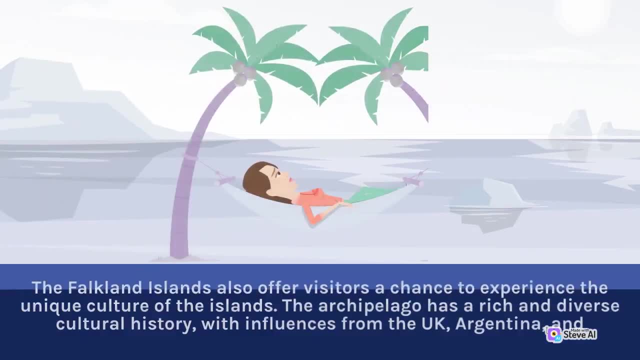 This is a great way to experience the raw beauty of the Falkland Islands and explore some of the more remote locations. The Falkland Islands also offer visitors a chance to experience the unique culture of the islands. The archipelago has a rich and diverse cultural history, with influences from the UK, Argentina. 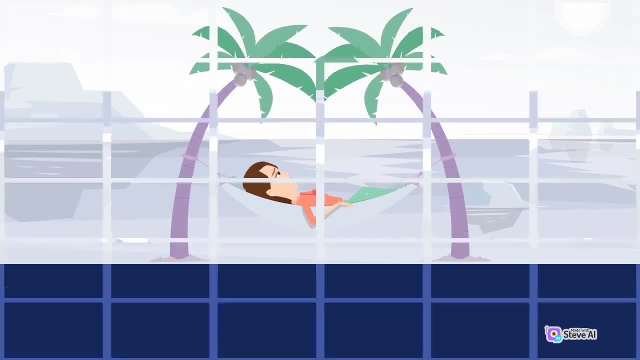 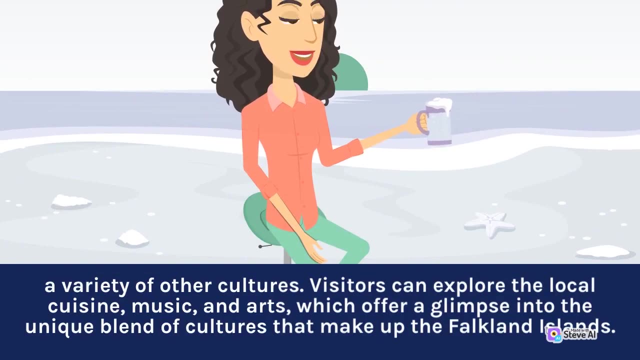 and a variety of other cultures. Visitors can explore the local quarters, the local parks and the local museums. Visitors can also explore the local cuisine, music and arts, which offer a glimpse into the unique blend of cultures that make up the Falkland Islands. 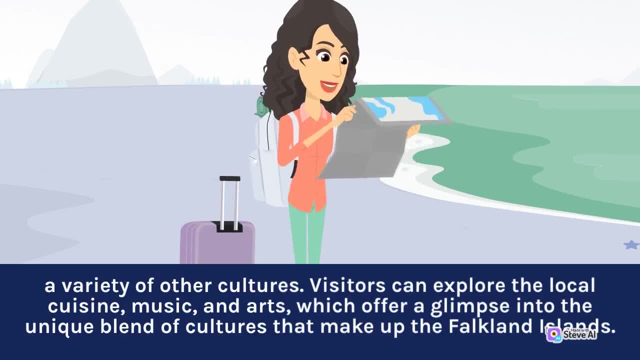 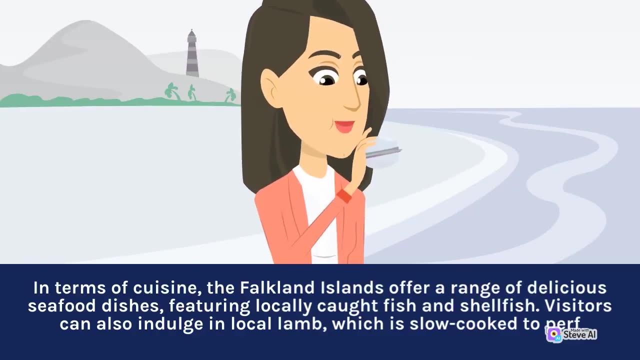 A variety of other cultures. Visitors can explore the local cuisine, music and arts, which offer a glimpse into the unique blend of cultures that make up the Falkland Islands. In terms of cuisine, the Falkland Islands offer a range of delicious seafood dishes, featuring locally caught fish and shellfish. 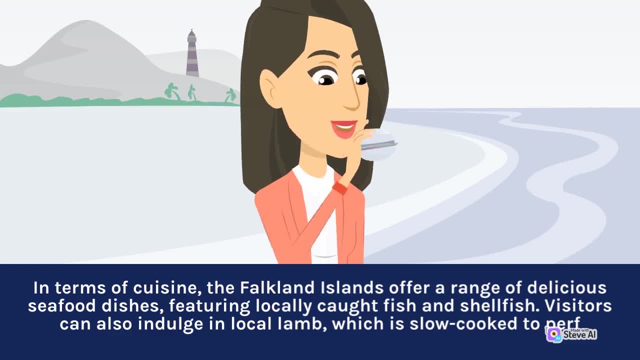 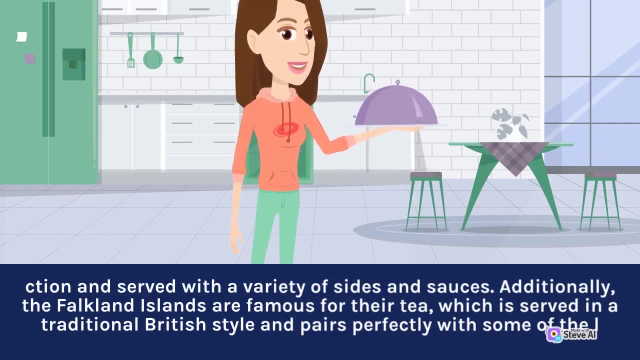 Visitors can also indulge in local lamb, which is slow cooked to exposing łos that are popular with lowinin. when these dishes are cooked, the Но Emigrés of the island have bamboo crowns, And this dish is ahead of the event and should be presented as an怕 pеж, which meant to ein dulu das ф? liquid. 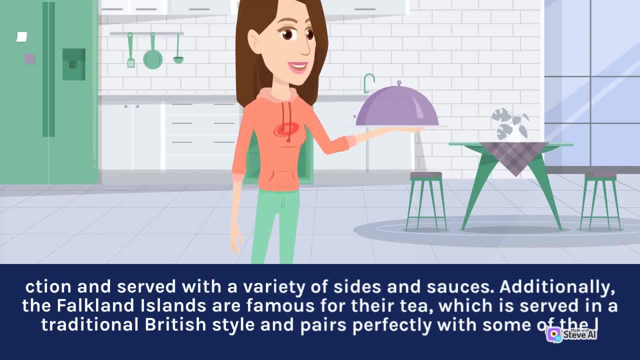 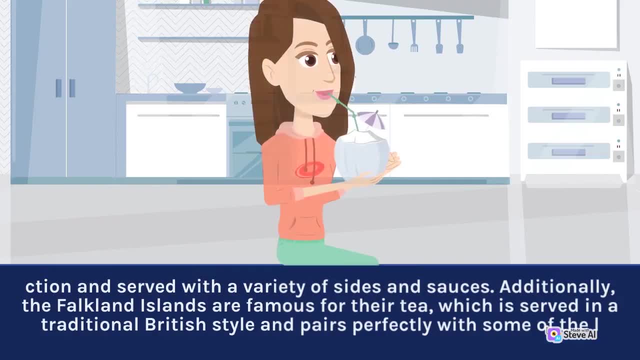 Additionally, the Falkland Islands are famous for their tea, which is served in a traditional British style and pairs perfectly with some of the Anitta of Ayrton and Dortmund specialty. Kayokes können tau gewinnen, an association compilat ther and served with a variety of sides and sauces. Xinnan, served with a variety of sides and sauces: those of Ayrton, Jenny, Strawberry. 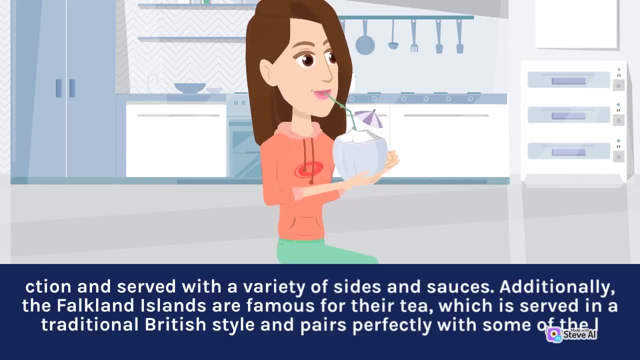 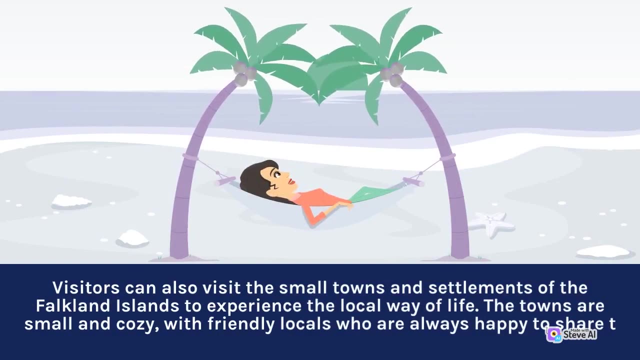 and sauces. Additionally, the Falkland Islands are famous for their tea, which is served in a traditional British style and pairs perfectly with some of the El CalSweet Treats. Visitors can also visit the small towns and settlements of the Falkland Islands to experience. 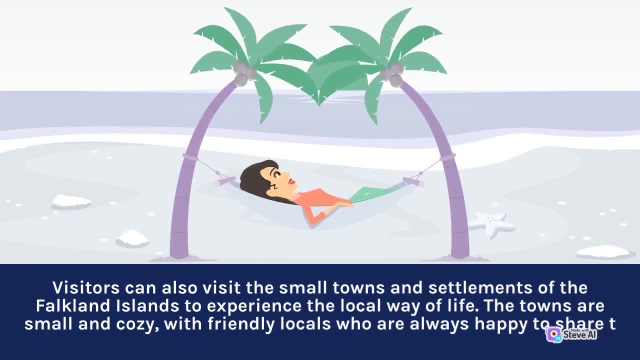 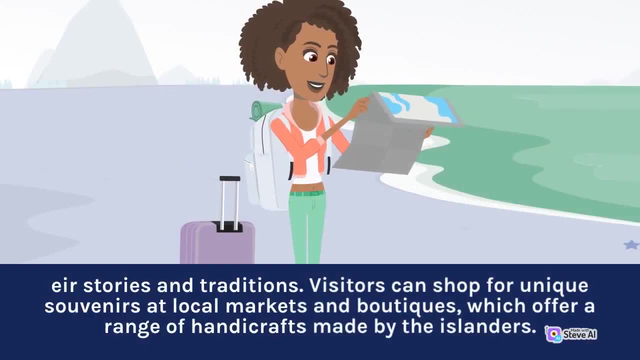 the local way of life. The towns are small and cozy, with friendly locals who are always happy to share tea, Air, Stories and Traditions. Visitors can shop for unique souvenirs at local markets and boutiques, which offer a range of handicrafts made by the islanders. 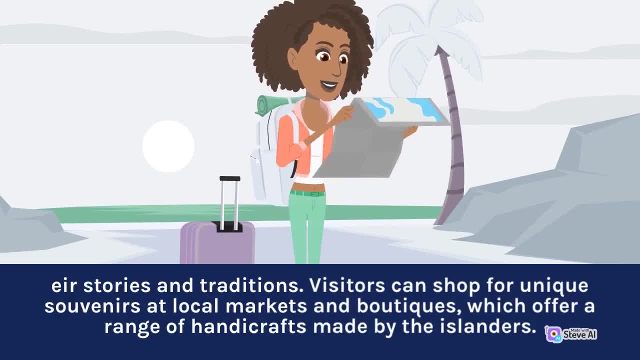 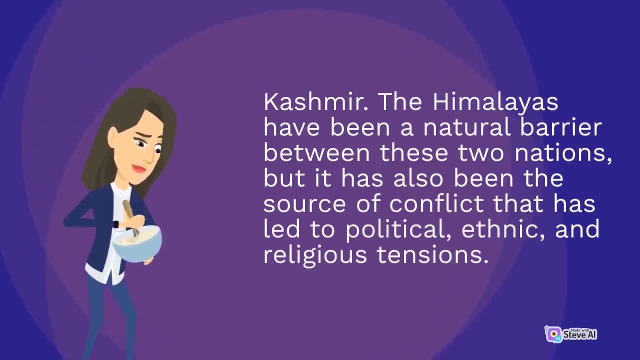 One of the most unique and popular local food is the Falkland Island Tea Kashmir. The Himalayas have been a natural barrier between these two nations, but it has also been the source of conflict that has led to political, ethnic and religious tensions. 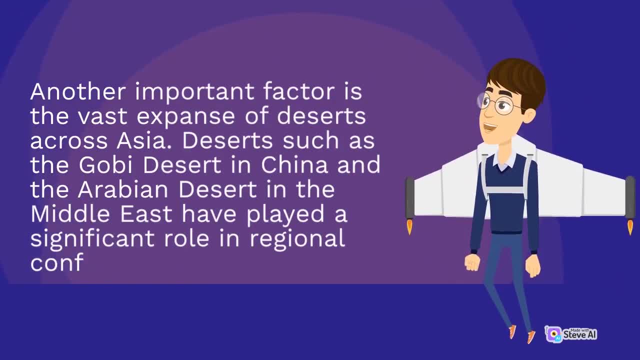 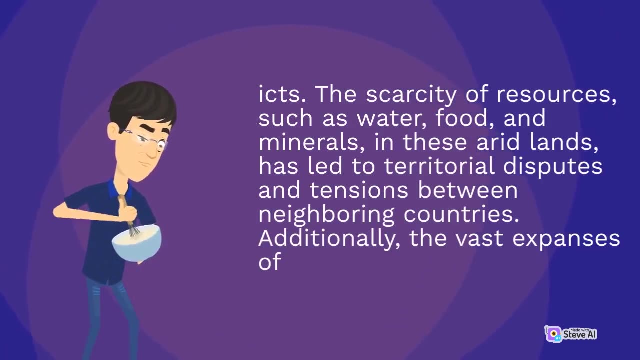 Another important factor is the vast expanse of deserts across Asia. Deserts such as the Gobi Desert in China and the Arabian Desert in the Middle East have played a significant role in regional conference Ix. The scarcity of resources such as water, food and minerals in these arid lands has led to territorial disputes and tensions between neighboring countries. 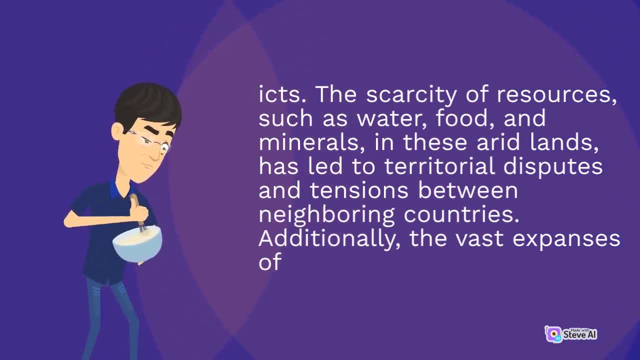 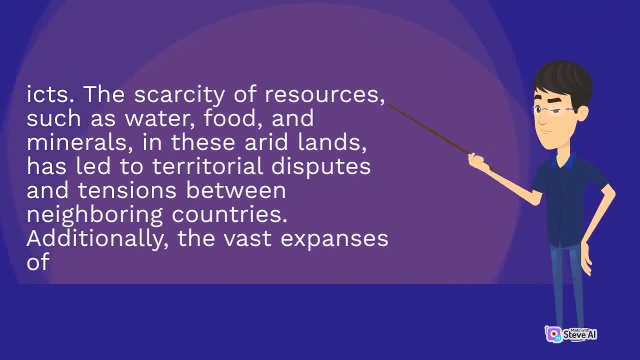 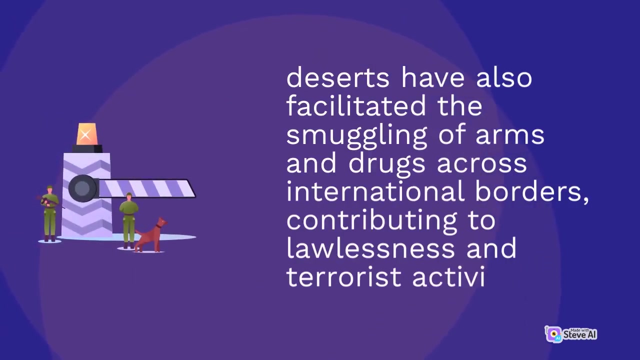 Additionally, the vast expanses of Ix. The scarcity of resources such as water, food and minerals in these arid lands has led to territorial disputes and tensions between neighboring countries. Additionally, the vast expanses of Ix Deserts have also facilitated the smuggling of arms and drugs across international borders, contributing to lawlessness and terrorist activities. 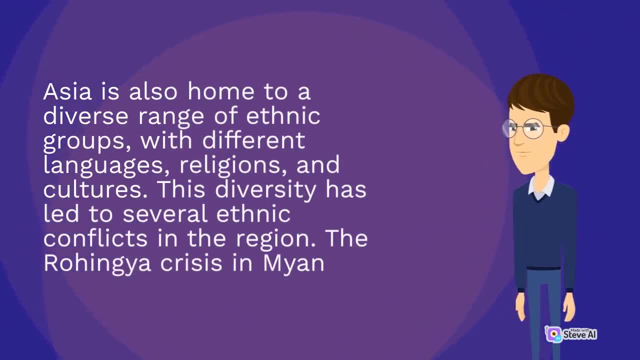 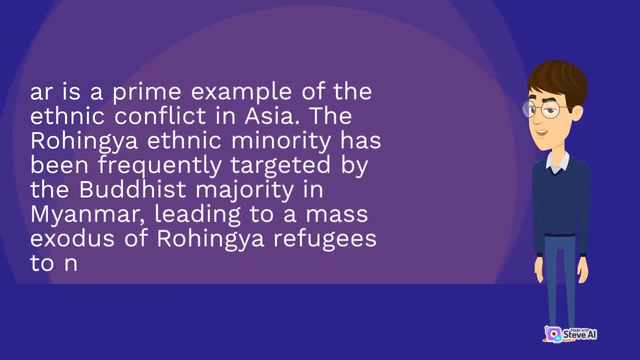 Rohingya Crisis in Mayan. Rohingya Crisis in Mayan. Rohingya Crisis in Mayan- prime example of the ethnic conflict in Asia. The Rohingya ethnic minority has been frequently targeted by the Buddhist majority in Myanmar, leading to a mass exodus of Rohingya refugees to N? R is a prime example of the ethnic conflict in Asia. The Rohingya ethnic minority has been frequently targeted by the Buddhist majority in Myanmar, leading to a mass exodus of Rohingya refugees to N I bring, Bangladesh. This conflict has been fueled by religious and ethnic differences, with the Rohingya being viewed as illegal immigrants and outsiders by the Myanmar government. 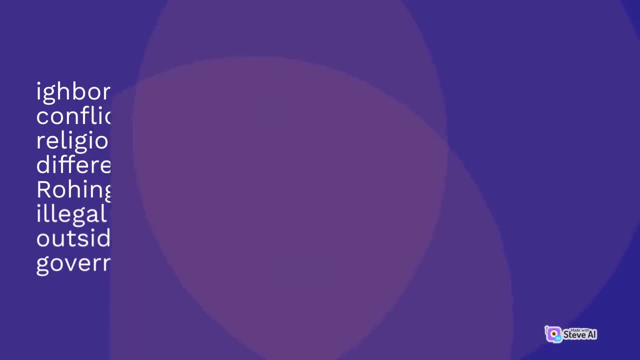 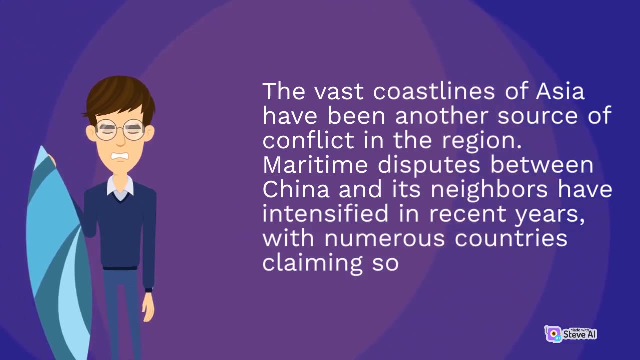 Similarly, the C. The vast coastlines of Asia have been another source of conflict in the region. Maritime disputes between China and its neighbors have intensified in recent years, with numerous countries claiming so Reedy over islands and reefs in the South China Sea. These conflicts are mainly territorial in 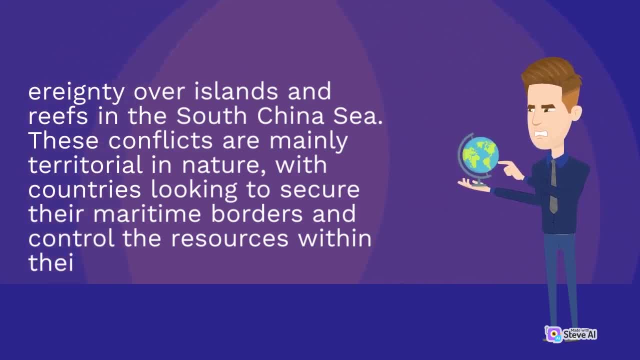 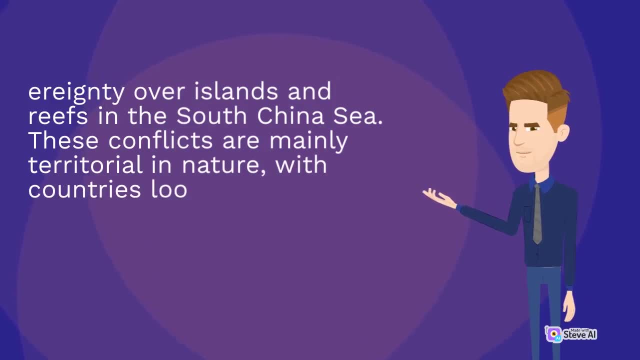 nature, with countries looking to secure their maritime borders and control the resources within the eye, Reedy over islands and reefs in the South China Sea. These conflicts are mainly territorial in nature, with countries looking to secure their maritime borders and control the resources within the eye. 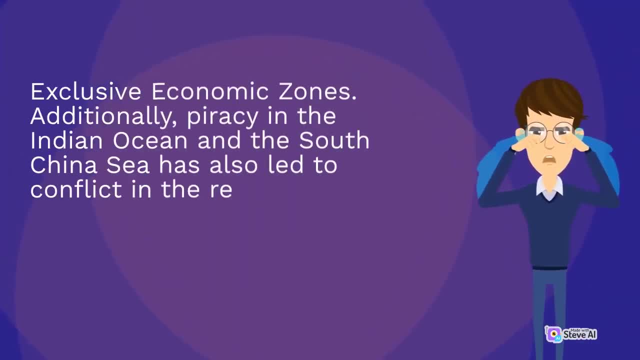 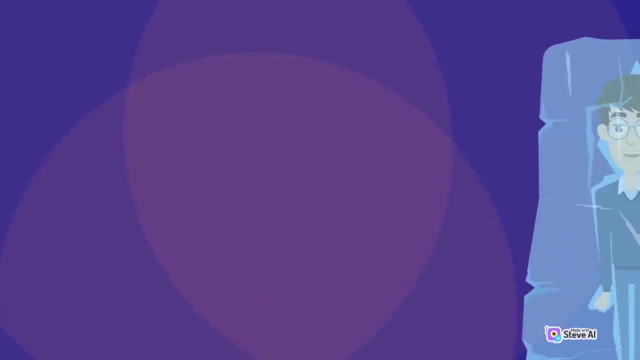 Exclusive economic zones. Additionally, piracy in the Indian Ocean and the South China Sea is also led to conflict in the region. Pirates from Somalia and Southeast Asia have targeted commercial SH. Asia is also home to several active volcanoes and earthquake zones- The Ring of Fire. 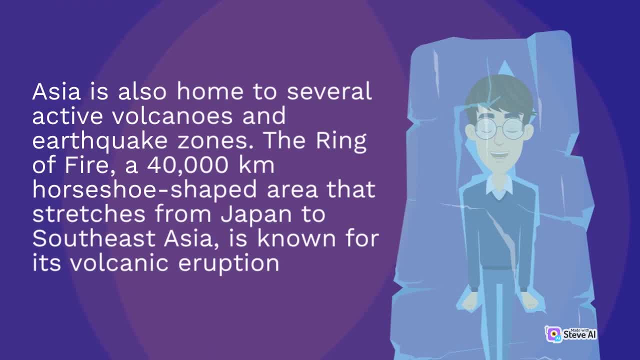 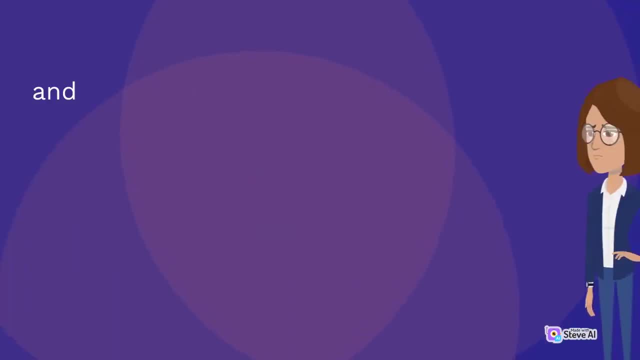 a 40,000 kilometers horseshoe-shaped area that stretches from Japan to Southeast Asia, is known for its volcanic eruptions. Human resources and others are certified by the exchange somewhere in the region, whether it's this base or another area in Indonesia. 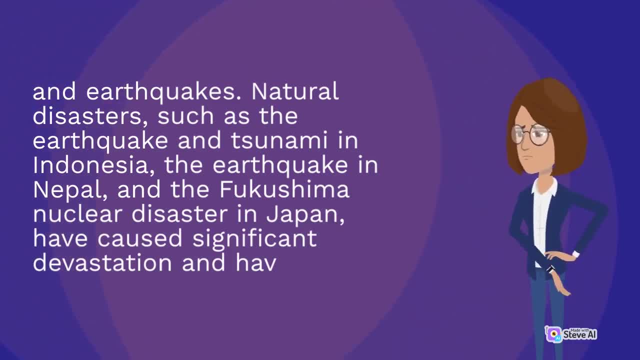 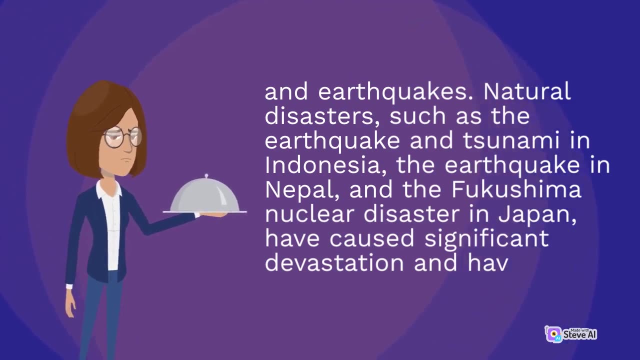 And earthquakes. Natural disasters such as the earthquake and tsunami in Indonesia, the earthquake in Nepal and the Fukushima nuclear disaster in Japan have caused significant devastation and have affected 13 super narrow-scale Darling's Triangle Earthquakes. natural disasters such as the earthquake and tsunami in Indonesia. the earthquake in Nepal. 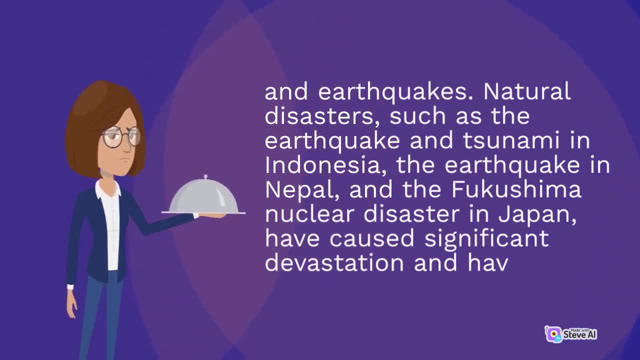 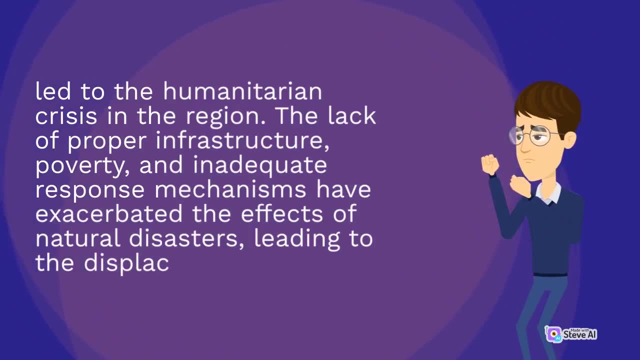 and the Fukushima nuclear disaster in Japan have caused significant devastation and have caused significant devastation have led to the humanitarian crisis in the region. The lack of proper infrastructure, poverty and inadequate response mechanisms have exacerbated the effects of natural disasters, leading to the disblack. Finally, economic disparities and poverty are also key driving. 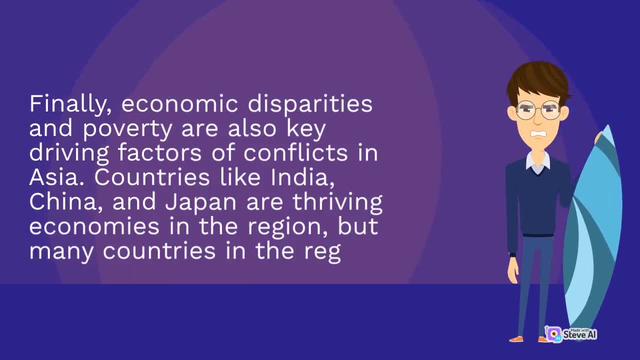 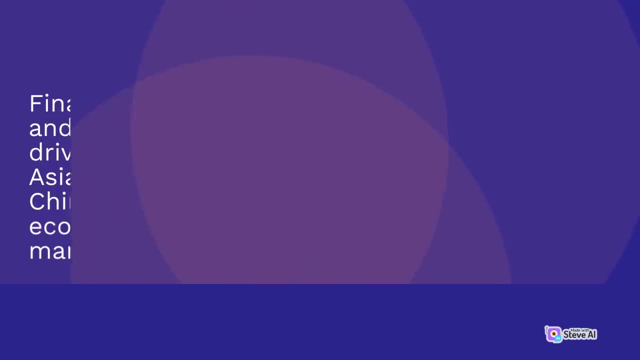 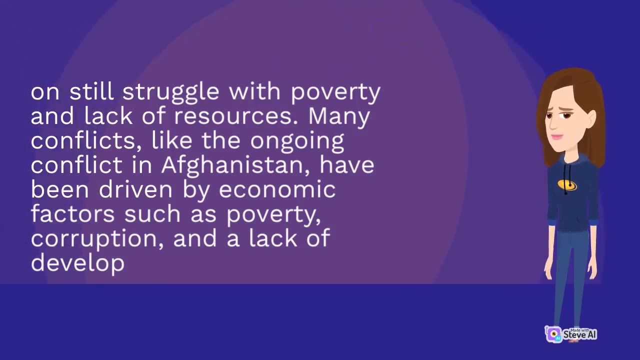 factors of conflicts in Asia. Countries like India, China and Japan are thriving economies in the region, but many countries in the reg On still struggle with poverty and lack of resources. Many conflicts, like the ongoing conflict in Afghanistan, have been driven. 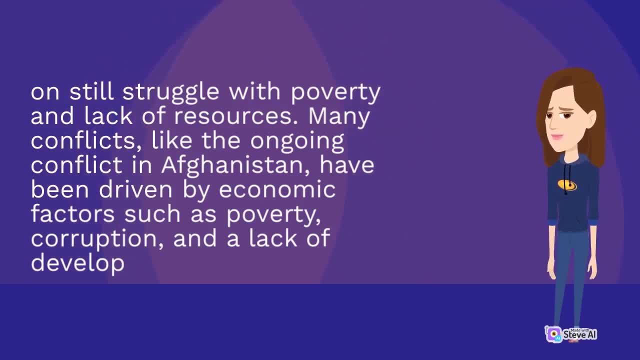 by economic factors such as poverty, corruption and a lack of develop. On still struggle with poverty and lack of resources. Many conflicts, like the ongoing conflict in Afghanistan, have been driven by economic factors such as poverty, corruption and a lack of develop. 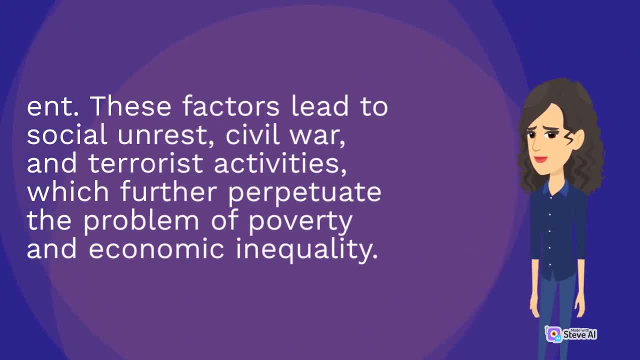 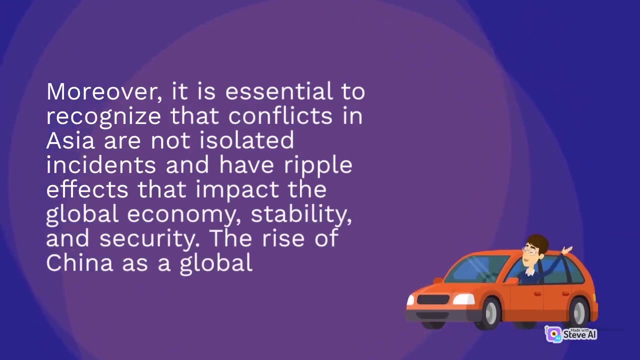 And these factors lead to social unrest, civil war and terrorist activities, which further perpetuate the problem of poverty and economic inequality. Moreover, it is essential to recognize that conflicts in Asia are not isolated incidents and have ripple effects that impact the global economy, stability and security. The rise of 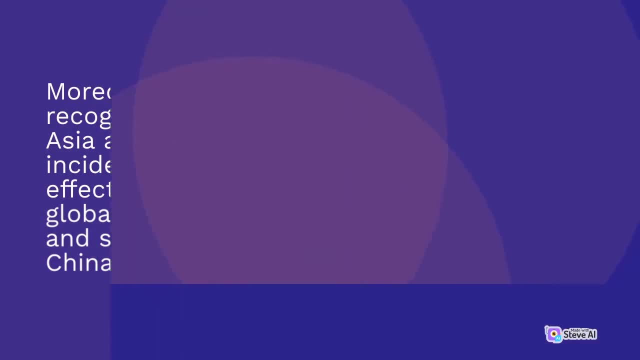 China is a clear example of this. The rise of China is a clear example of the rise of China. Unofficiously, China is a proud to have incorporated immenseazed innovation and плат 항상. Information goes out to the world Without the whole world. that can't adapt to our current price. people like China would 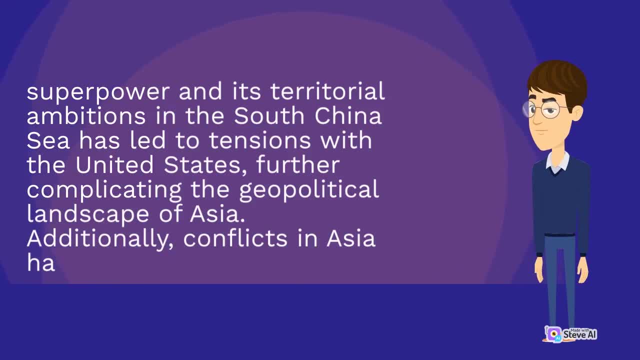 not be able to calm the economy down. Breaking News: China is now currently facing long-term trade wars. The South China Sea is надing the liability in its territory, and thereof the US is toeija saying that China isibi track. So far, the South China Sea has been under seize enfzzing, and 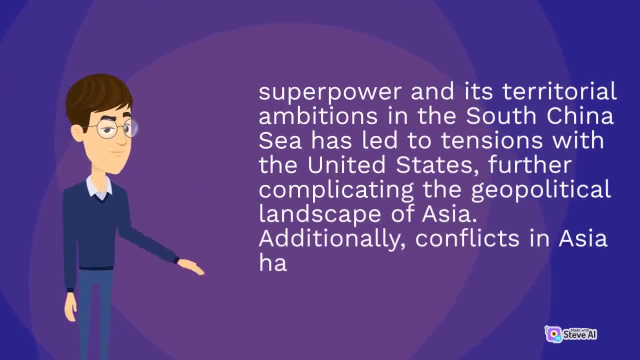 llesing until 70 years ago, a period of increased turmoil to fight the world war. It is an earlymenoing of China's inter 1944 economic development, while getting even worse 있거든요. China is now 아직atic to keep its anchor til 2017�. 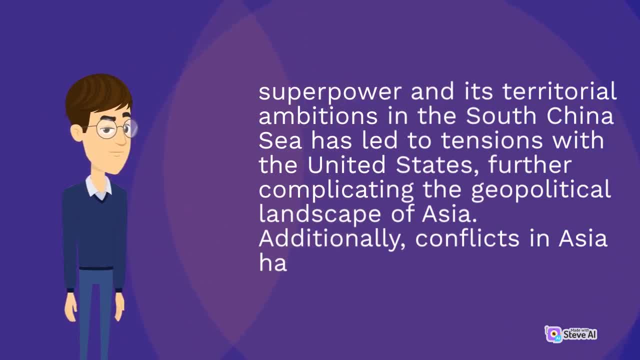 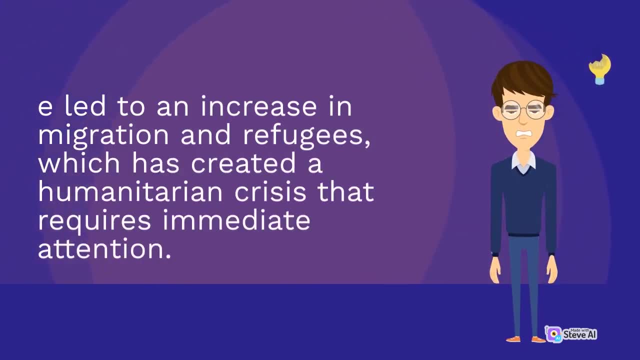 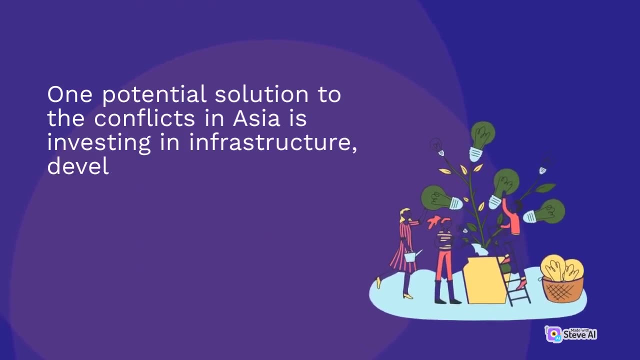 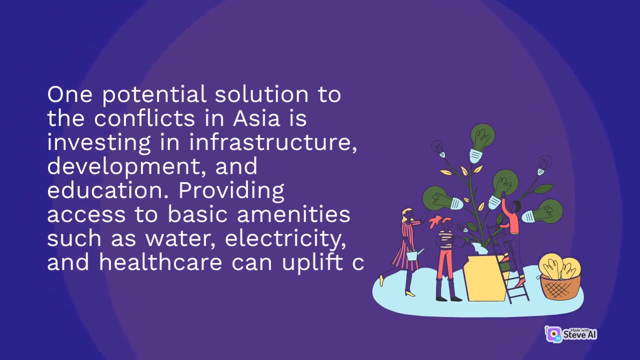 Malaysia GDP. The Chinese intermediary online business Eally app has agreed toπ. E led to an increase in migration and refugees, which has created a humanitarian crisis that requires immediate attention. One potential solution to the conflicts in Asia is investing in infrastructure development and education, Providing access to basic amenities such as water. 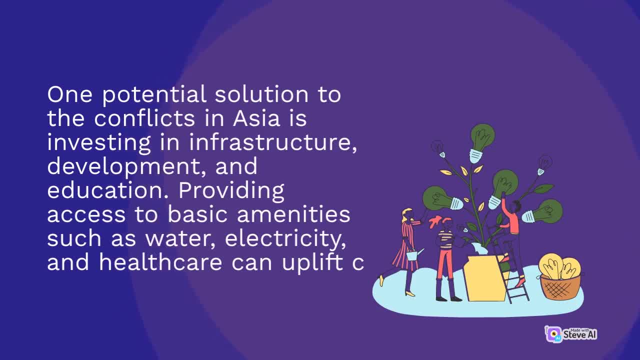 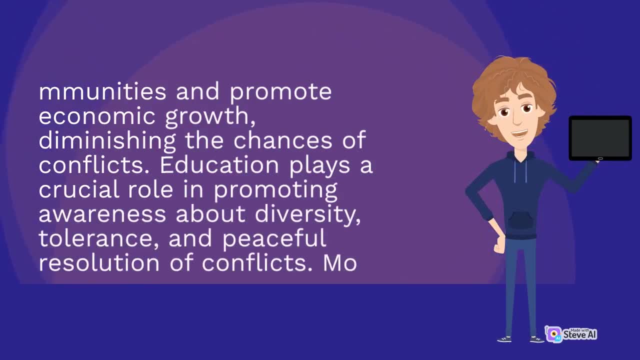 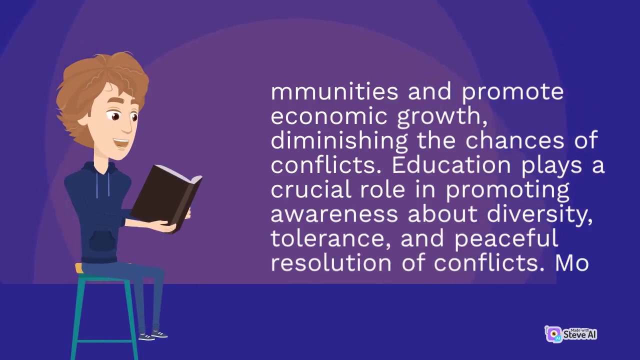 electricity and healthcare can uplift sea Munities and promote economic growth, diminishing the chances of conflicts. Education plays a crucial role in promoting awareness about diversity, tolerance and peaceful resolution of conflicts, Munities and promote economic growth, diminishing the chances of conflicts. 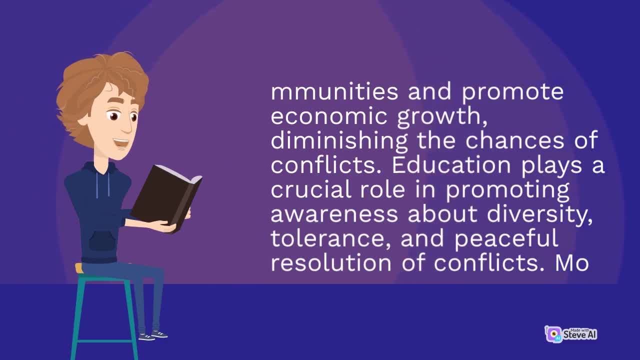 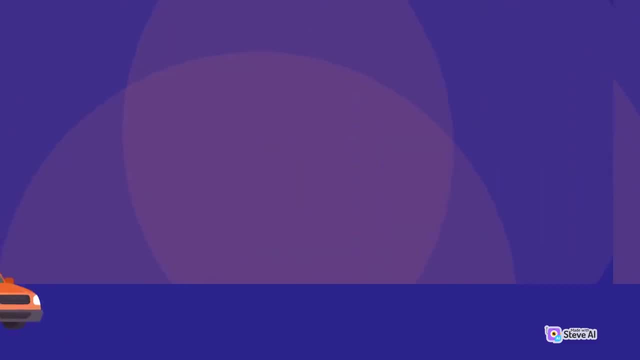 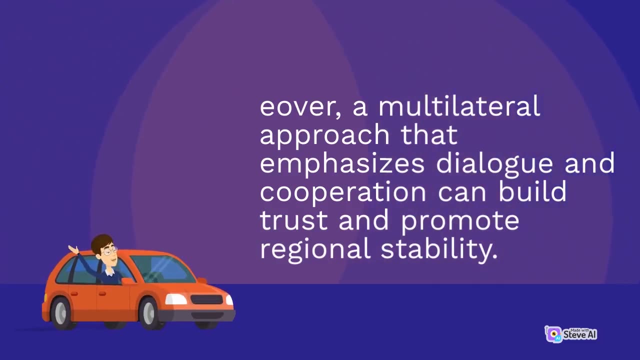 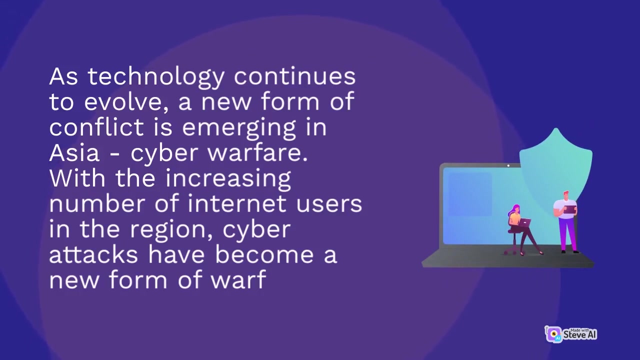 Education plays a crucial role in promoting awareness about diversity, tolerance and peaceful resolution of conflicts Mo Over. a multilateral approach that emphasizes dialogue and cooperation can build trust and promote regional stability. As technology continues to evolve, a new form of conflict is emerging in Asia: cyber warfare. With the increasing number of 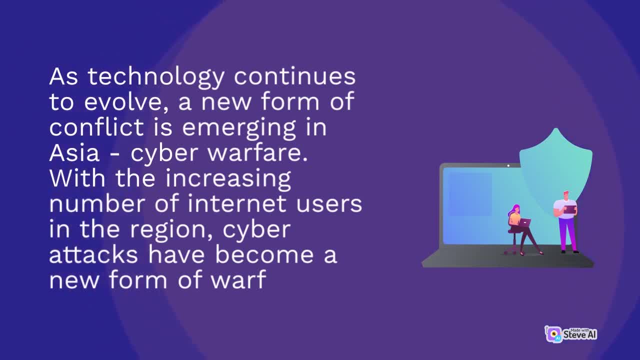 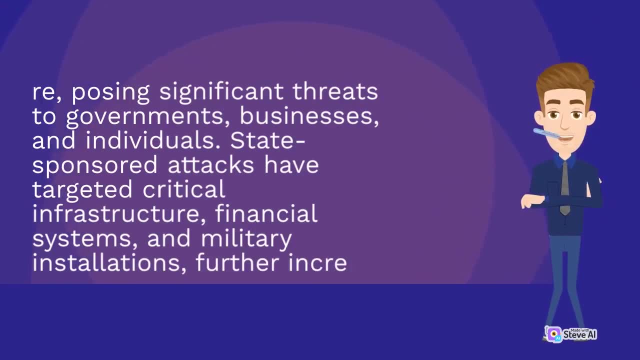 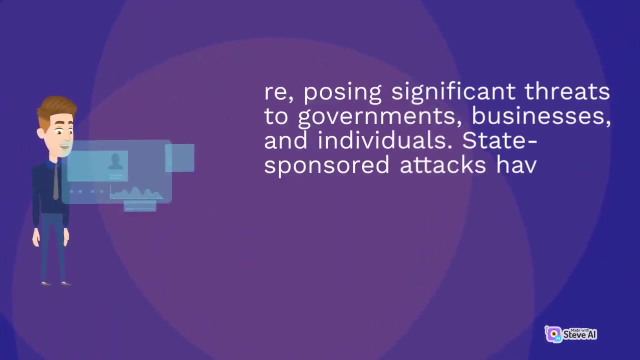 internet users in the region. cyber attacks have become a new form of warf, Re-posing significant threats to governments, businesses and individuals. State-sponsored attacks have targeted critical infrastructure, financial systems and military installations further incur, Re-posing significant threats to governments, businesses and individuals. State-sponsored attacks have targeted critical infrastructure, financial systems and military installations further incur. 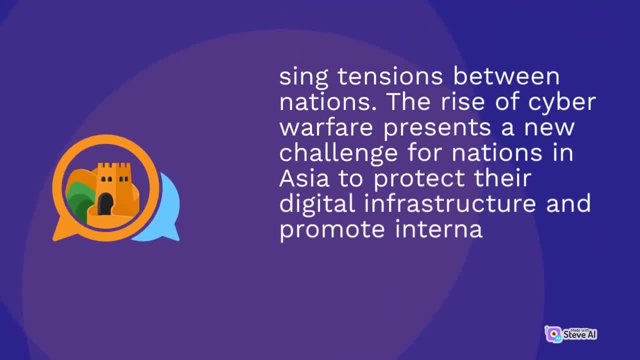 In Asia, theтаwelling of films in the form of crackdowns against North Korean states and regions has led to partisan acts in the form of amputations, rapes and several clashes among independent governments, and generations attacked the North Korean government, Re-posing significant threats to governments, businesses and businesses further incur. 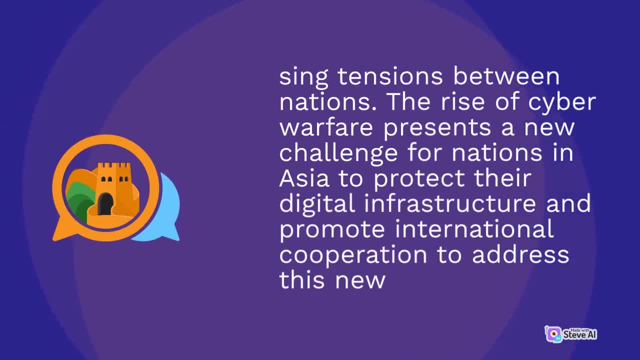 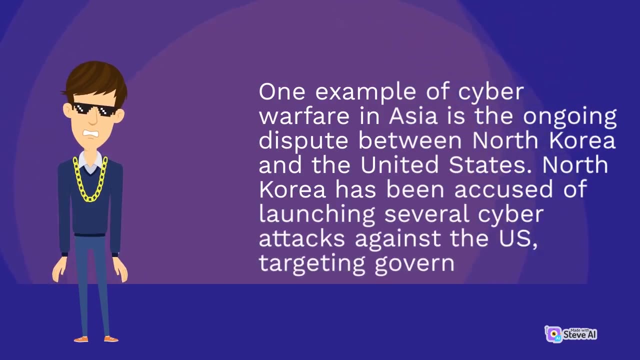 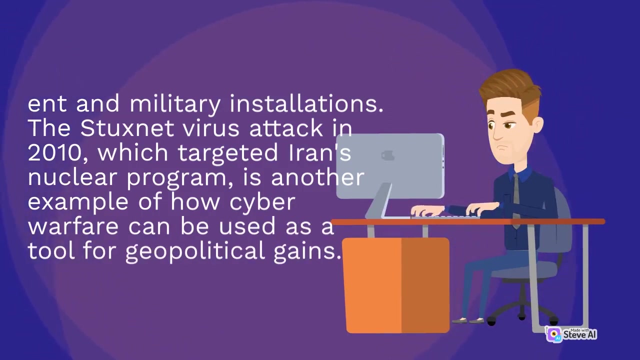 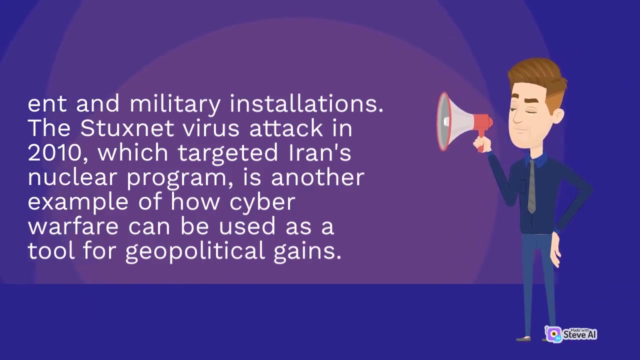 Open �� Royal Flamengo eliminatory and in military installations. The Stuxnet virus attack in 2010, which targeted Iran's nuclear program, is another example of how cyber warfare can be used as a tool for geopolitical gains. and in military installations. The Stuxnet virus attack in 2010, which targeted Iran's 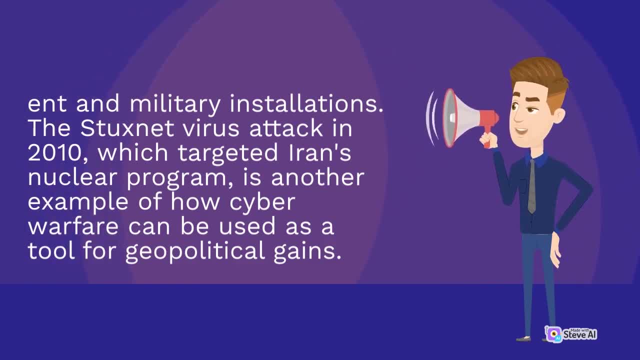 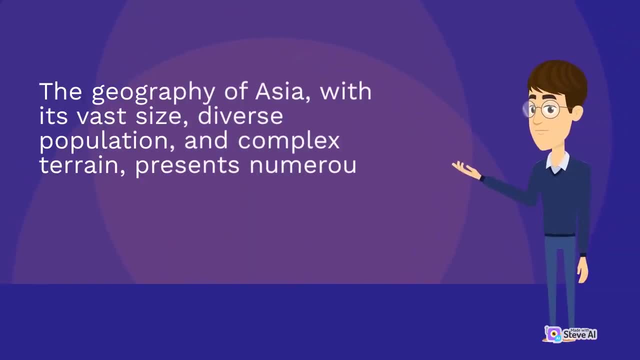 nuclear program is another example of how cyber warfare can be used as a tool for geopolitical gains. The geography of Asia, with its vast size, diverse population and complex terrain, presents numerous challenges for addressing conflicts and promoting peace. However, these challenges also present O. 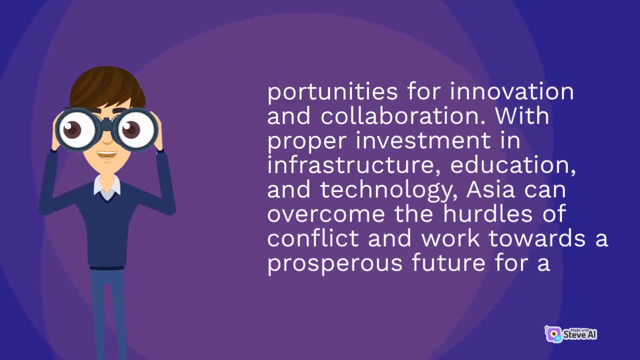 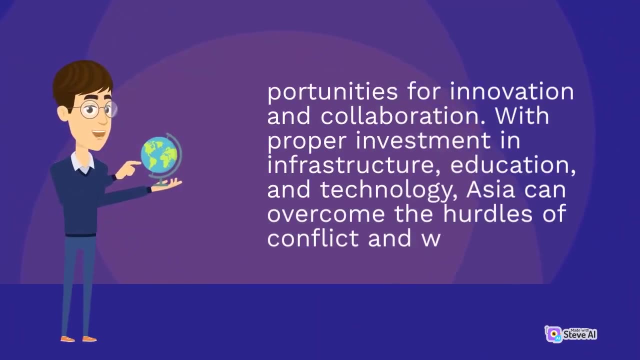 Opportunities for Innovation and Collaboration. With proper investment in infrastructure, education and technology, Asia can overcome the hurdles of conflict and work towards a prosperous future for A Opportunities for Innovation and Collaboration. With proper investment in infrastructure, education and technology, Asia can overcome the hurdles of. 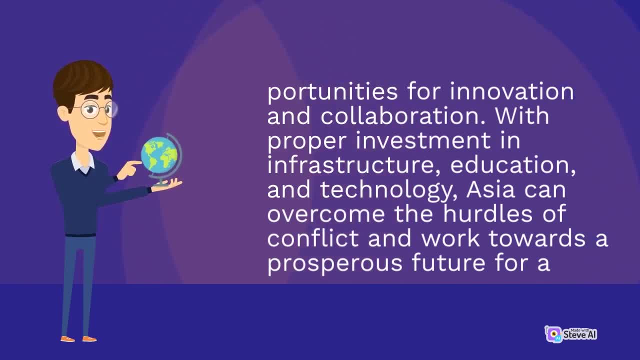 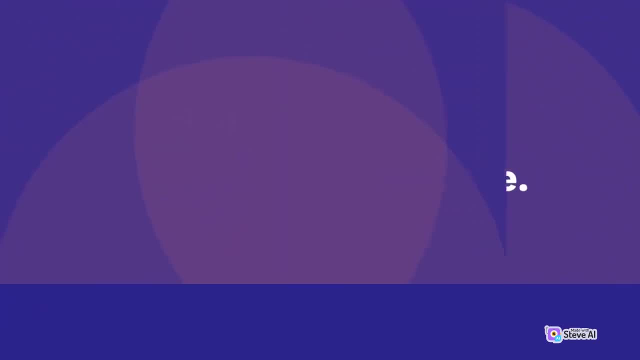 conflict and work towards a prosperous future for A Opportunities for Innovation and Collaboration. With proper investment in infrastructure, education and technology, Asia can overcome the hurdles of conflict and work towards a prosperous future for A? L Its people. Moreover, it is essential to recognize the role of international organizations in promoting peace. 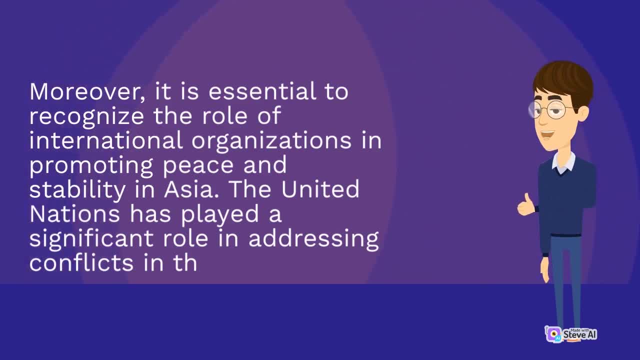 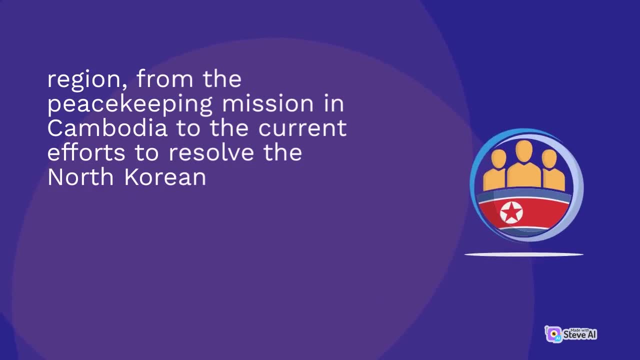 and stability in Asia. The United Nations has played a significant role in addressing conflicts in TH Region, from the peacekeeping mission in Cambodia to the current efforts to resolve the Nordic conflict. Asia has played a significant role in addressing conflicts in TH- the North Korean nuclear crisis, Regional organizations such as the Association of Southeast Asian 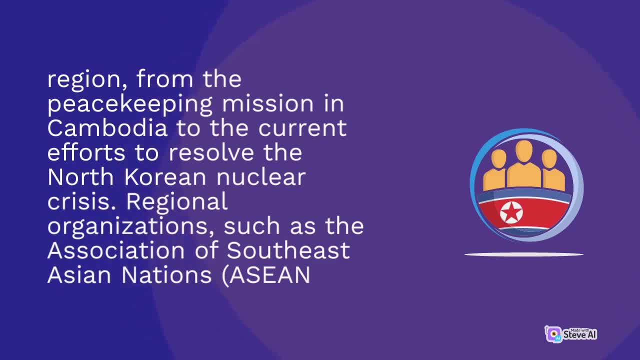 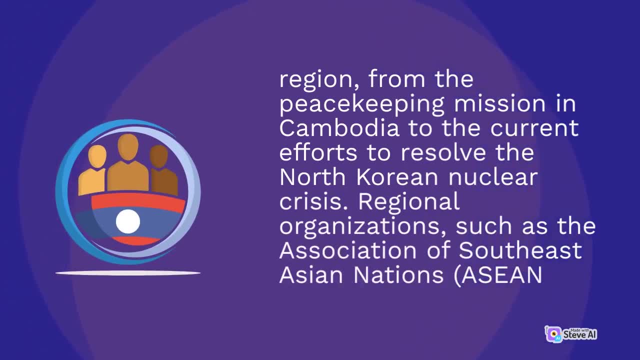 Nations ASEAN Region, from the peacekeeping mission in Cambodia to the current efforts to resolve the North Korean nuclear crisis, Regional organizations such as the Association of Southeast Asian Nations, ASEAN, Have also played an essential role in promoting cooperation and cooperation between ASEAN and. 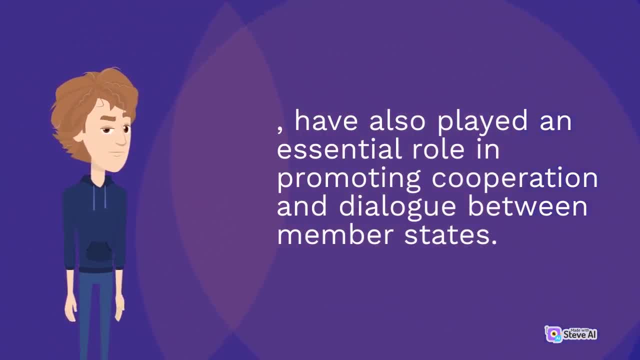 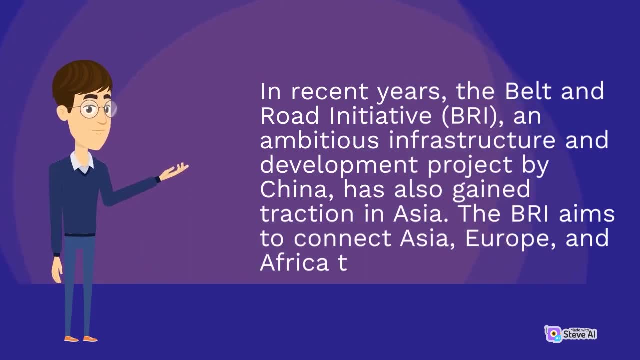 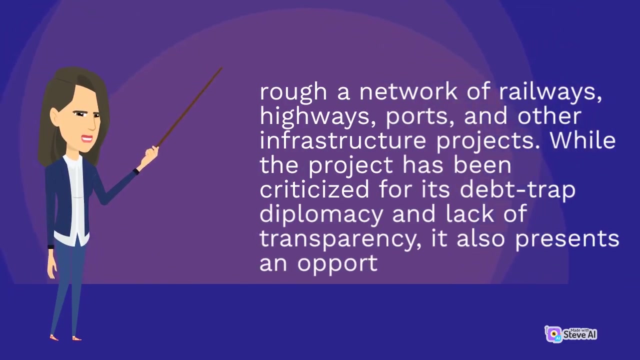 and dialogue between member states. In recent years, the Belt and Road Initiative, BRI, an ambitious infrastructure and development project by China, has also gained traction in Asia. The BRI aims to connect Asia, Europe and Africa t rough a network of railways, highways, ports and other infrastructure projects. 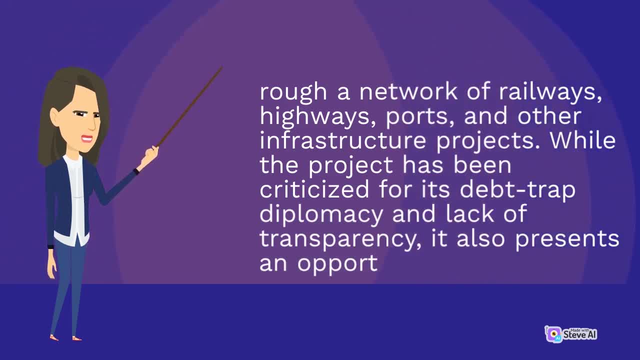 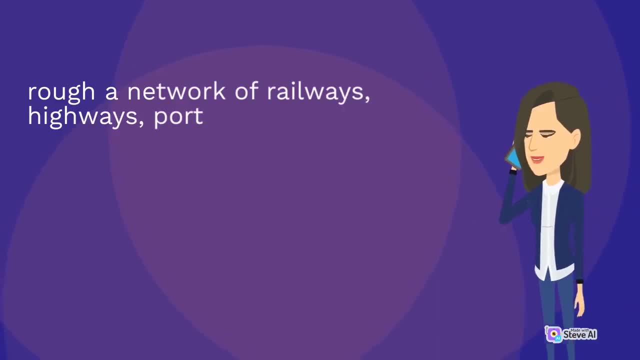 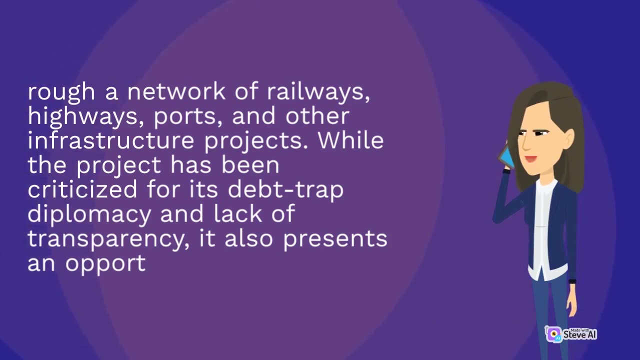 While the project has been criticized for its debt-trap diplomacy and lack of transparency, it also presents an opert rough a network of railways, highways, ports and other infrastructure projects. While the project has been criticized for its debt-trap diplomacy and lack of transparency, 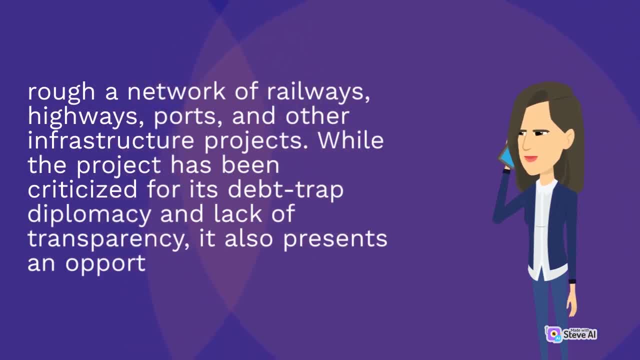 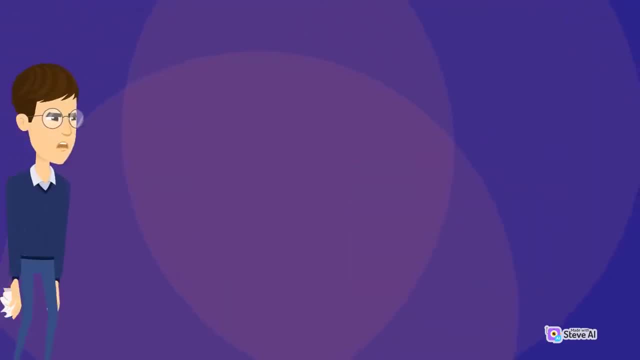 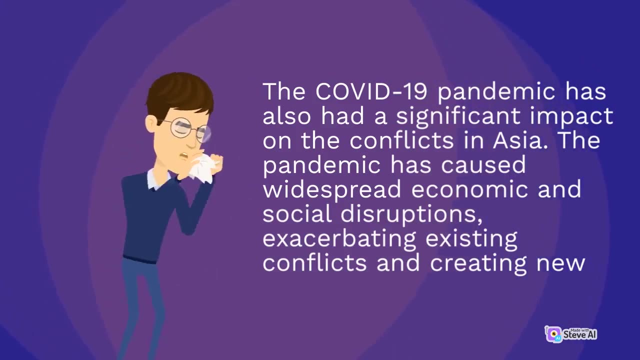 it also presents an opert NIDI for Economic Integration and Cooperation in the Region. The COVID-19 pandemic has also had a significant impact on the conflicts in Asia. The pandemic has caused widespread economic and social disruptions, exacerbating existing conflicts and creating new. 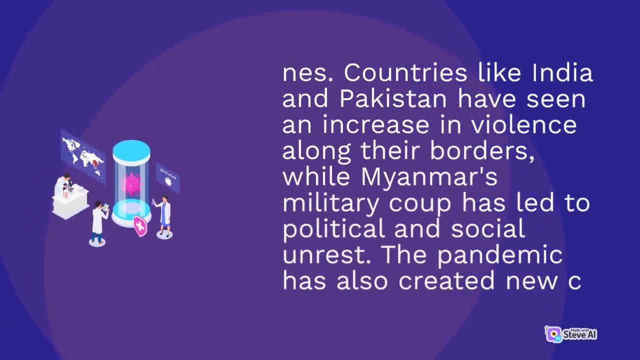 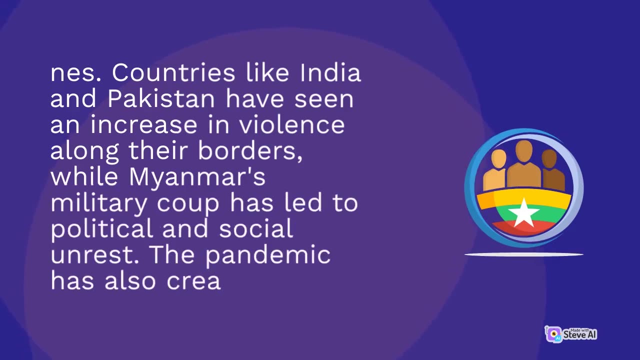 NESS. Countries like India and Pakistan have seen an increase in violence along their borders, while Myanmar's military coup has led to political and social unrest. The pandemic has also created new sea Allenges for vulnerable populations like refugees and migrant workers, who face added. 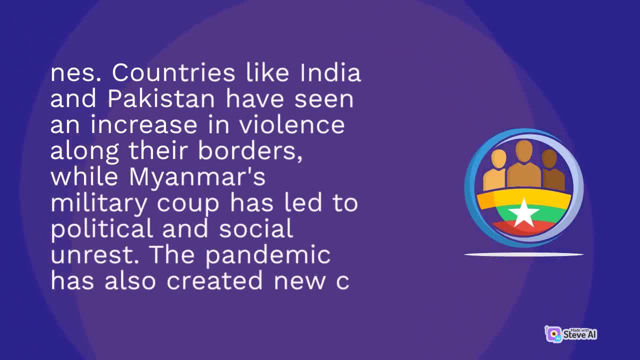 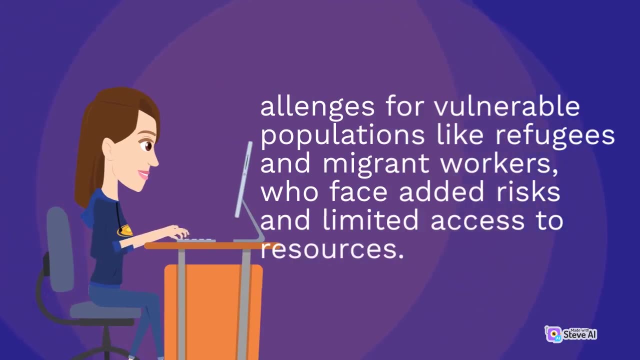 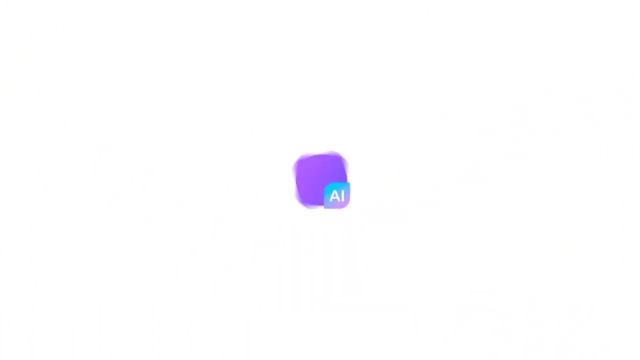 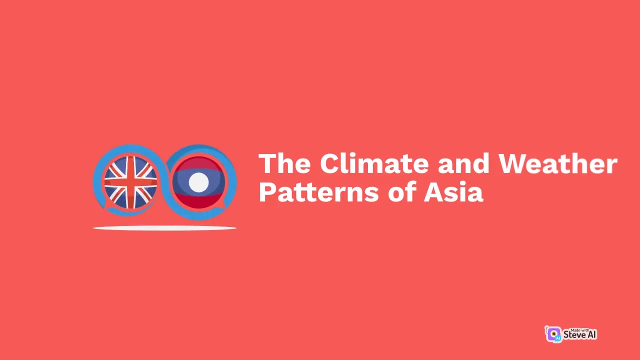 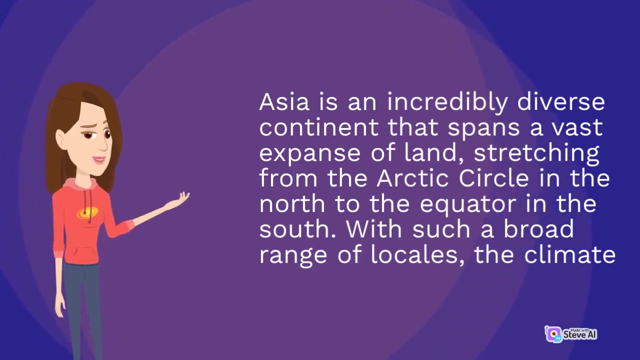 risks and limited access to resources. NEDRASCAM, Andrea M. The Climate and Weather Patterns of Asia. Asia is an incredibly diverse continent that spans a vast expanse of land stretching from the Arctic Circle in the north to the equator in the south. With such a broad range of locales, the climate 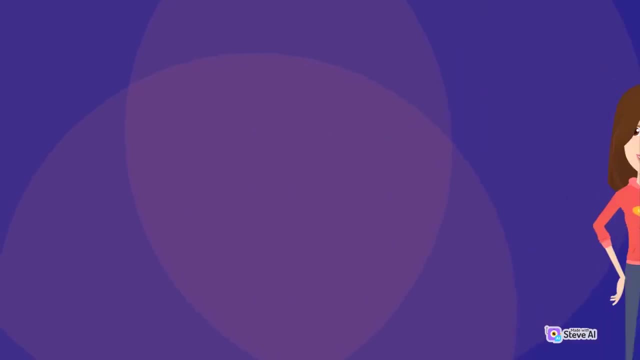 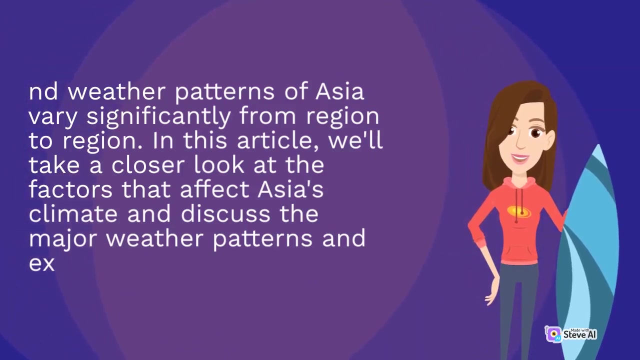 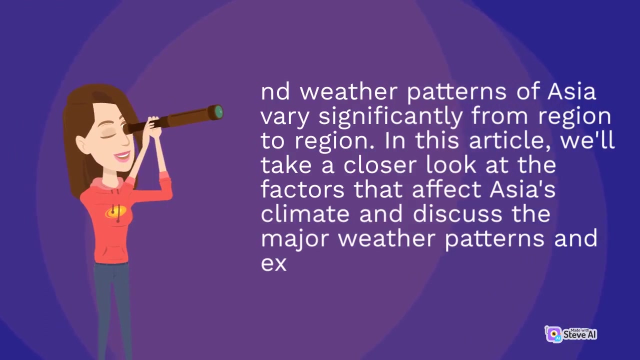 and weather patterns of Asia vary significantly from region to region. In this article, we'll take a closer look at the factors that affect Asia's climate and discuss the major weather patterns in X- ND. weather patterns of Asia vary significantly from region to region. In this article, we'll take a closer look at the factors that affect Asia's climate and discuss the major weather patterns in X. 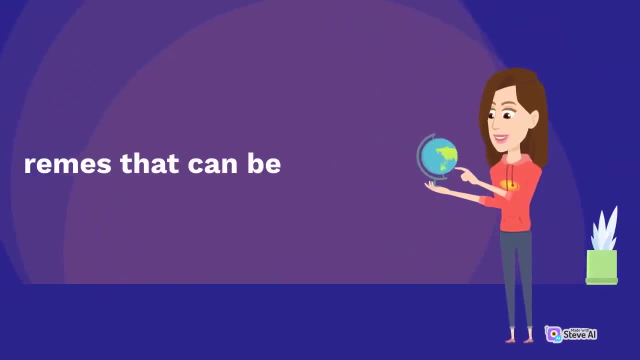 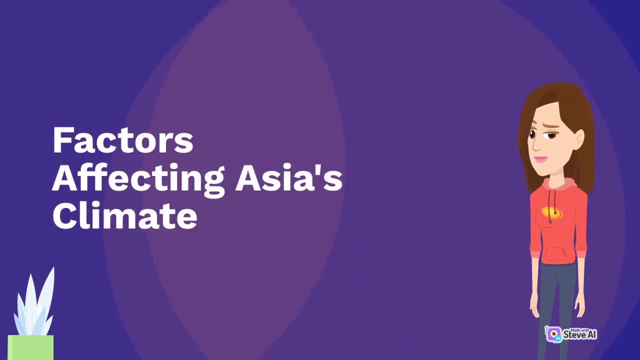 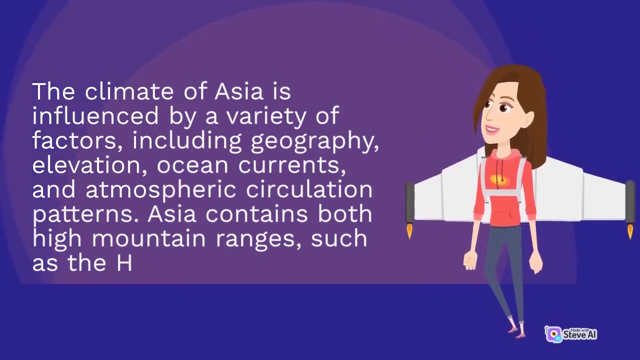 Remes that can be found across the continent. Factors Affecting Asia's Climate. The climate of Asia is influenced by a variety of factors, including geography, elevation, ocean currents and atmospheric circulation patterns. Asia contains both high mountain ranges, such as the H 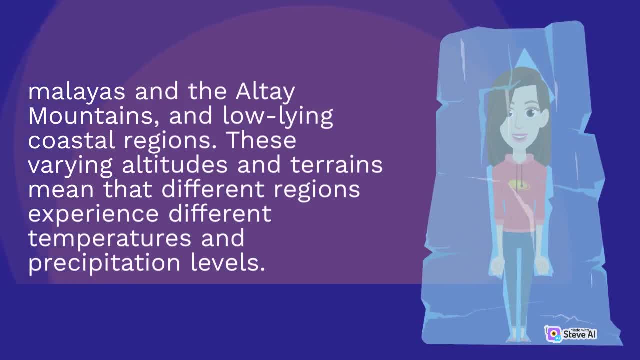 Malayas and the Aztecs Malayas and the Aztecs Malayas and the Aztecs Malayas and the Altai Mountains and low-lying coastal regions. These varying altitudes and terrains mean that different regions experience different temperatures and precipitation levels. 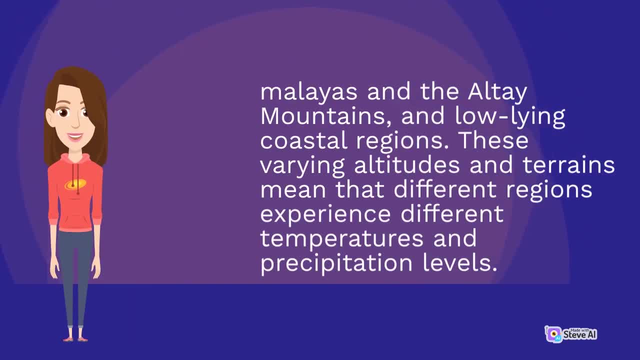 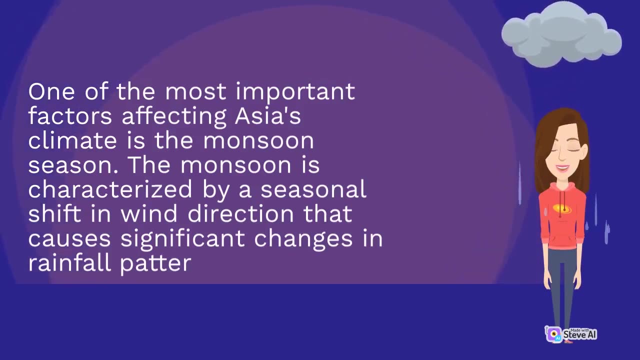 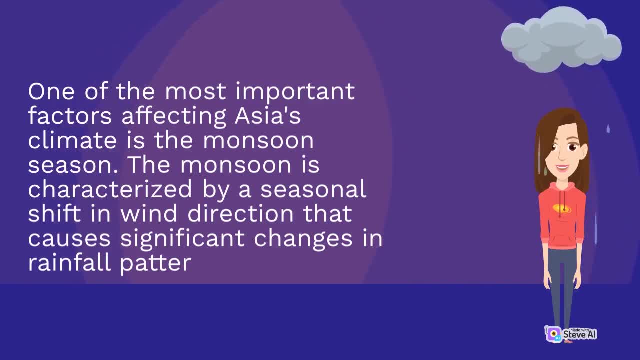 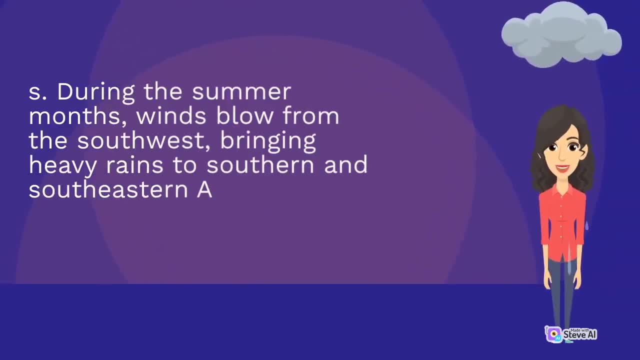 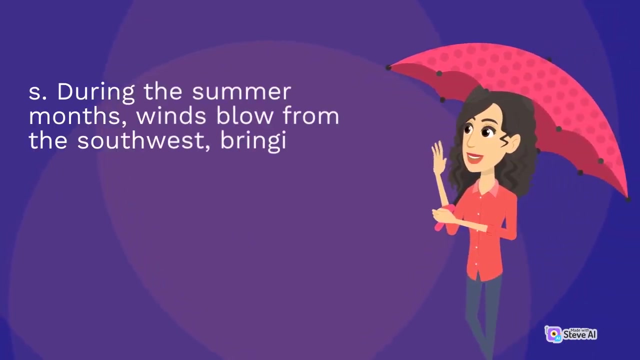 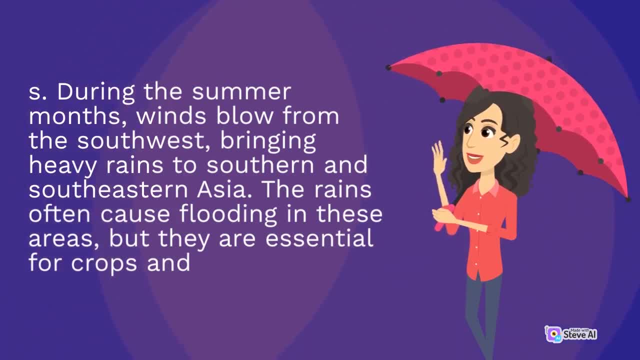 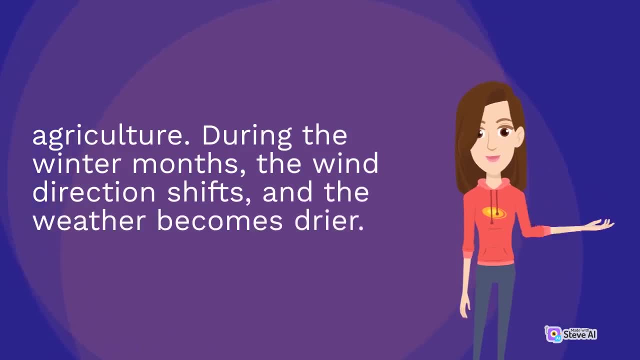 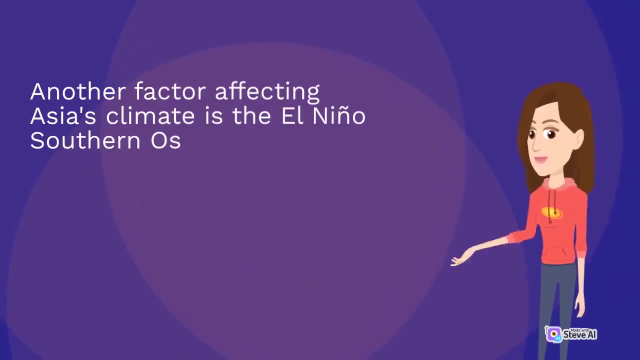 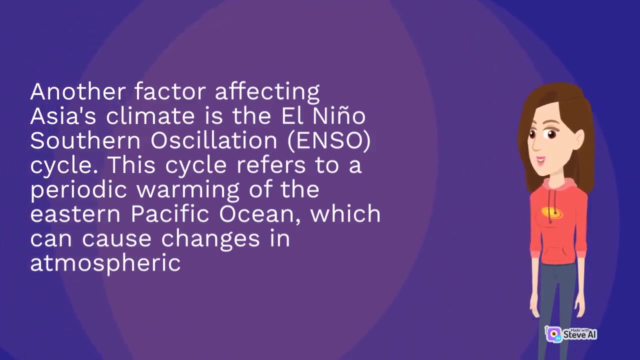 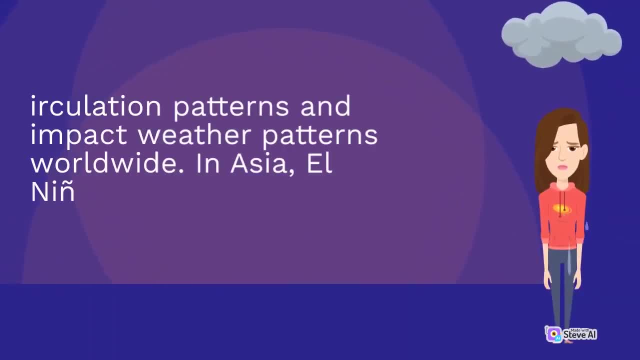 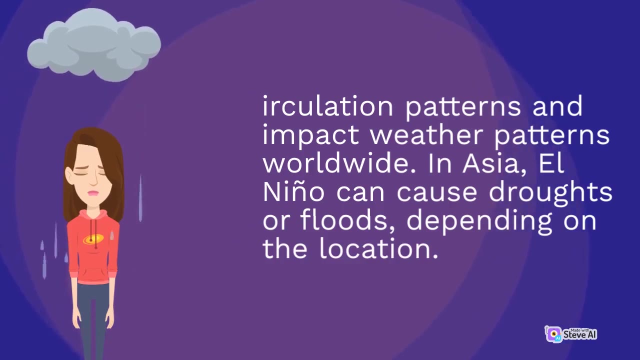 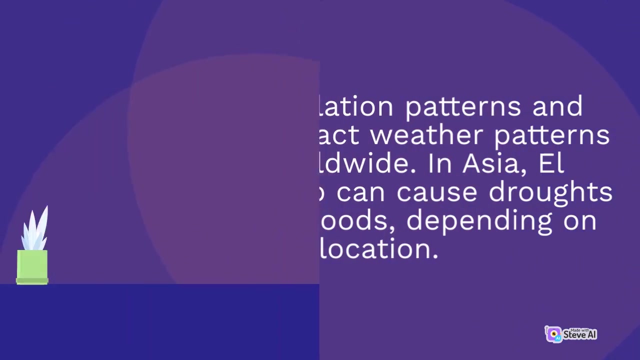 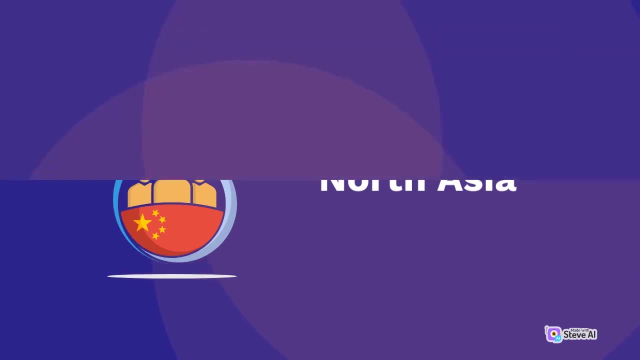 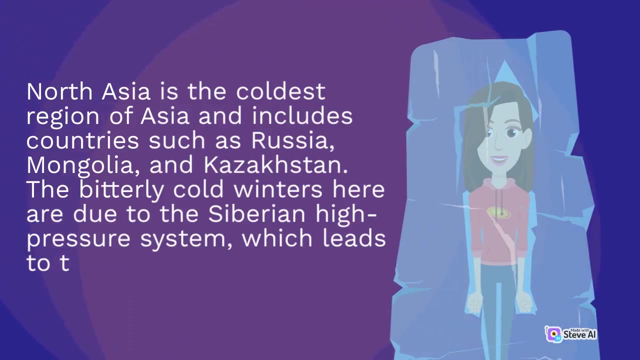 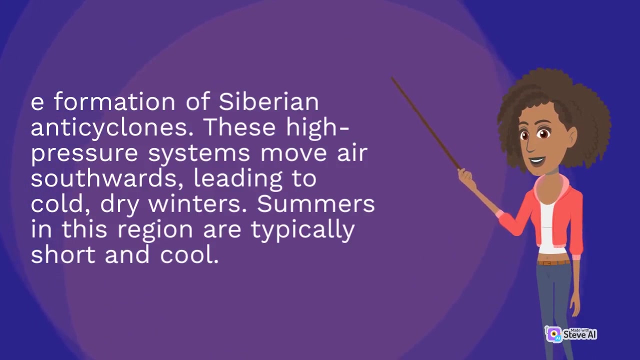 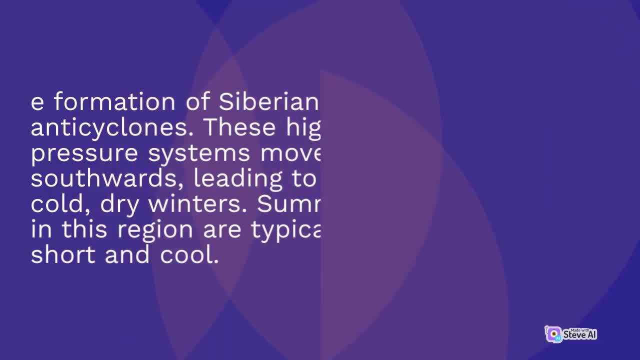 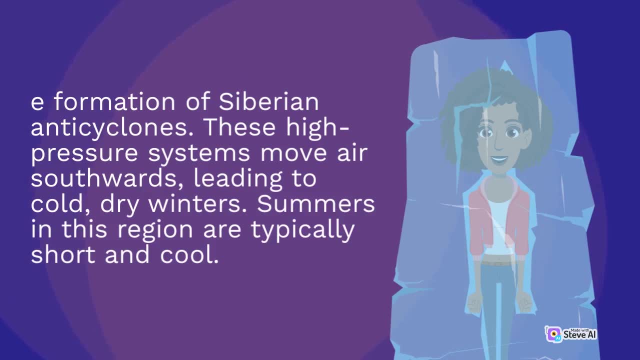 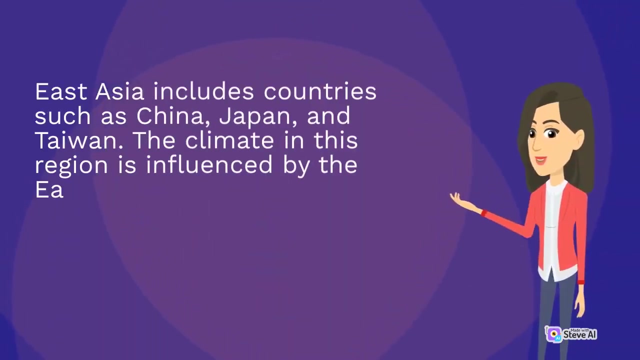 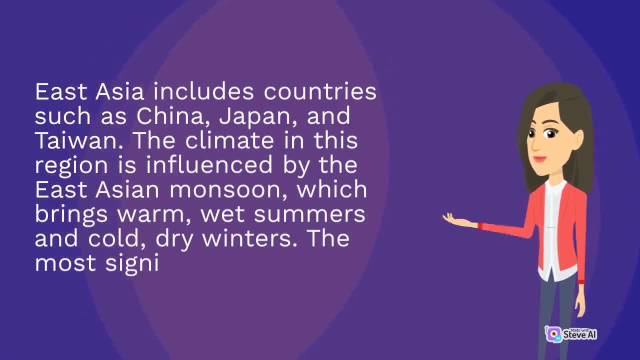 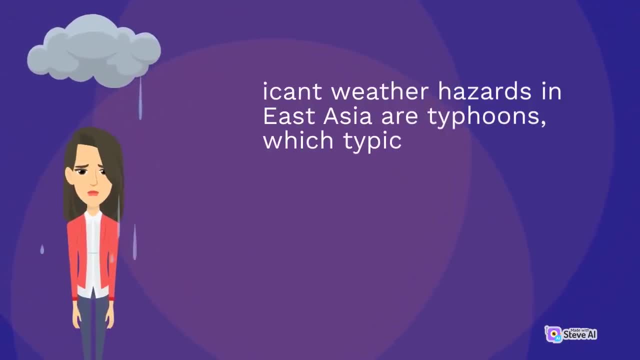 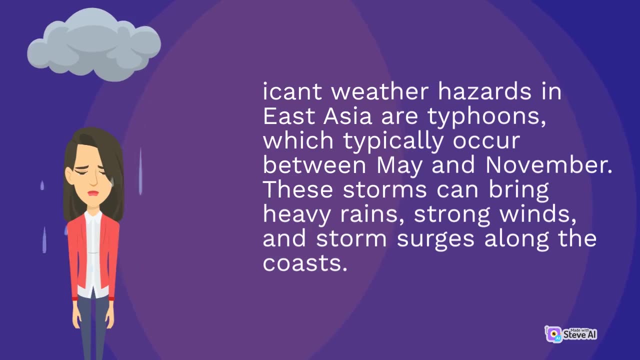 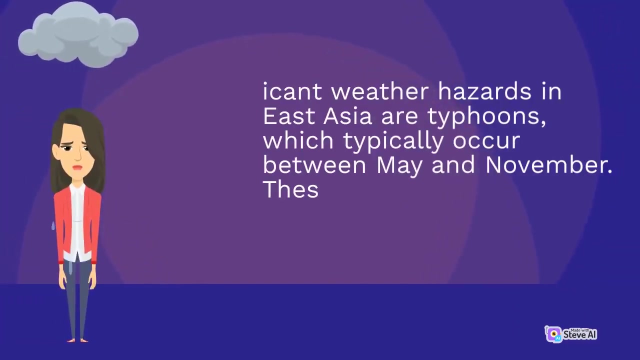 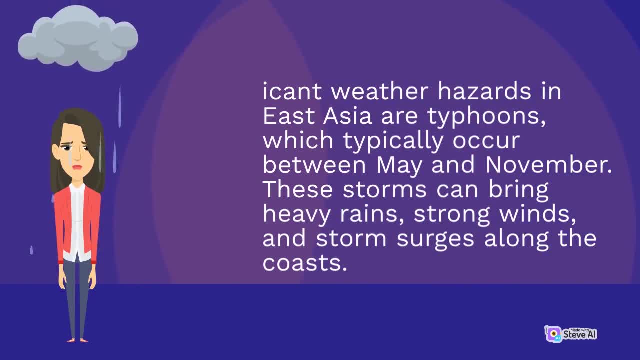 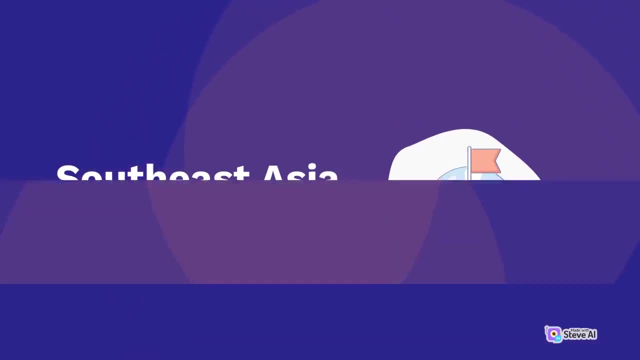 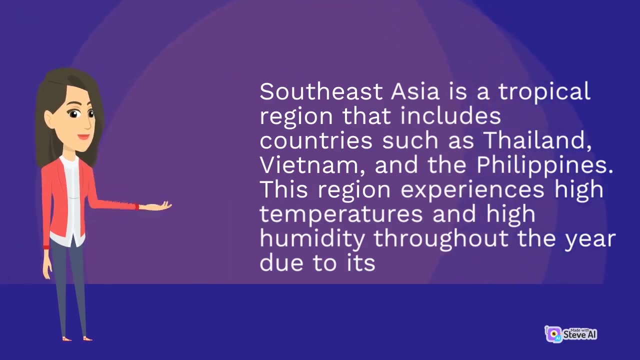 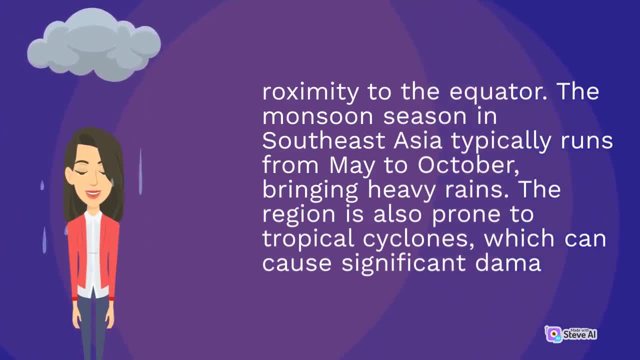 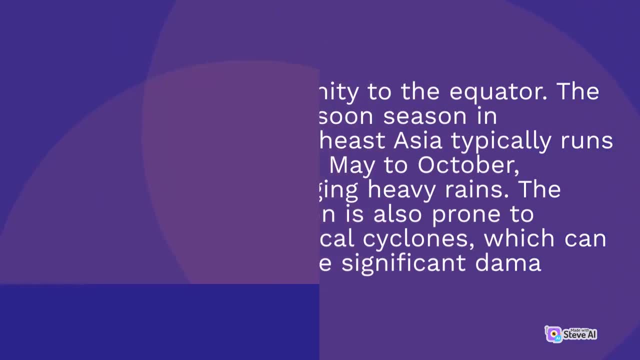 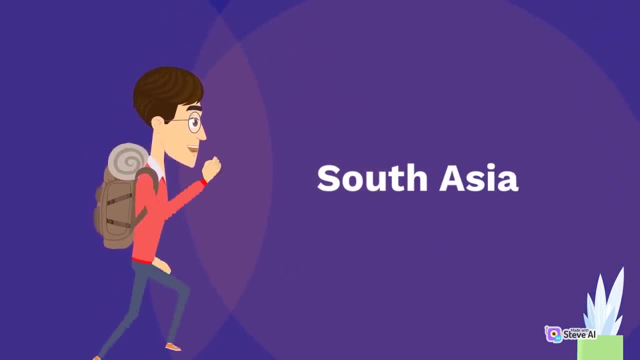 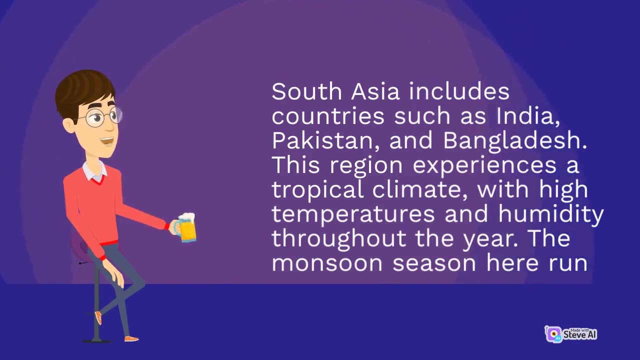 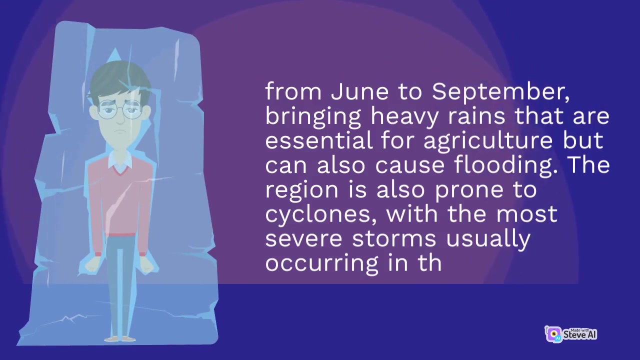 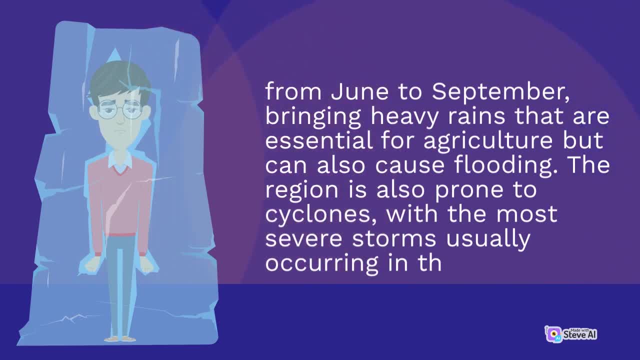 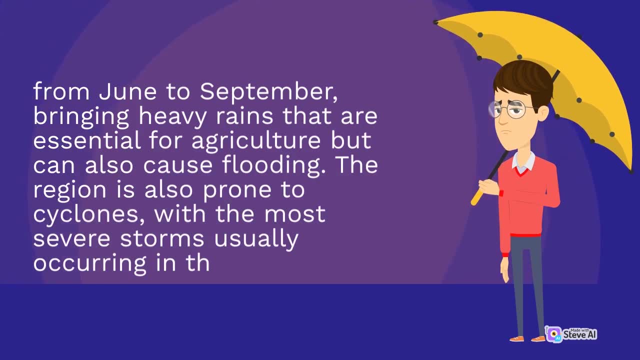 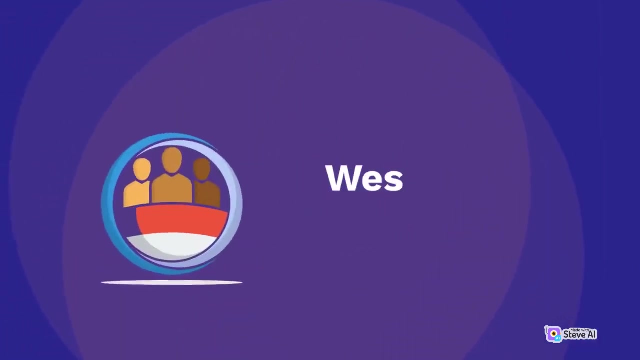 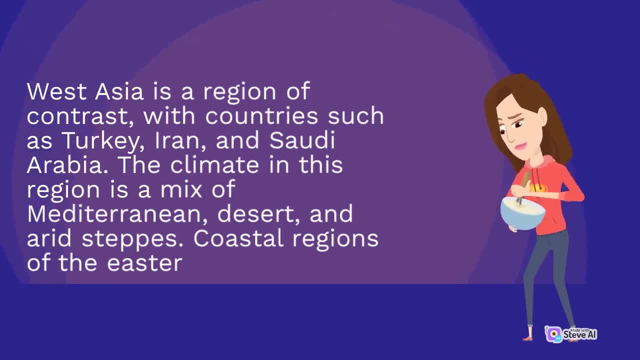 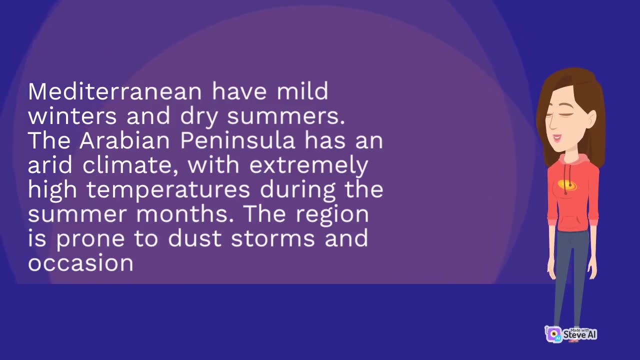 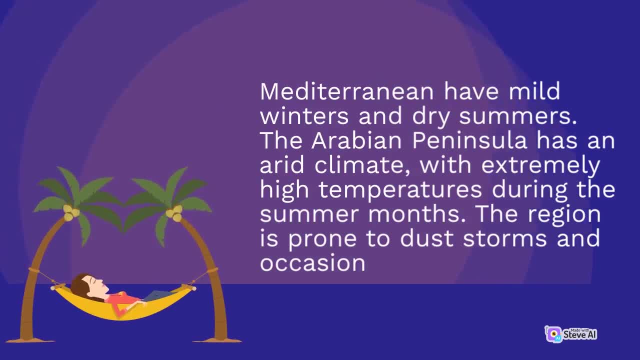 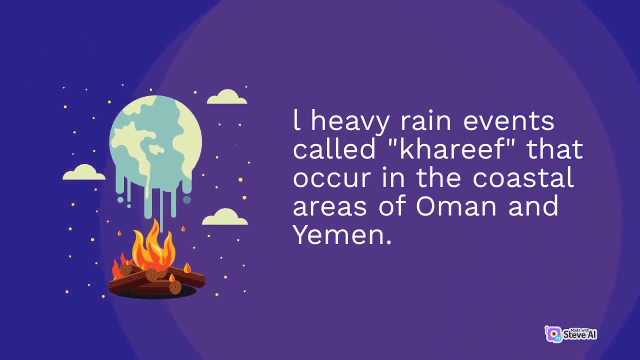 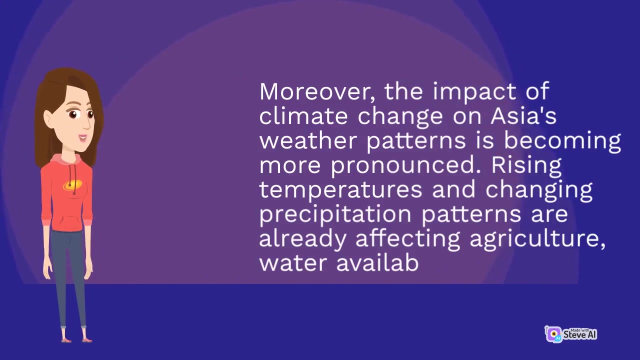 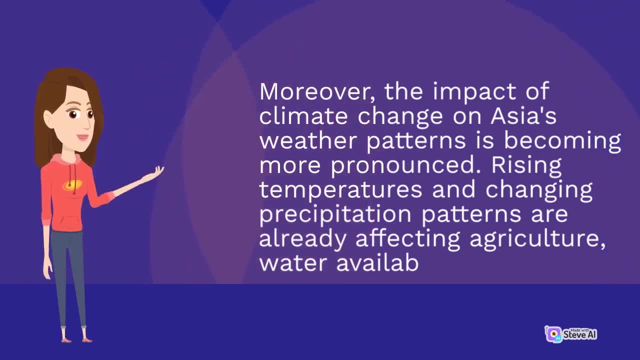 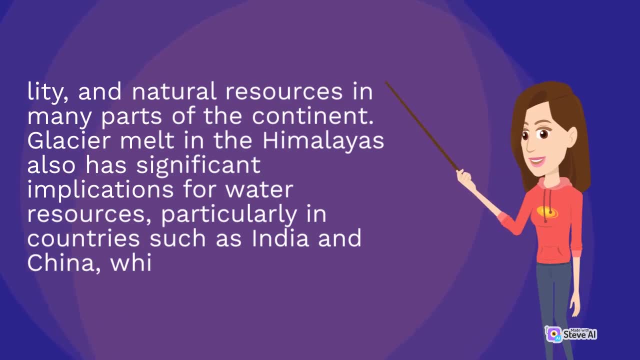 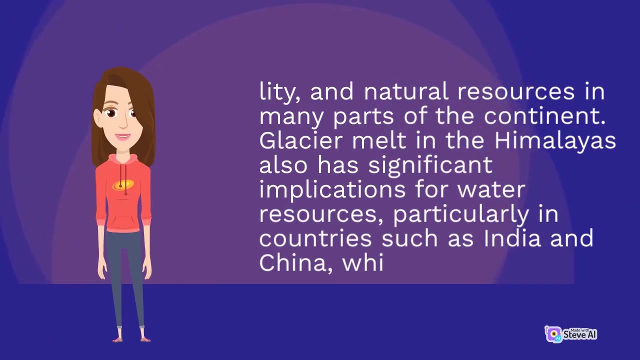 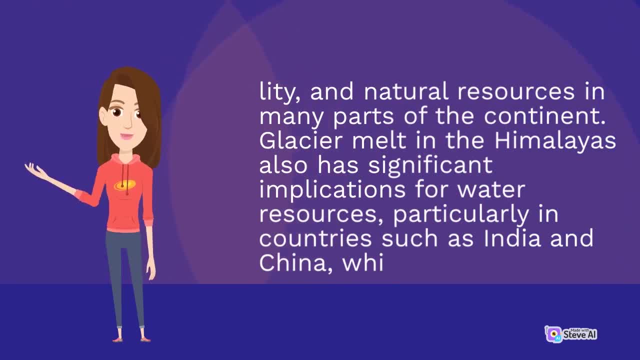 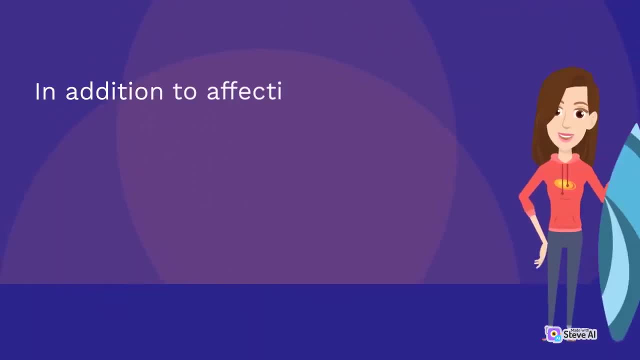 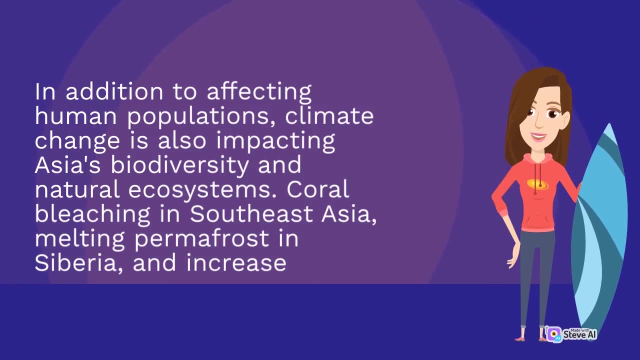 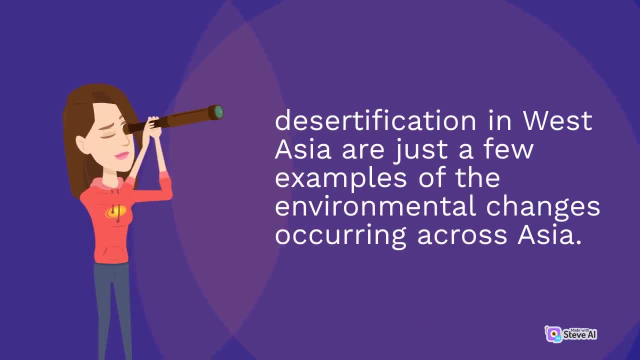 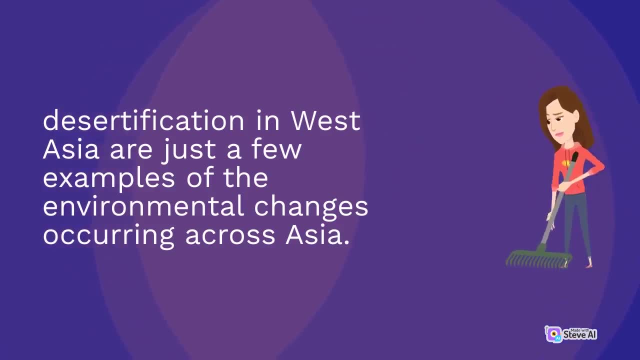 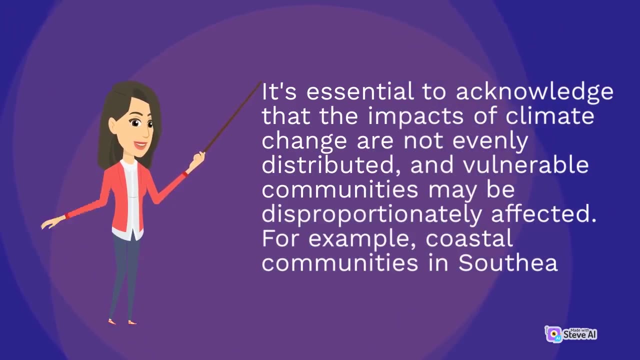 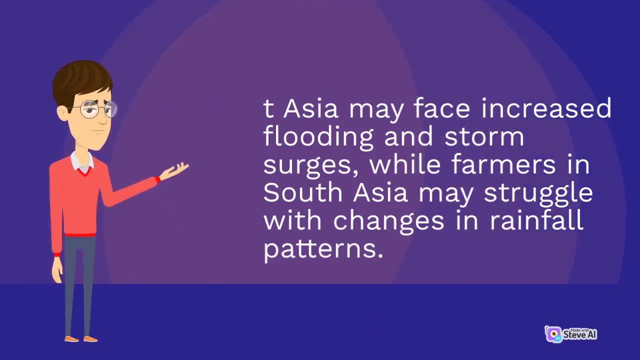 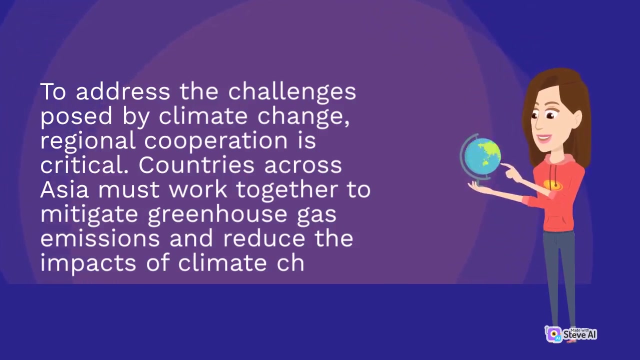